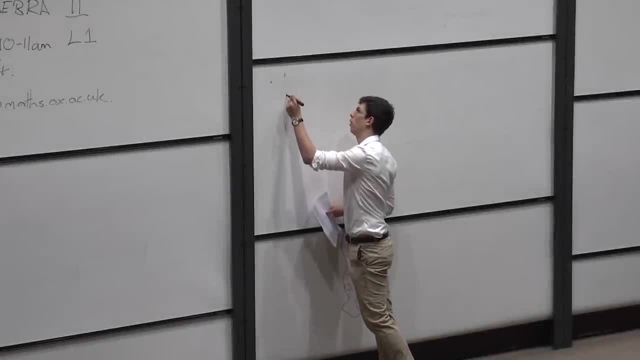 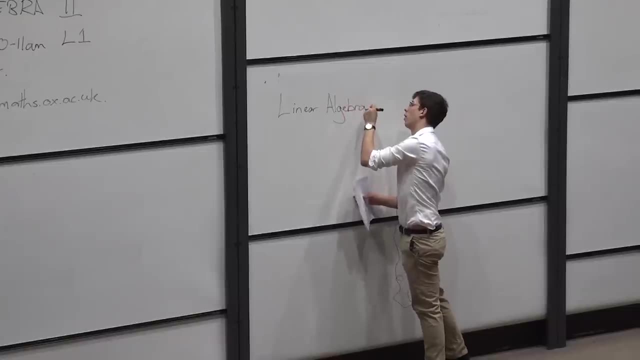 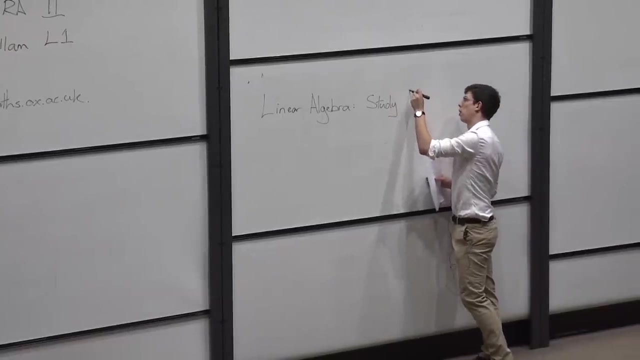 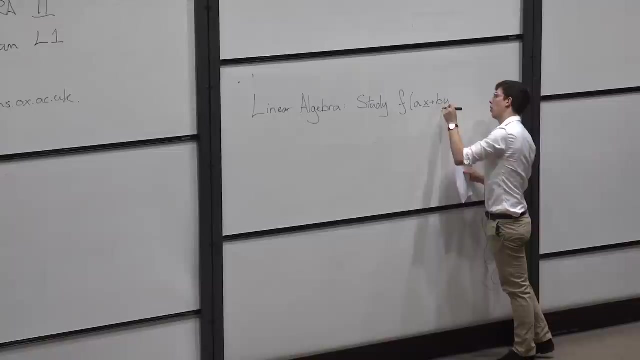 As you saw in Linear Algebra 1, the idea of Linear Algebra is really to study, maybe, functions which have the property that f of a, x plus b y is a times f of x plus b times f of y. 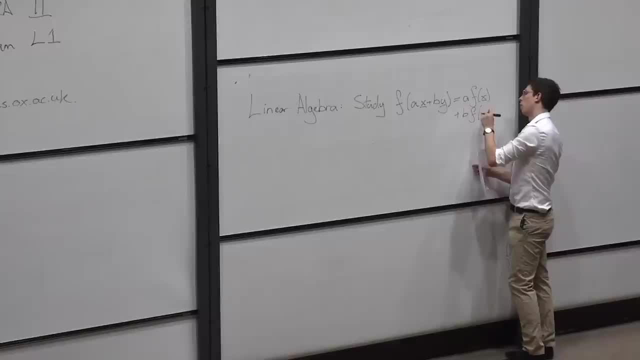 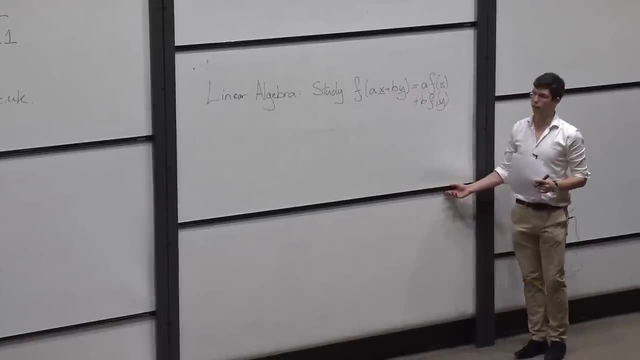 a times f of x plus b times f of y, a times f of x plus b times f of y of y. And here maybe I'm thinking of x and y as being vectors and a and b as being scalars, but you could also: 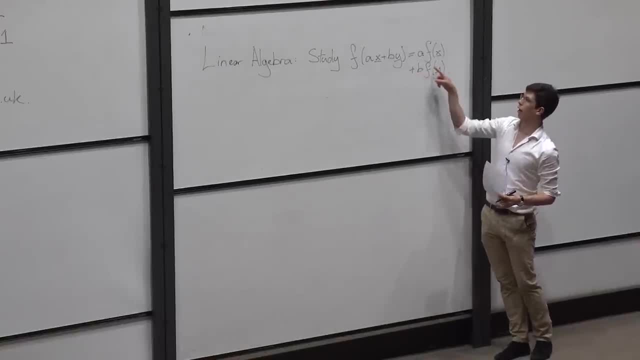 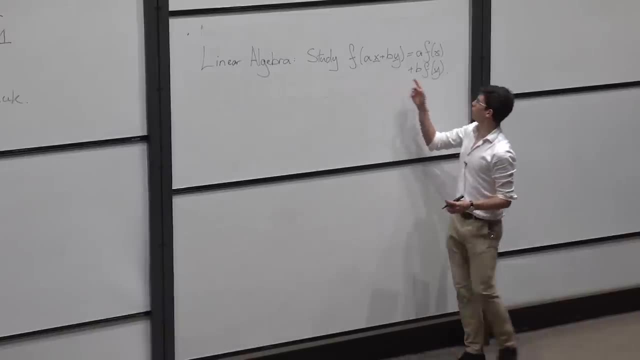 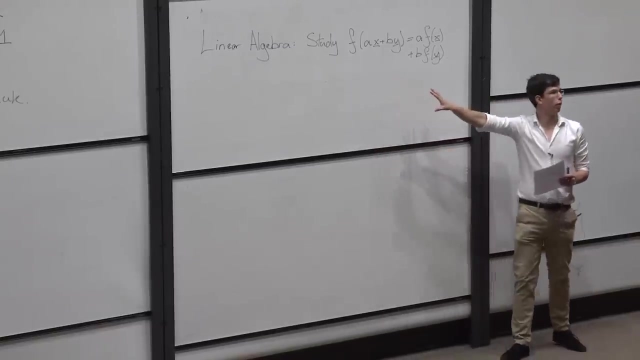 imagine slightly more general situations where this is true, And any function that satisfies this. we call it linear, And then linear algebra is the algebraic study of these sorts of functions, And it turns out that this is one of the most important and well-understood areas. 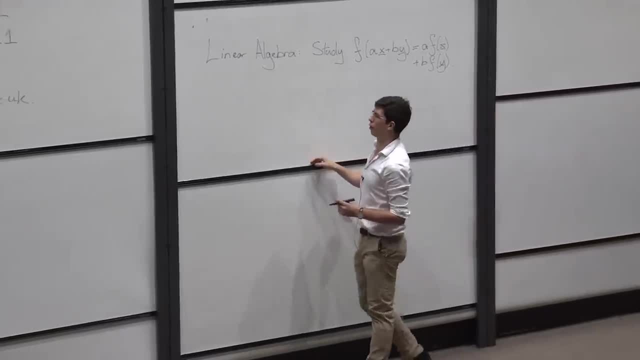 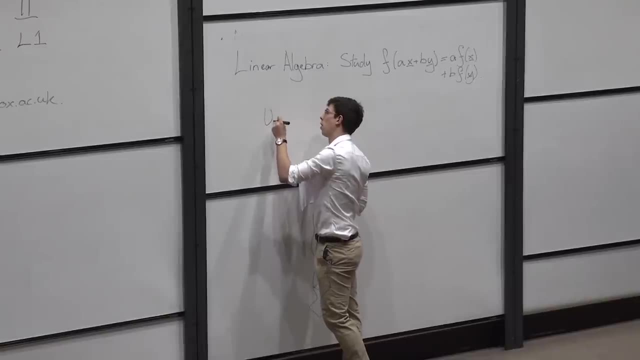 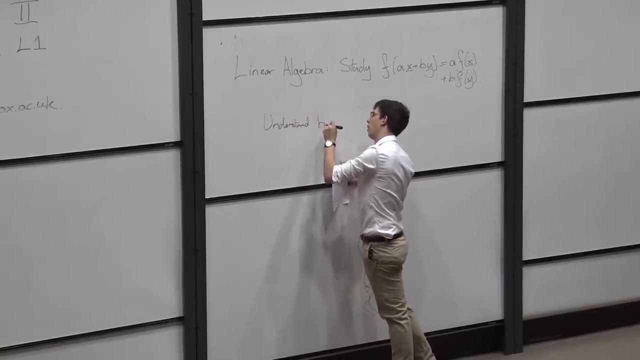 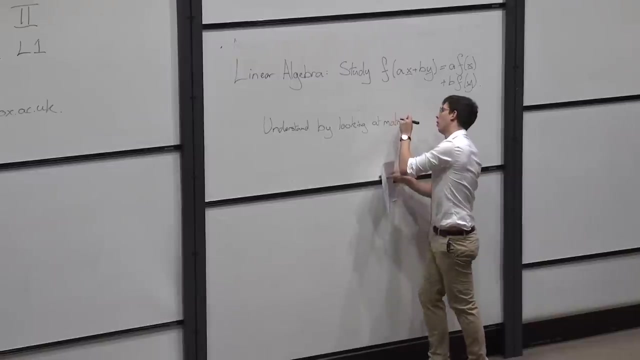 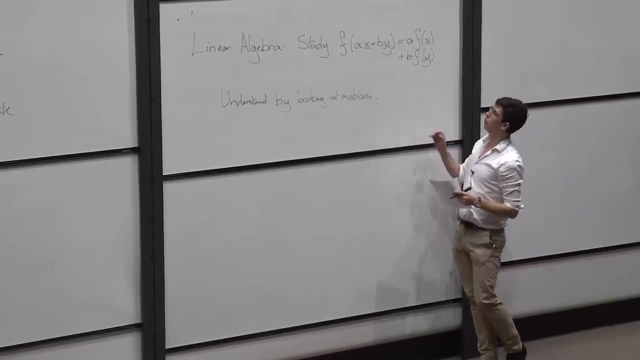 of mathematics. So there's a very beautiful theory of this And one quick summary is: you can understand a lot about this by looking at matrices and vector spaces, so objects that we've encountered in linear algebra 1. And actually a huge amount of modern mathematics. 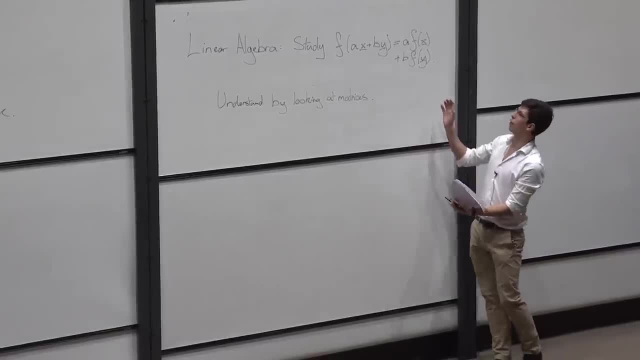 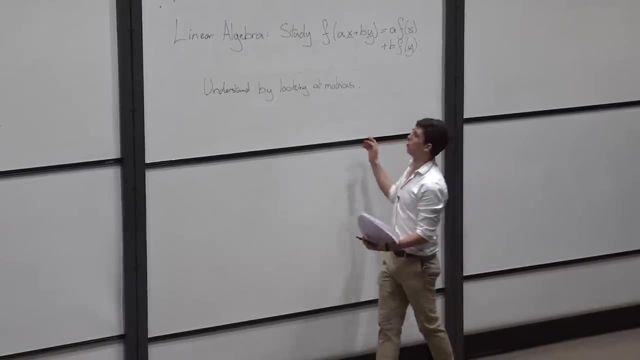 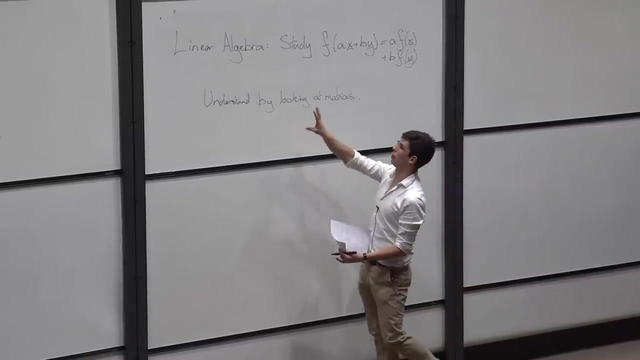 is often to take some very complicated situation and to try and maybe approximate it in some way by some linear system. So when you do calculus you're approximating a more general function by something that looks linear on a small scale, And linear algebra really lies at the very heart. 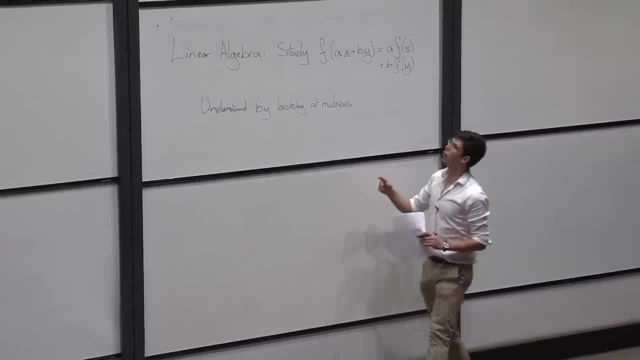 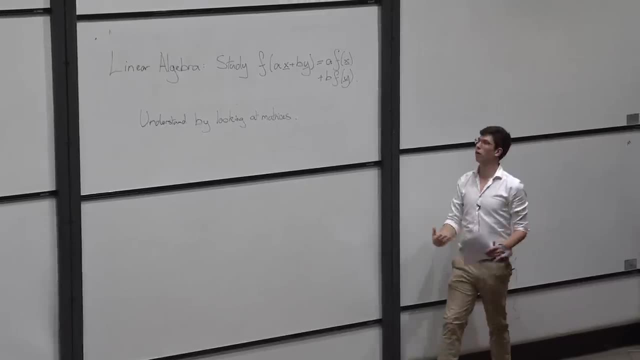 of a huge amount of mathematics, So I'm going to show you how to do this. You've maybe already seen that linear algebra has various different applications. If you want to solve simultaneous equations, you can cast this as a problem in linear algebra. 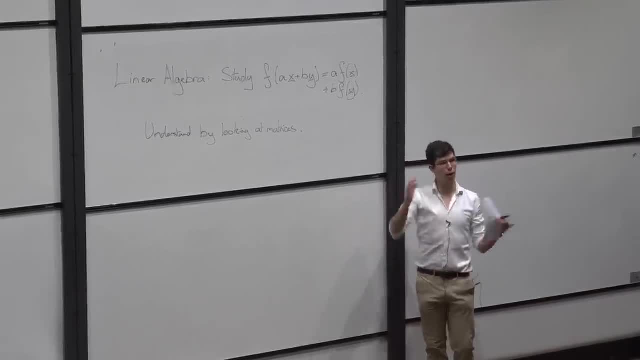 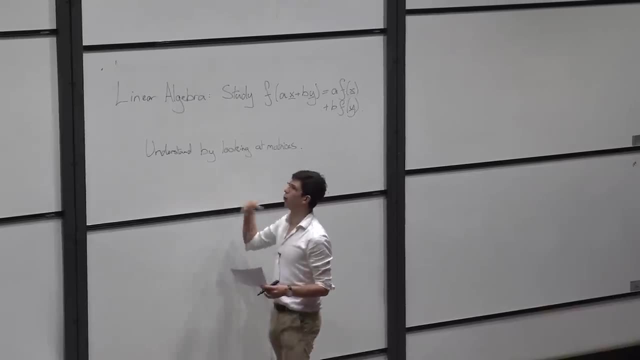 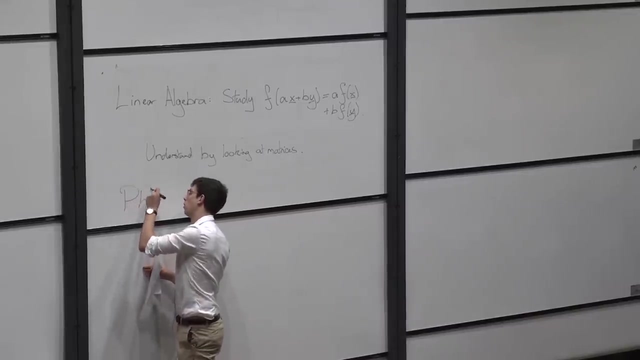 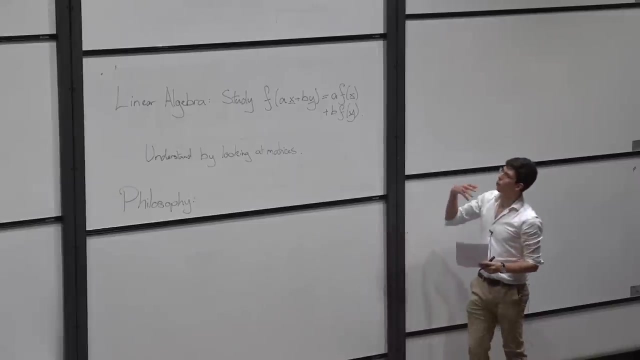 just as you can understand linear algebra as looking at vector spaces and more geometric problems, And one philosophy for the way that I like to think about linear algebra that I think would be useful in this course Is to when you're thinking about statements. 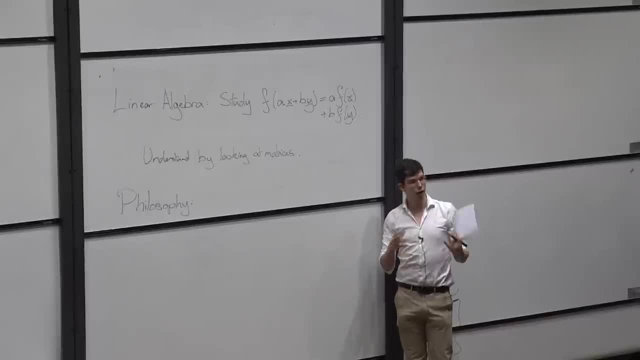 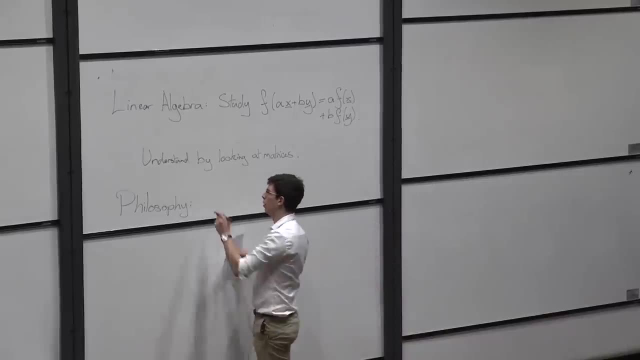 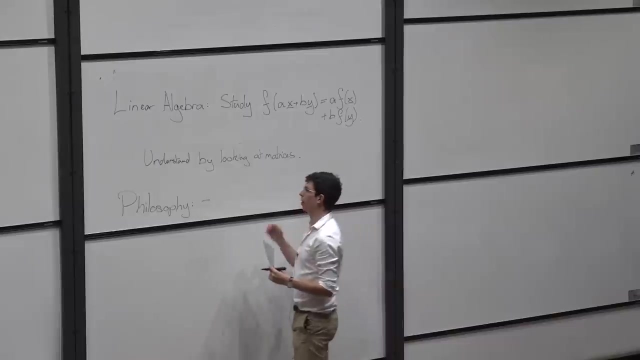 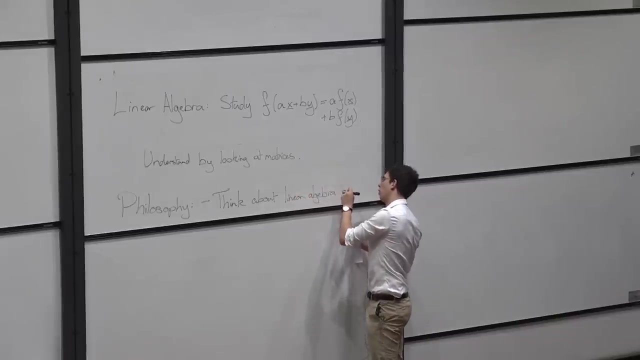 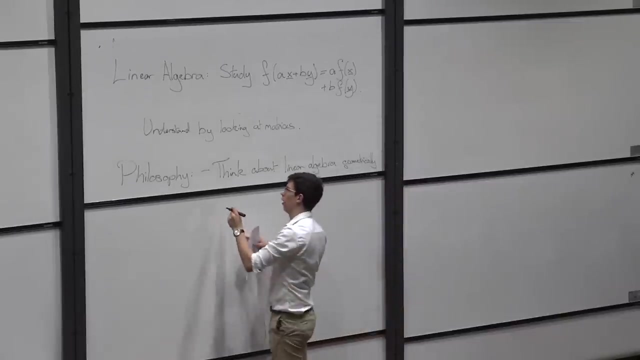 to always imagine them geometrically as questions about 2 by 2 matrices and transformations of the plane, But to always write down proofs and arguments much more abstractly using algebra. So think about linear algebra geometrically in particular, as say, transformations of the plane. 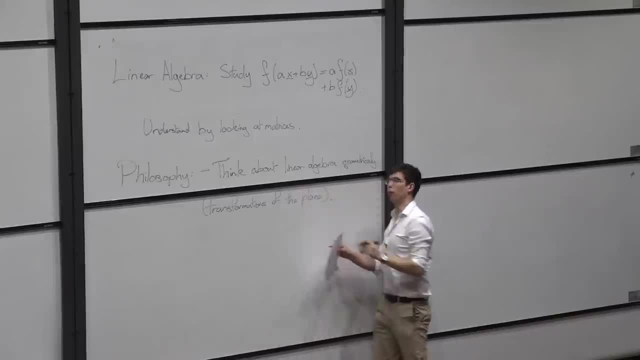 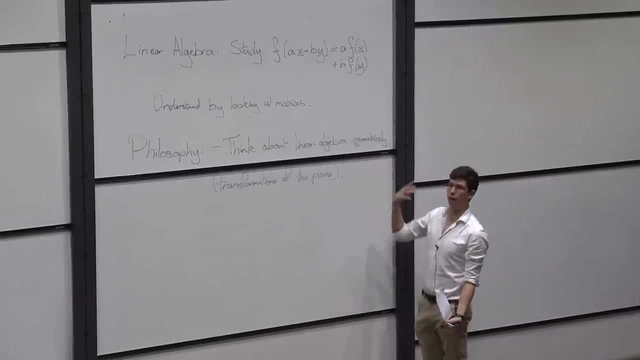 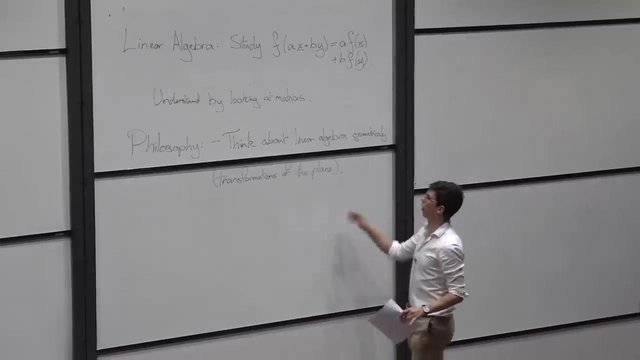 So I'm not too good at visualizing things in three dimensions, But I can visualize things OK in two dimensions, And often it's very easy to visualize things if you just imagine that everything is some operation on the plane. So I like to think about what's going on. 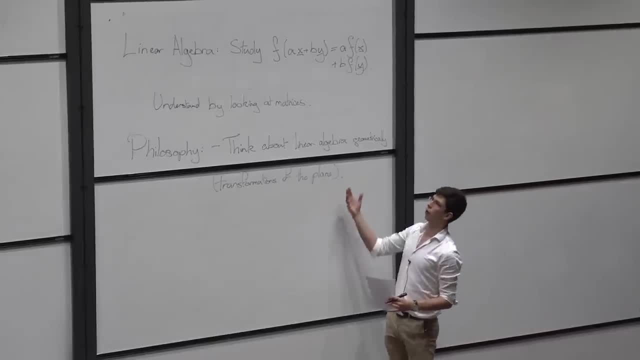 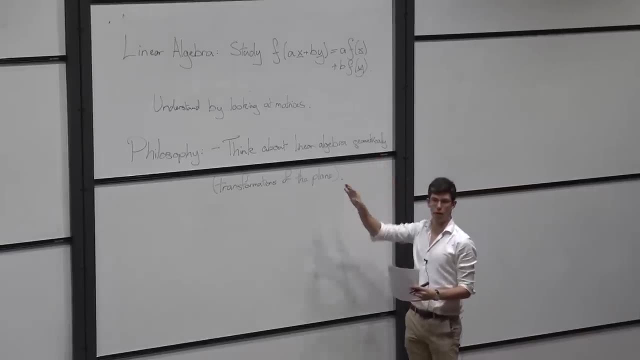 in a sort of geometric way, But we're going to prove rather more general statements. And one of the big powerful things about linear algebra is: I hate this geometric intuition, But then write down formulae that work in arbitrary dimensions in a very nice way. 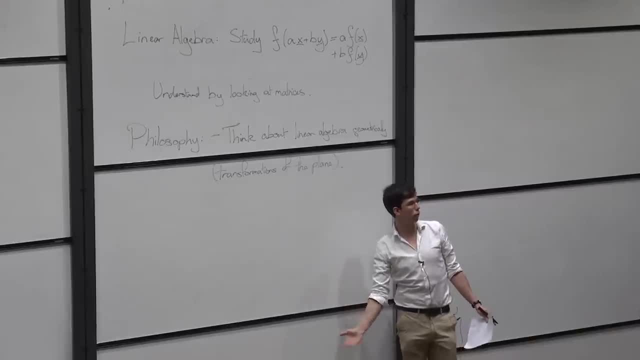 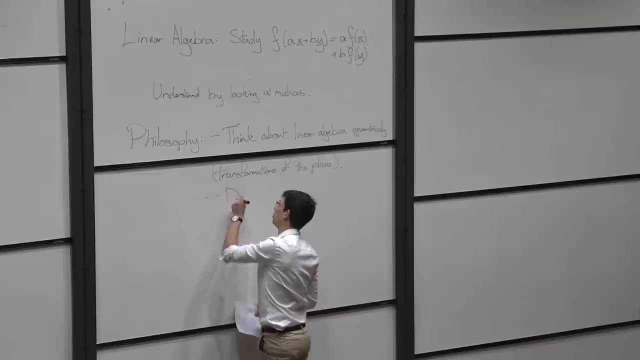 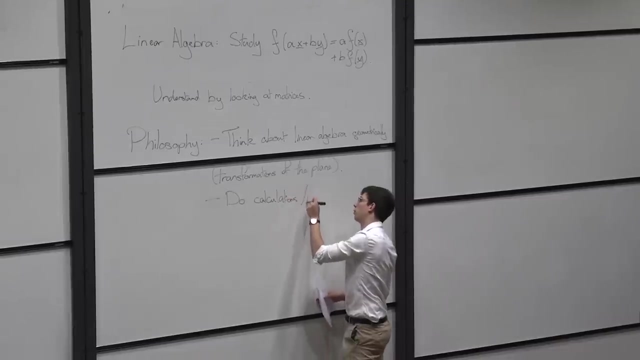 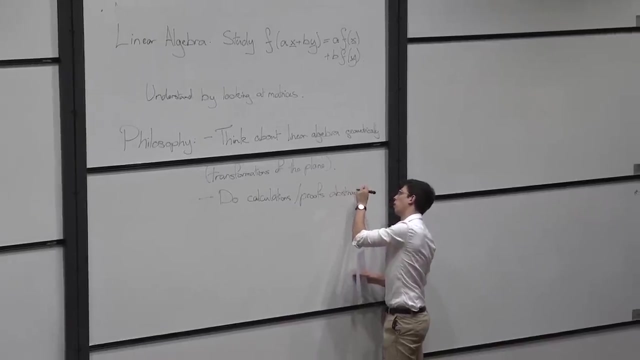 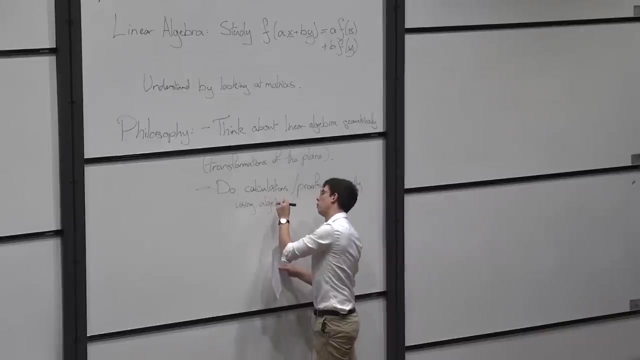 And often the algebraic way of doing the calculations is much, much more convenient than the geometric way, even if maybe we were actually motivated by the geometry. So I want to do calculations and proofs abstractly using algebra. So if you do it this way, the proofs and the statements 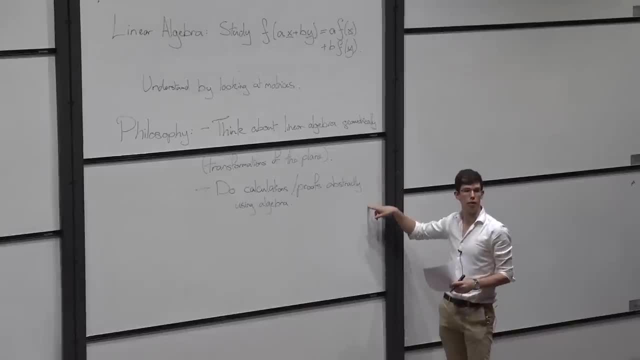 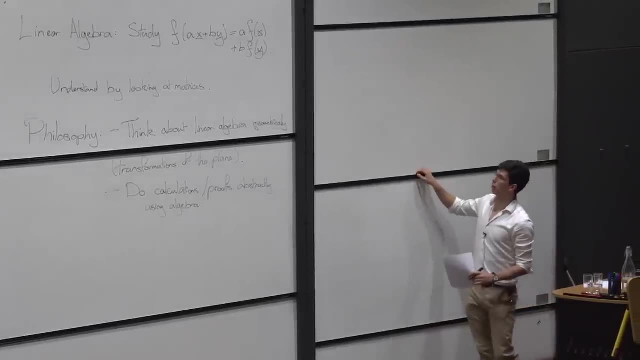 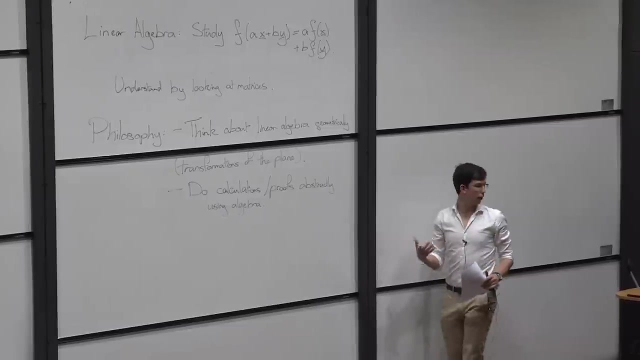 often hold in much more generality, But also it's much more convenient to do the calculations in this way. And OK, So I've maybe said this In very vague terms. maybe we can sort of think about a concrete example as to how this might work. 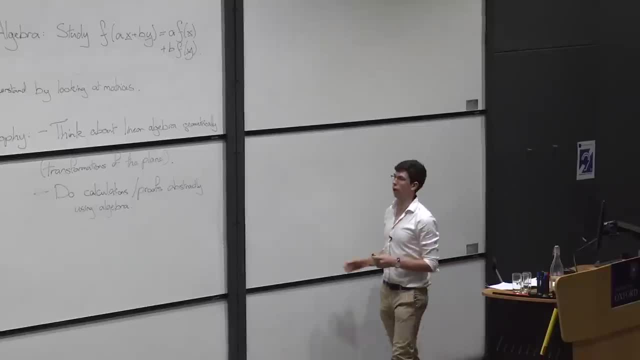 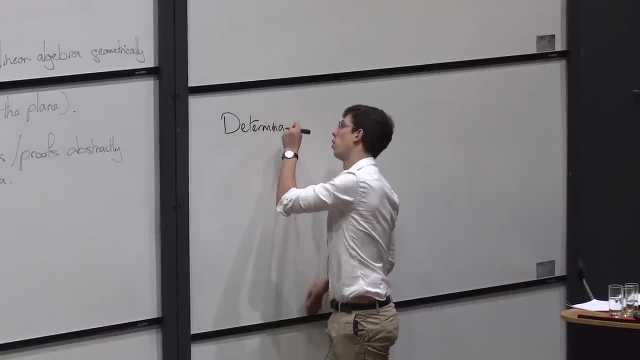 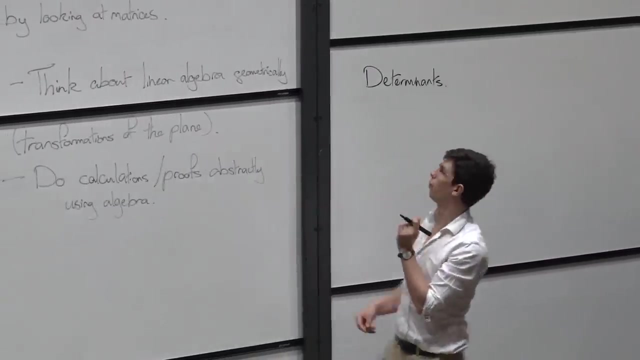 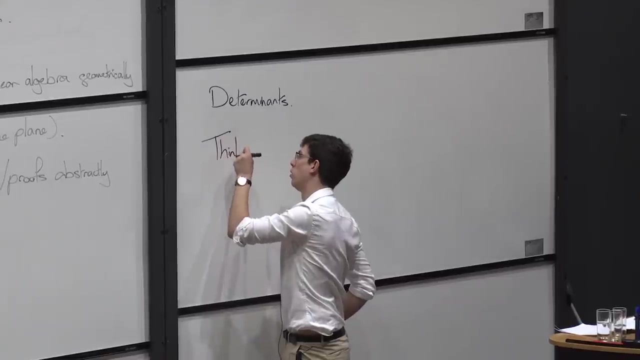 And this gets us to the first thing that I'd like to talk about in linear algebra, which is determinants, But I'd like to demonstrate it through this sort of philosophy. So Let's think of just some linear transformation of the plane. 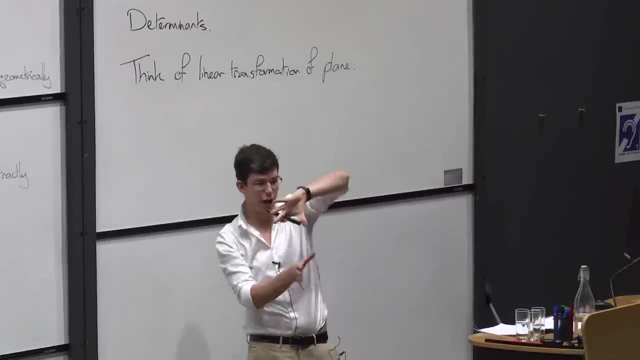 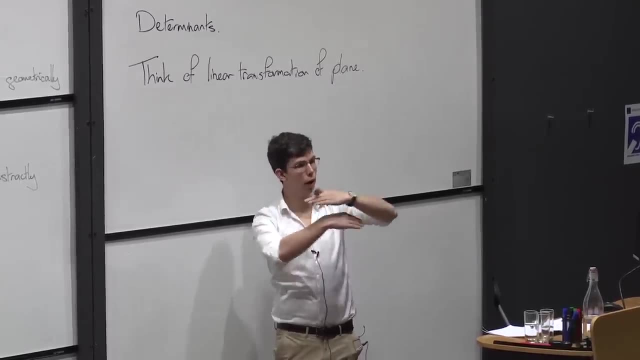 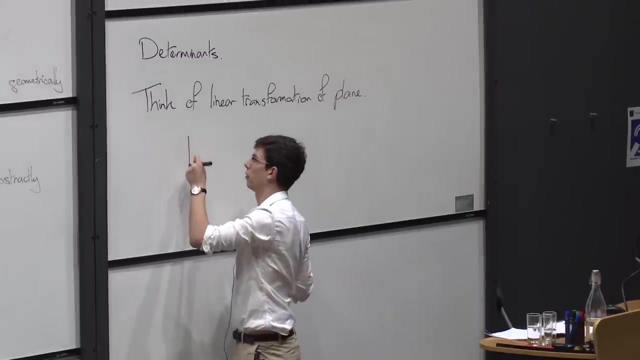 So what do I mean by this? Well, some combination of rotation or stretching in one direction, Or maybe I could skew it if I shift things. But a linear transformation is going to preserve lines And I can think about just taking the unit box. 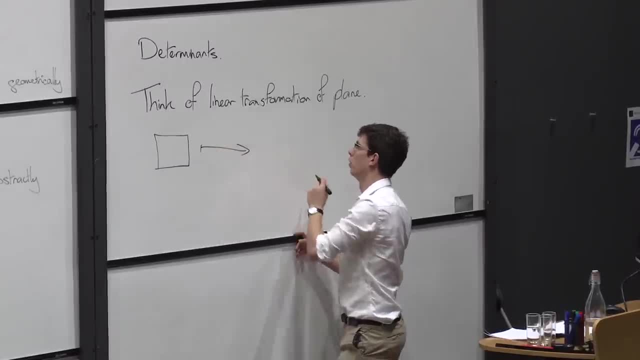 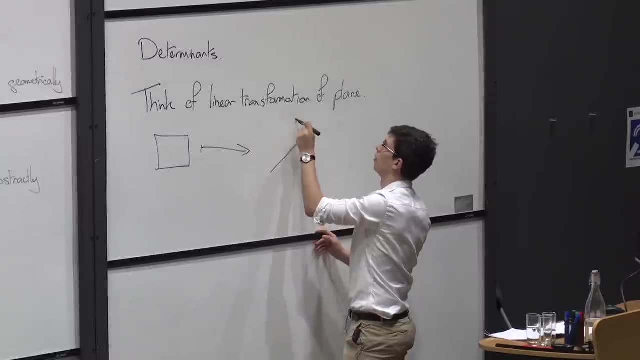 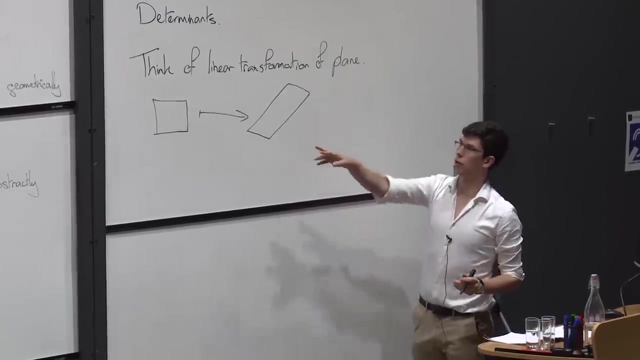 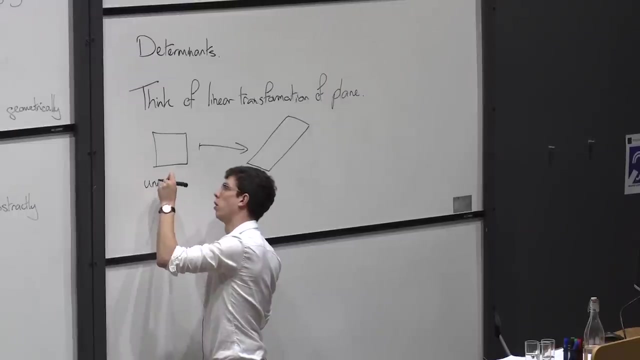 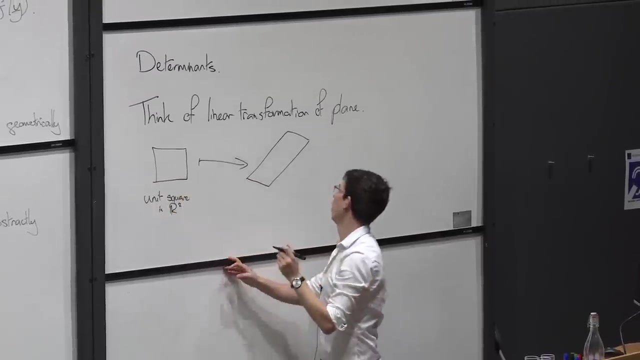 And this will then be mapped to some maybe skewed box, So it'll be some sort of parallelogram And maybe the axes won't be what I was onto anymore, And I want to understand transformations like this. So this is just the unit square in r squared. 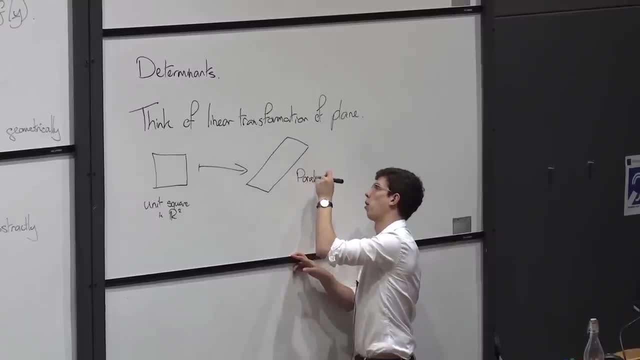 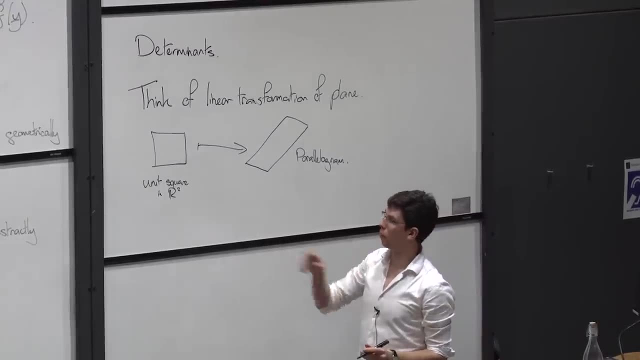 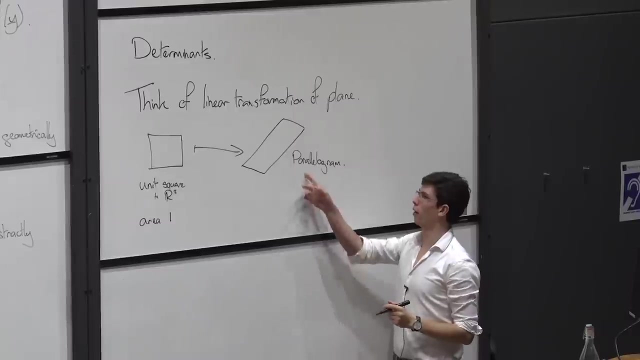 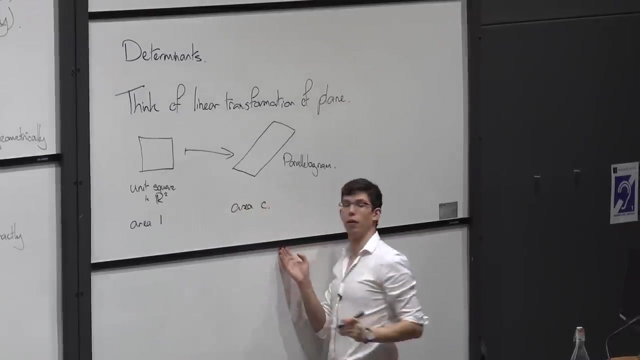 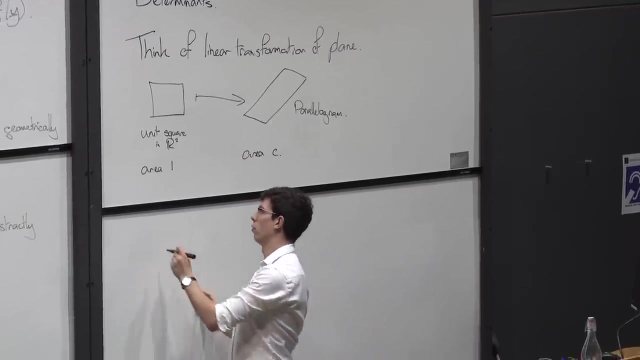 And then this gets mapped to some parallelogram And the unit square has area And this parallelogram, the area, won't necessarily be preserved, So we'll have some different area c, But I can think about the linear transformation acting on other shapes. 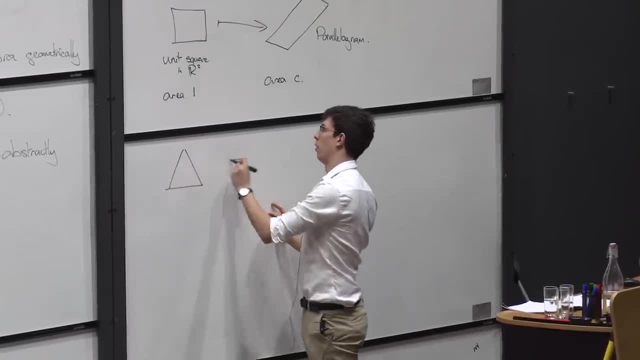 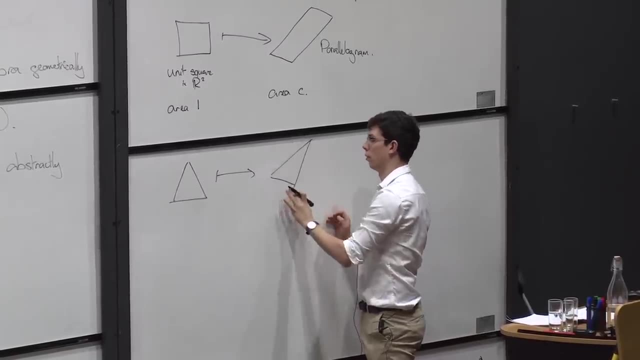 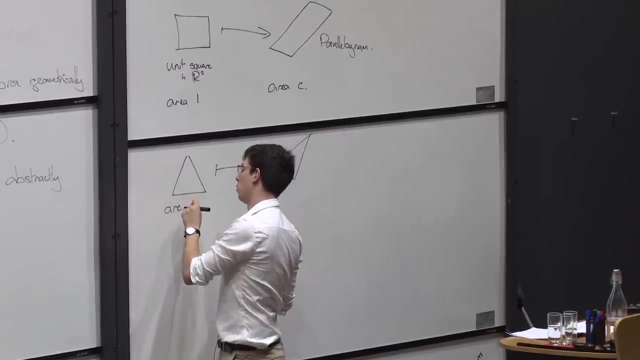 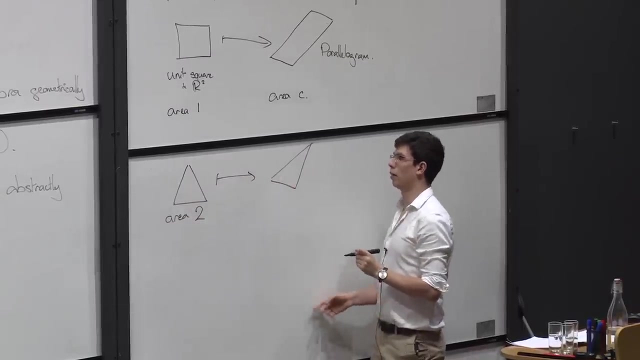 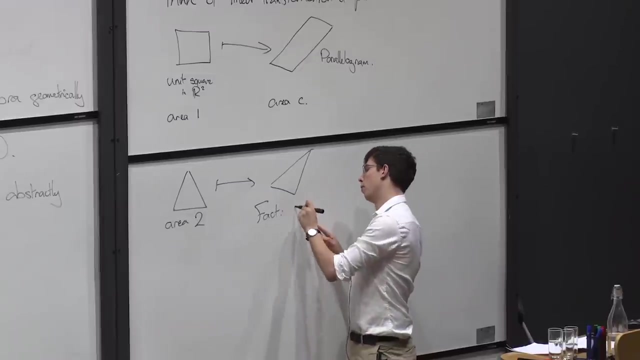 So I could have maybe a triangle And then so that will get mapped to some strange skewed triangle or something And maybe I can draw some triangle with area 2. And it's a fact that the image of the triangle would then have area 2c. 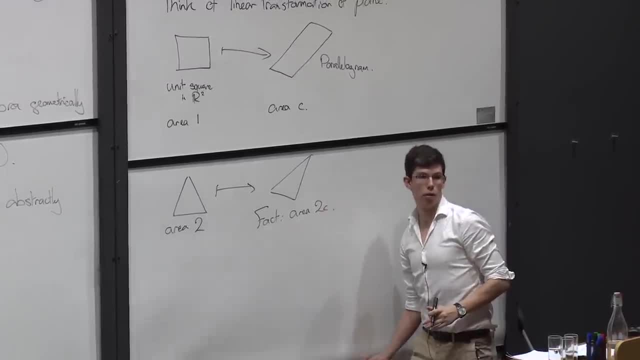 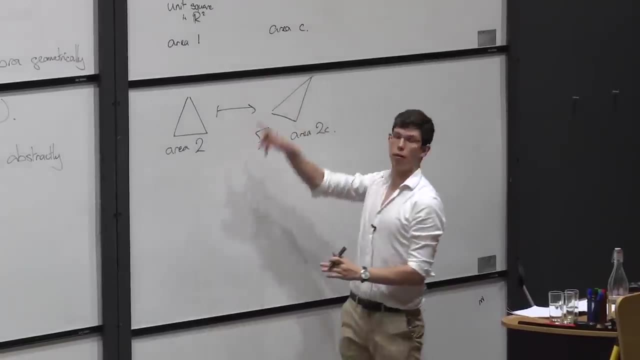 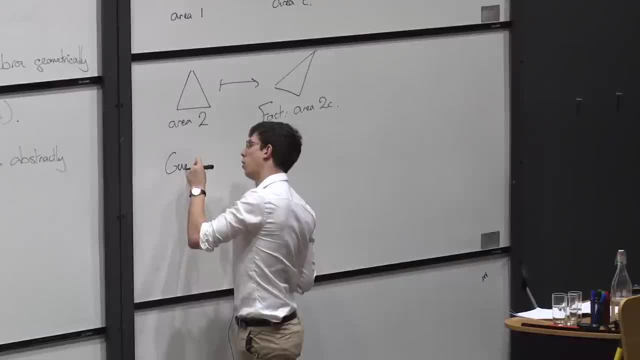 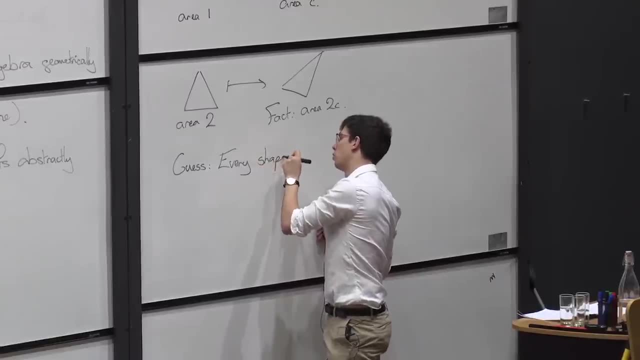 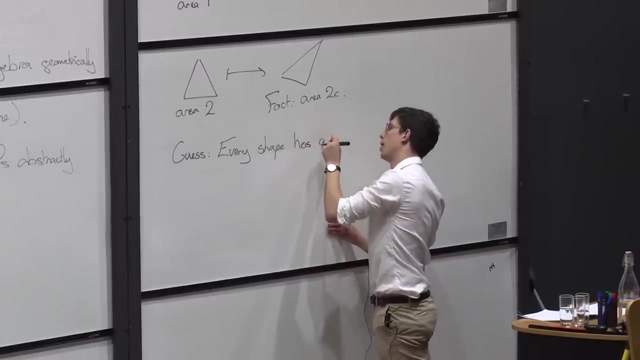 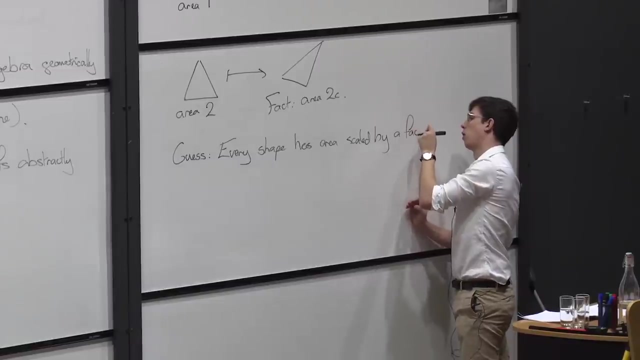 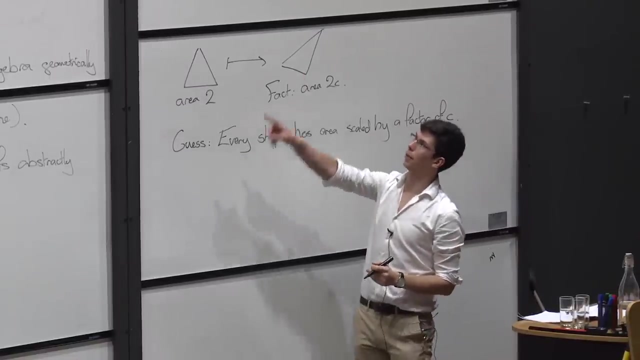 like this, that every shape- well, I'm not going to be precise about what I mean by shape- has the area scaled by a factor of c. So often it's unwise to make a general guess just from doing two examples, But you can do a few more examples if you like. 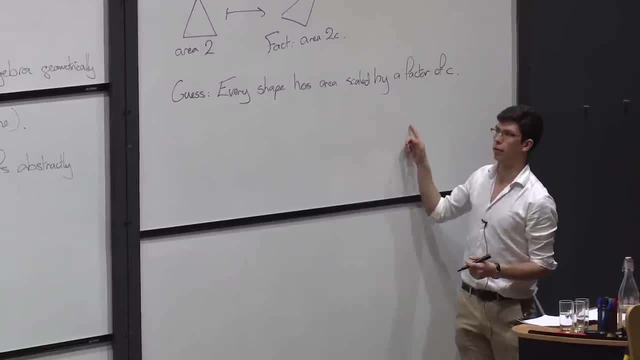 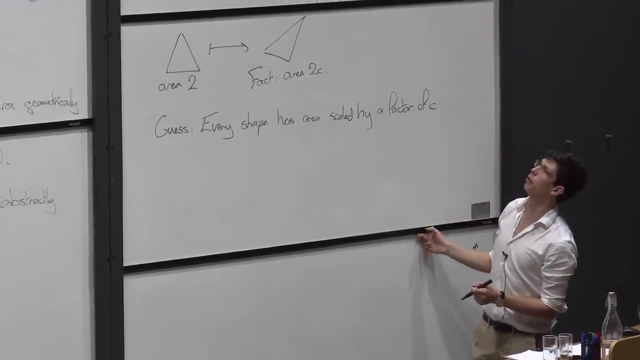 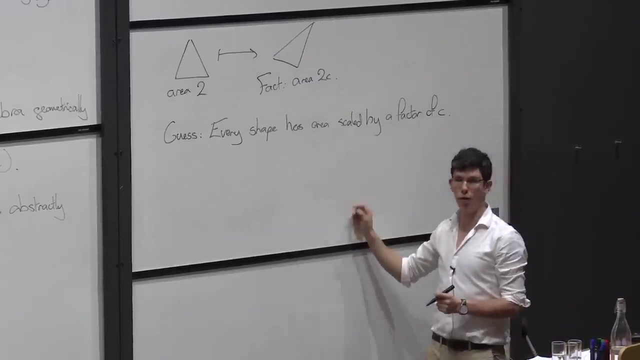 And it turns out this guess is true And this constant c is going to depend on the linear transformation And this constant c is essentially the determinant of the linear transformation. So it's clearly going to be some important property of any linear transformation that it turns out. 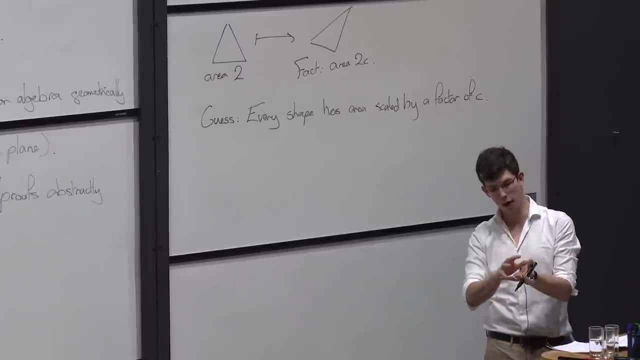 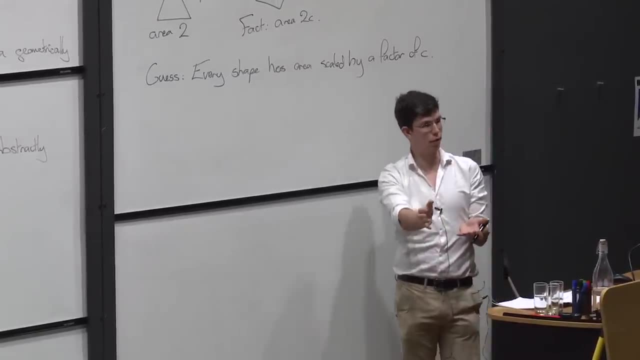 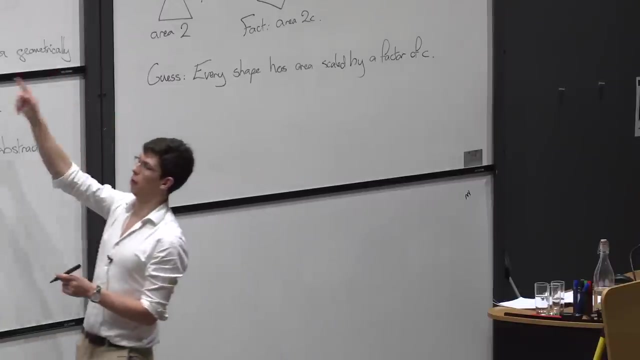 that even if you're working in many dimensions, any reasonable shape has its volume scaled by a constant factor, And this constant factor is called the determinant. So this is very much what I mean by thinking about things geometrically, But it turns out that it's really quite difficult to. 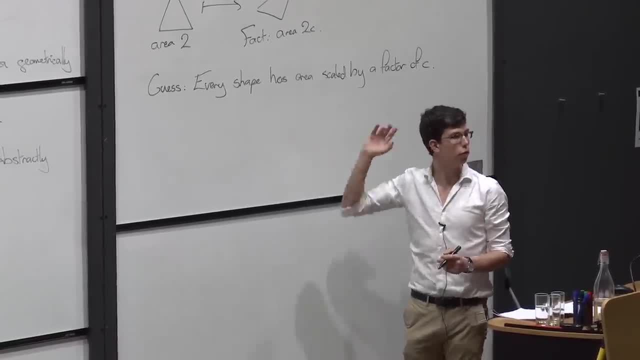 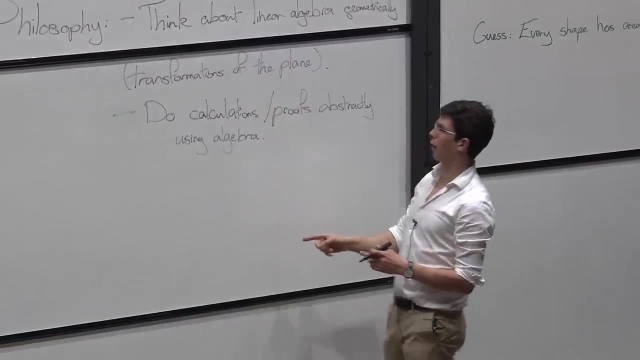 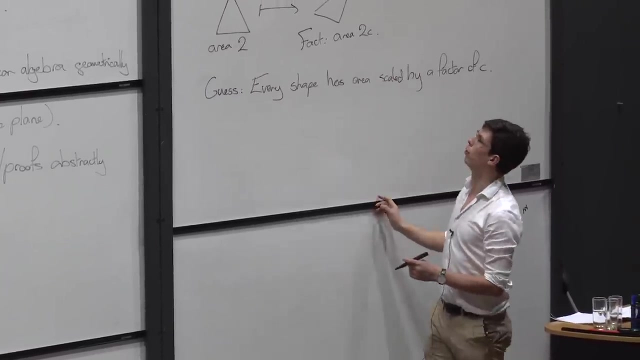 I think, make lots of this precise And the calculations get a bit horrible if you try and think about things just in terms of volumes. So very much in the spirit of this philosophy, I want to do calculations trying to abstract out properties of this. 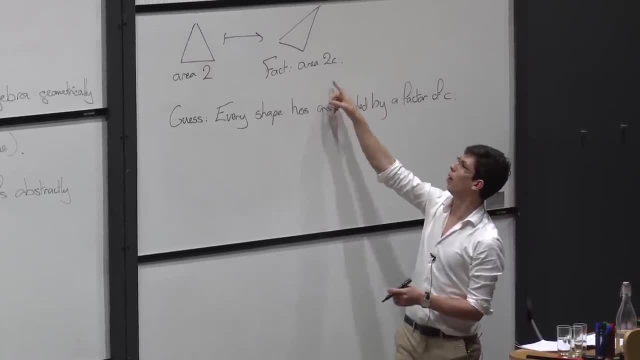 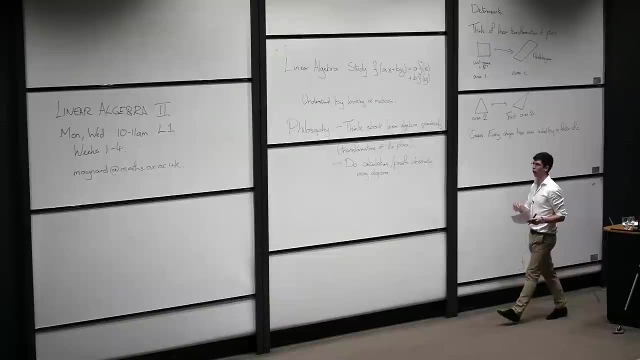 So let's think about a few properties of this scaling areas we'd have in r squared, And try and think of If I can do this, If I can do this, If I can do this, And write these down as abstract properties. 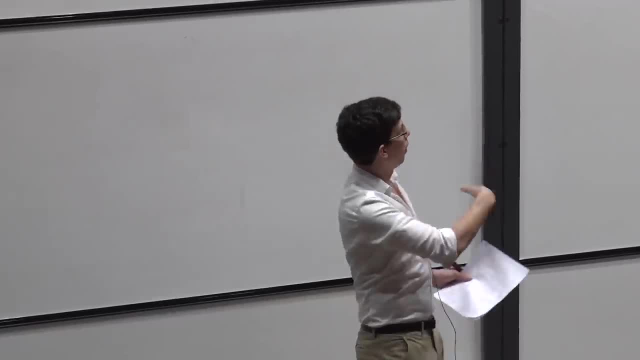 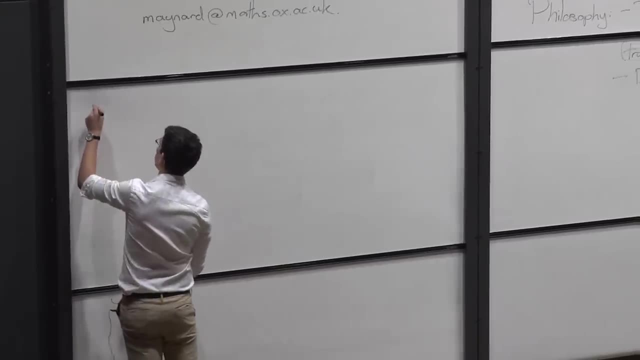 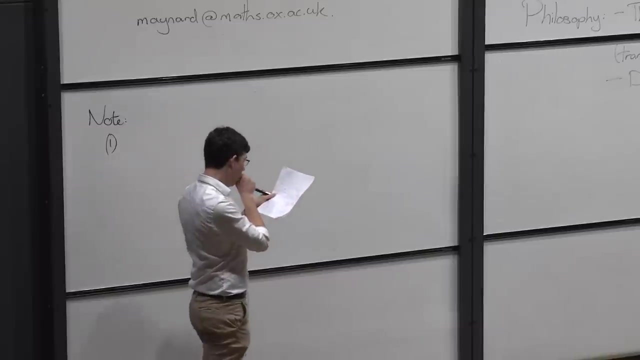 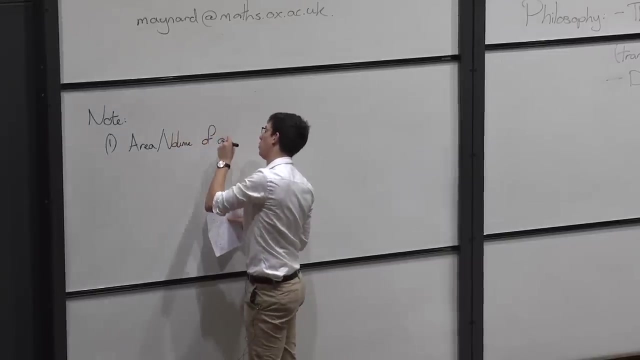 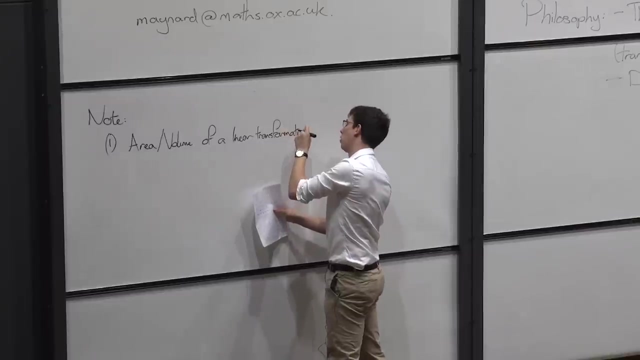 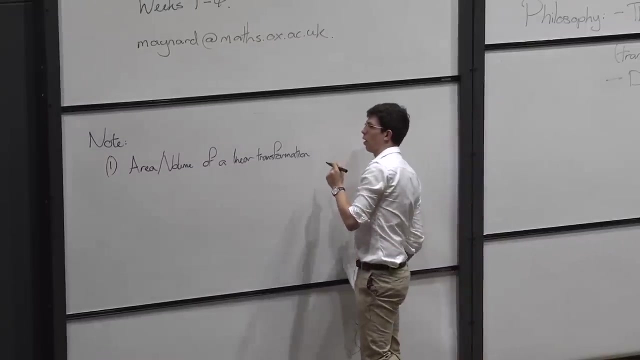 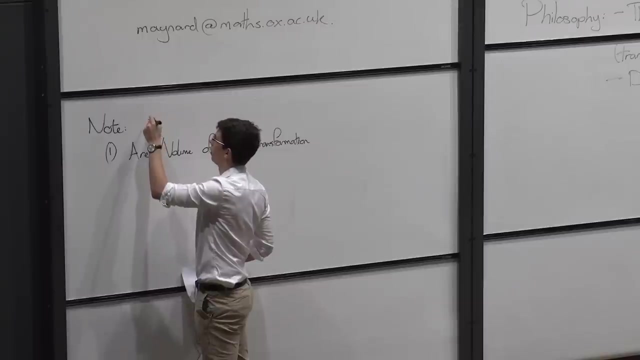 maybe I can understand properties of this linear transformation just from these abstract ideas, And so note that the area or volume of a linear transformation is linear in terms of the entries of the linear transformation. So maybe let's consider a matrix. So let A be a matrix. 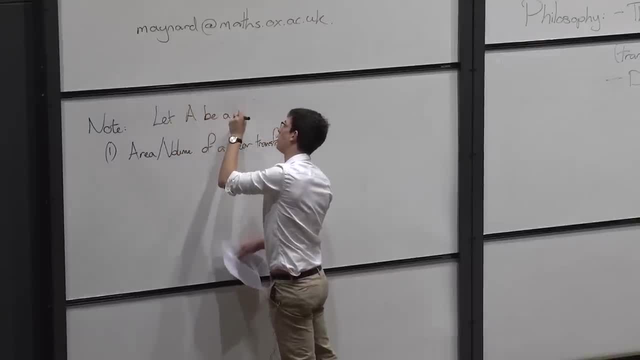 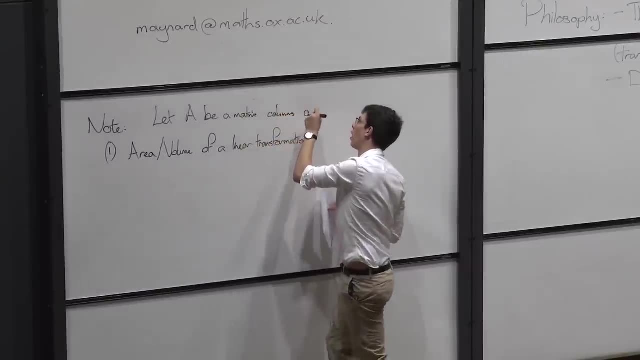 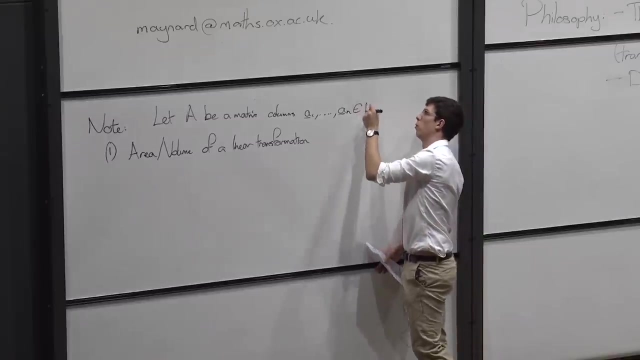 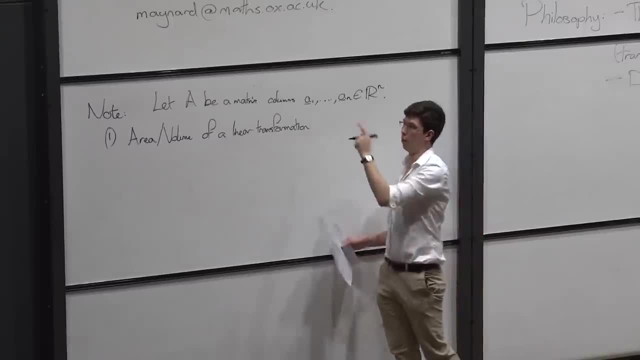 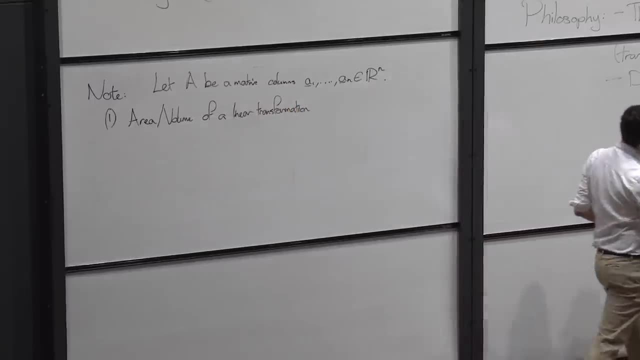 vectors in R to the n. so A's an n by n matrix And the volume of the image of, maybe, the unit matrix. if you will, If you're not going to say a function, you're going to, Are you going to say, for example, in the middle of the matrix, 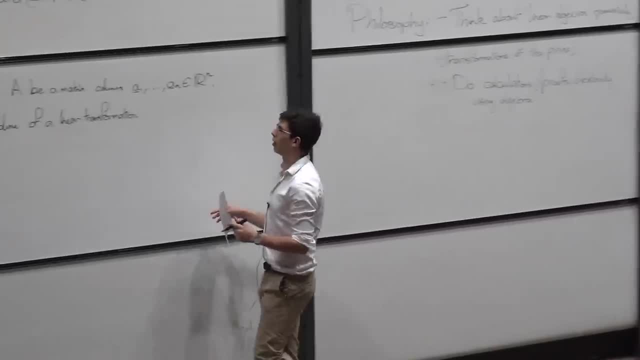 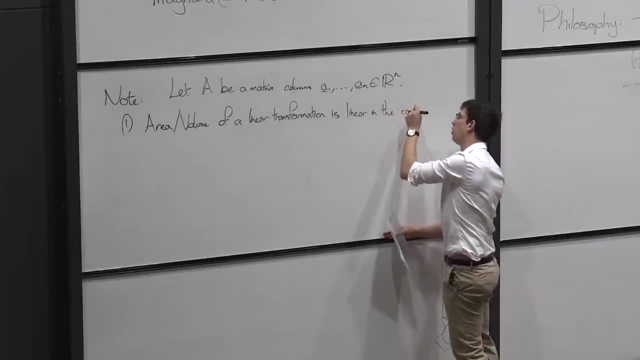 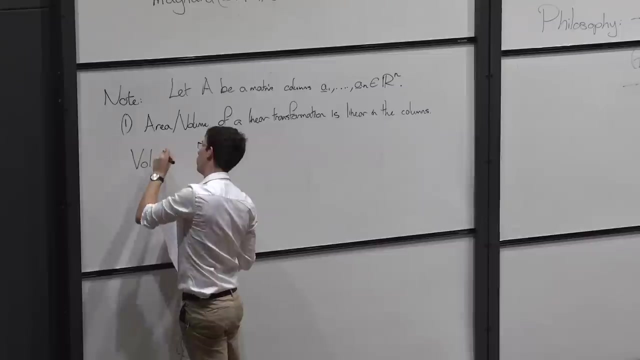 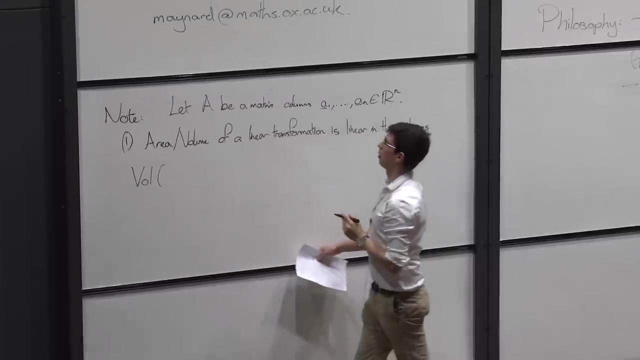 unit cube in r to the n is linear in the columns, So the volume of. so maybe a nice way for me to write this is: whenever matrix has columns a1 up to a n. I'll write this as a is equal to square brackets a1. 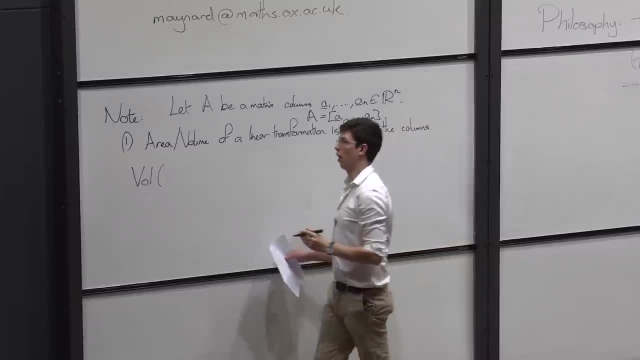 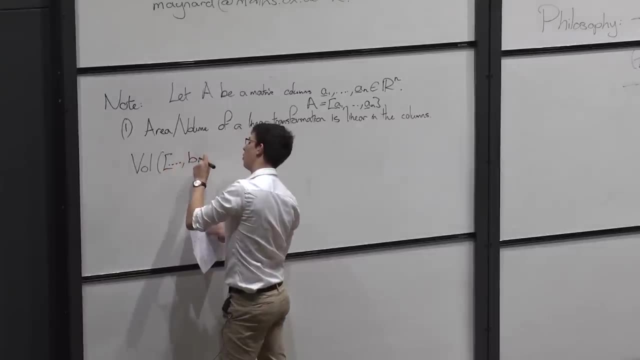 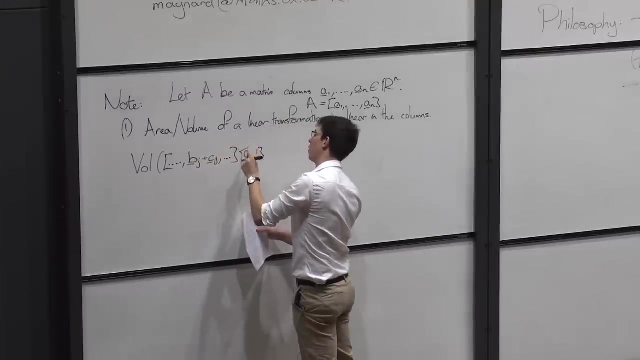 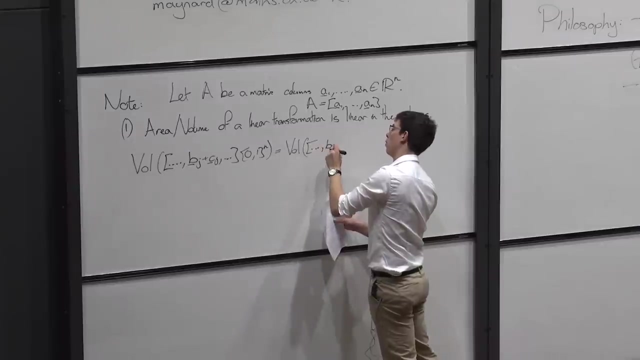 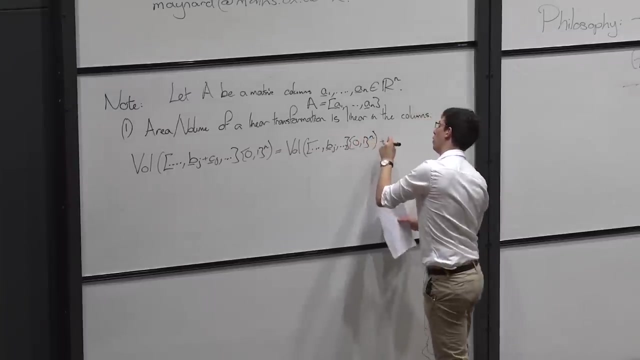 up to a, n and the volume of some columns. and if in the jth column I have a vector bj plus cj of the unit cube is equal to the volume where I have the same column with bj plus the volume when I have cj as the jth column. 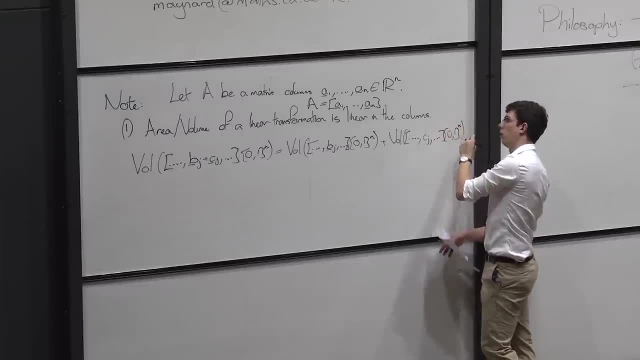 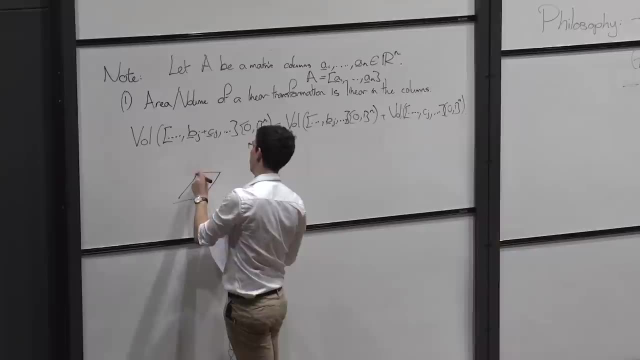 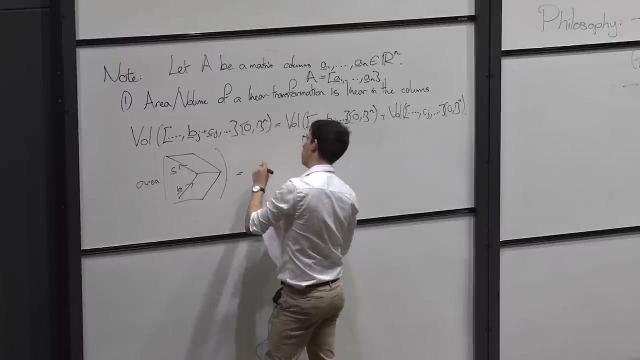 and this is basically based on the idea that the- if I have two vectors in the column here, a and b, so I'm thinking of this- is, or maybe I say, consistent. I'd call this b and c. the area of this is equal to just the area. 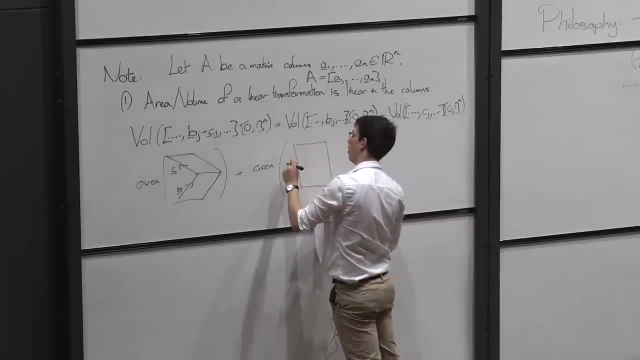 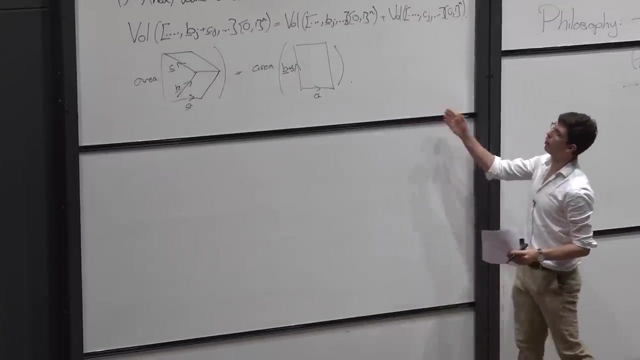 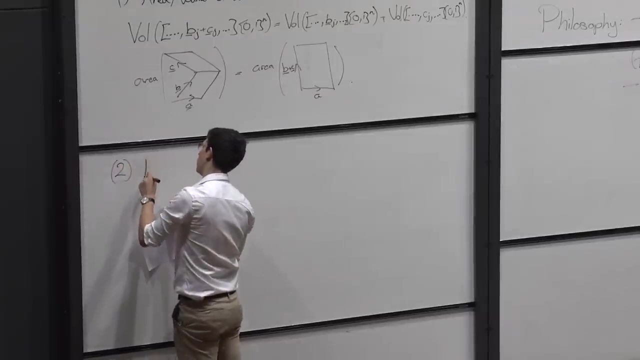 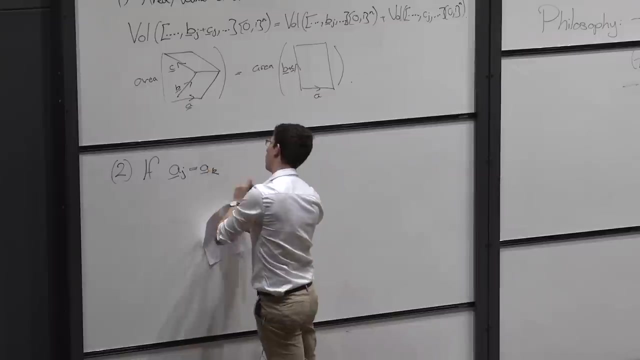 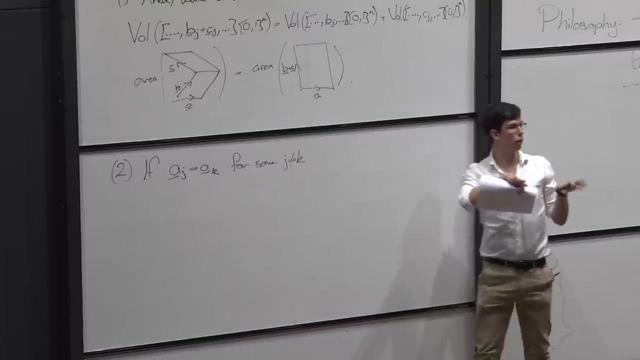 where I have the vector b plus c here, and so if that was a then I'd have just a here. So that's one property. A second and easy property is that if a j is equal to a k, for some j not equal to k. so two of the columns are the same. 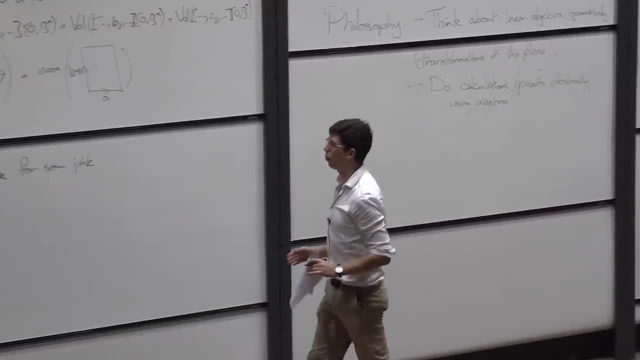 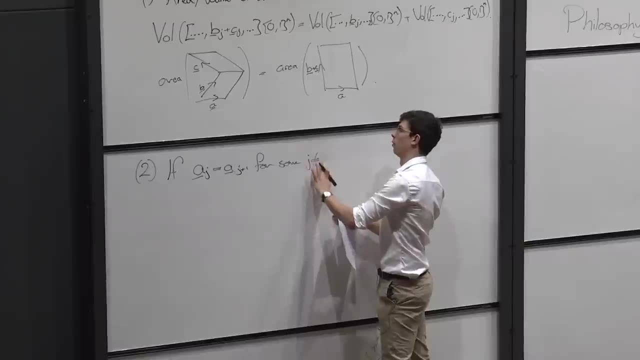 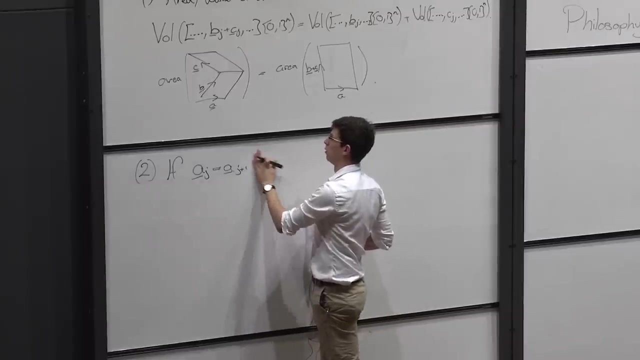 then the image of the unit Q will collapse. So maybe it's easiest if we just think about this- sorry for two consecutive columns- And then we don't need to worry about this. So I have two consecutive columns which are exactly. 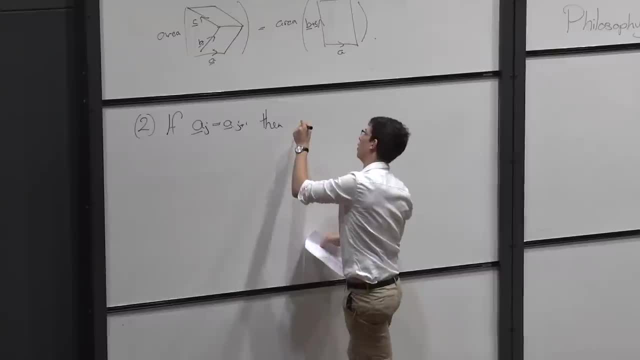 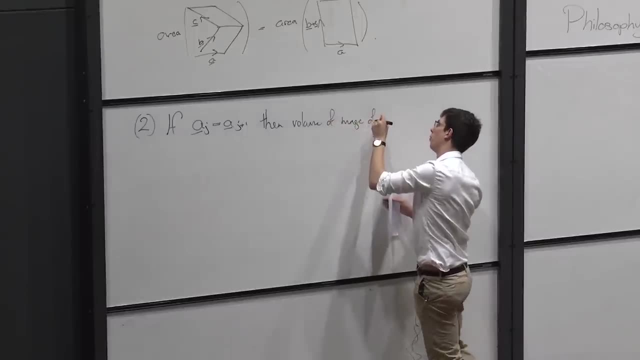 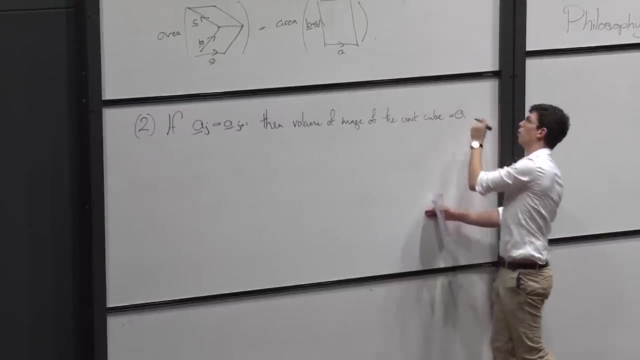 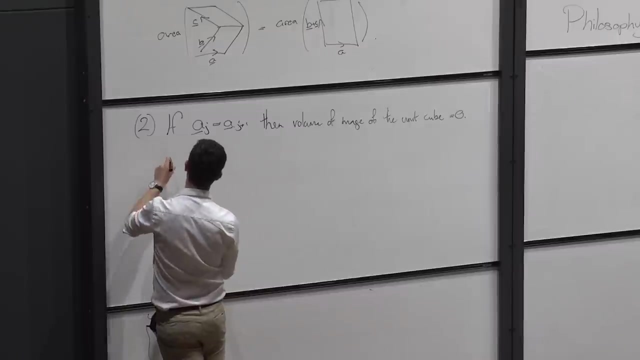 the same, Then the volume of the, So the image of the unit cube, is equal to 0.. And so again, I'm really thinking about this, And if I have two vectors being the same, they will just have two columns, aj and aj plus 1.. 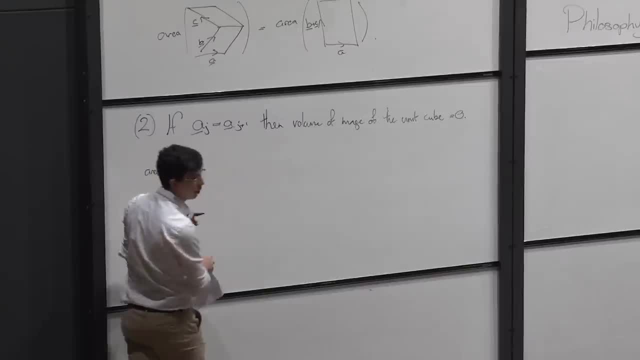 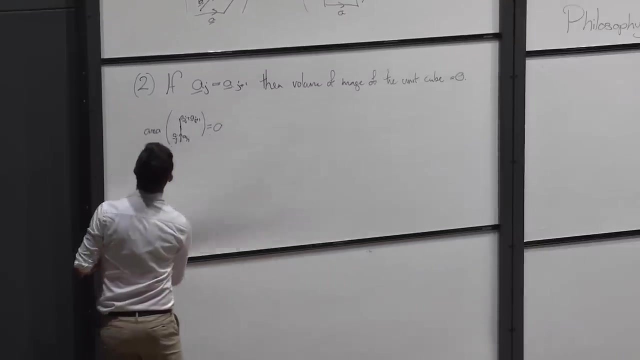 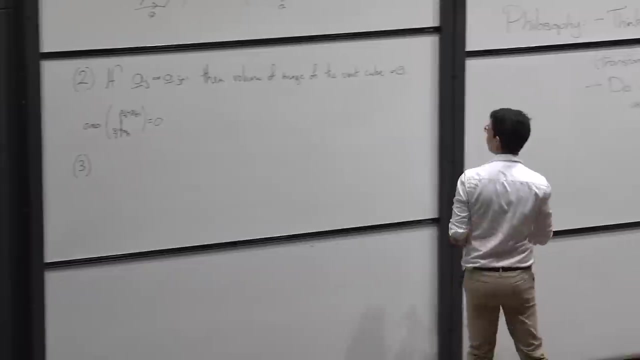 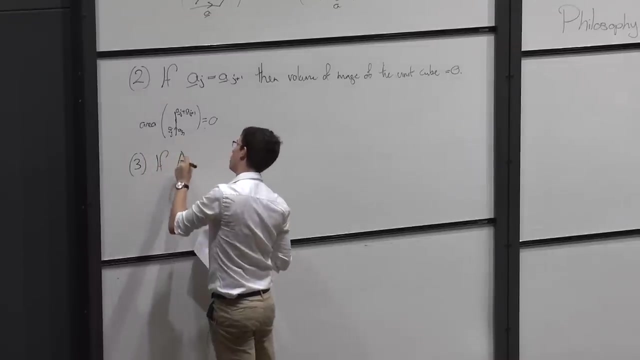 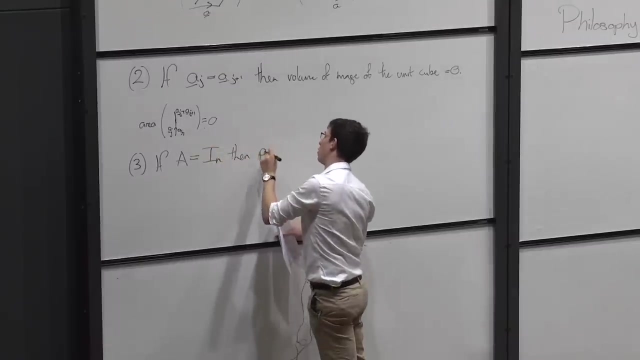 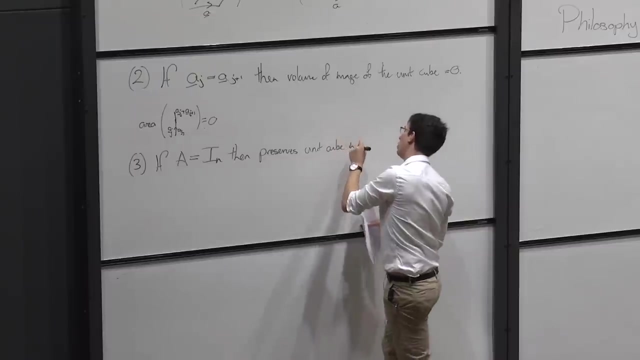 And the whole unit cube will just degenerate down to a line. And then a third property that we get from just looking at transformations on r squared is that if a is the identity matrix, then it preserves the unit cube in r to the n. 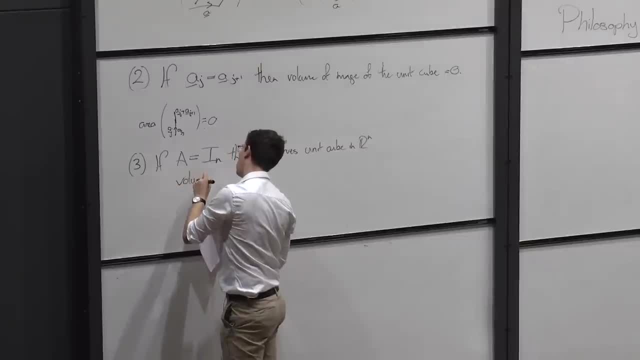 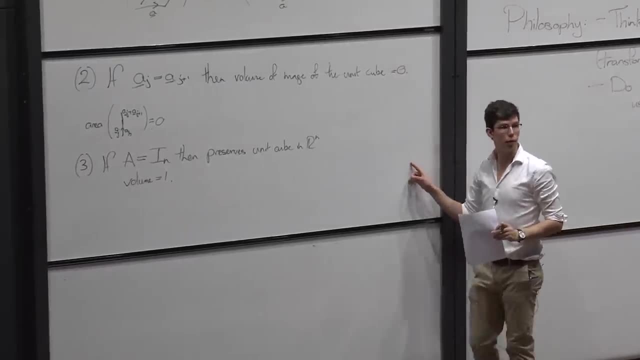 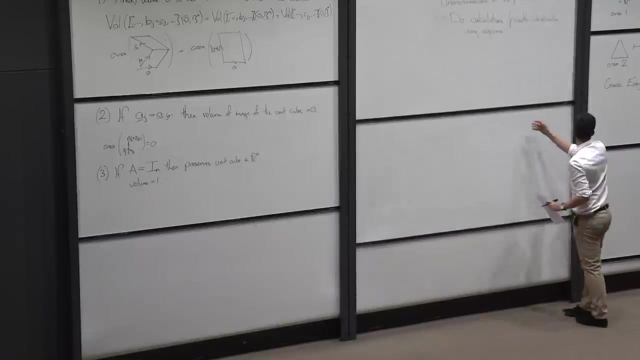 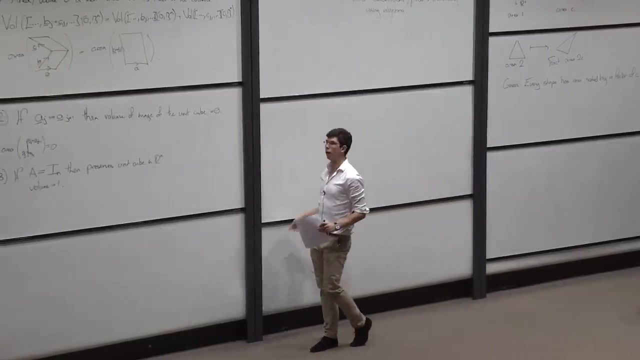 And the volume equals what? So I haven't necessarily proved any of these statements, but maybe they're all believable, And so what I want to say, then, is that these are properties that this determinant, I think, should satisfy, And these are all algebraic properties. 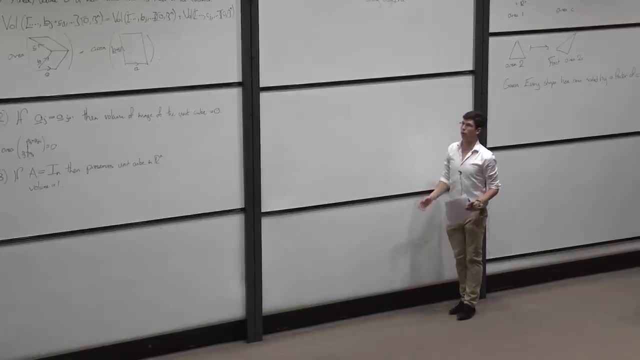 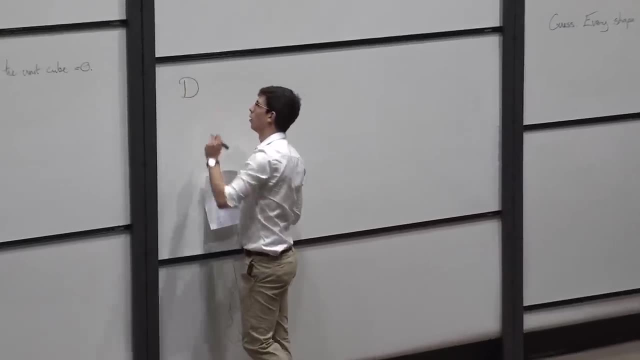 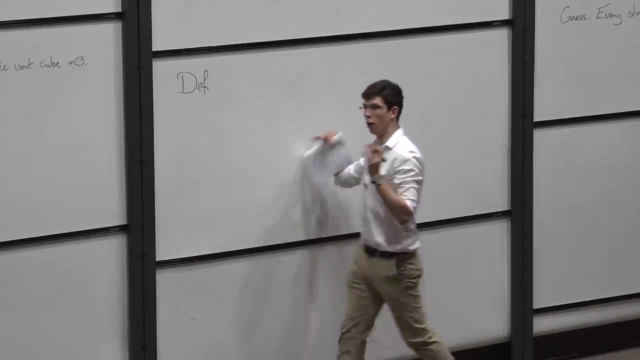 And therefore I want to study the determinant just through its algebraic properties. So this is going to To study the determinant. we're then going to define what it means for any map to be determinantal, which means it's going to satisfy the equivalent of these properties: 1,, 2,. 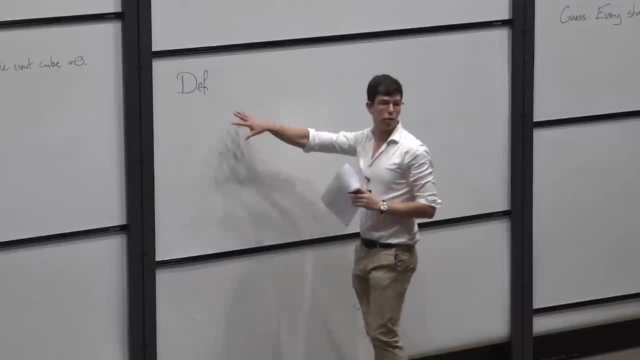 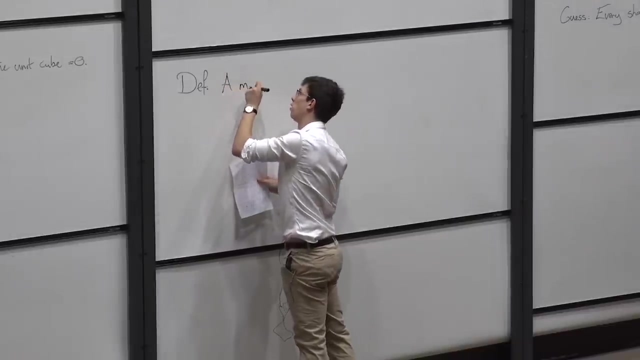 and 3.. So we're now going to start doing some concrete mathematics. Maybe before was some geometric motivation. So we're going to say if I take any function, I'm going to get a function. So I'm thinking of a function D And it's. 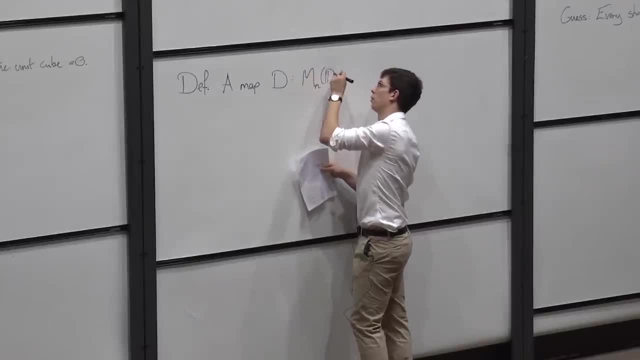 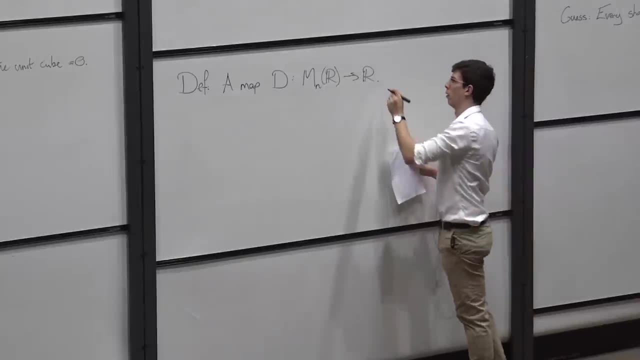 going to take its input n by n matrices with real entries And it's going to output some real value. And I'm going to call this map. I'm going to say it has the property of being determinantal, meaning it behaves like what I expect this determinant to behave. 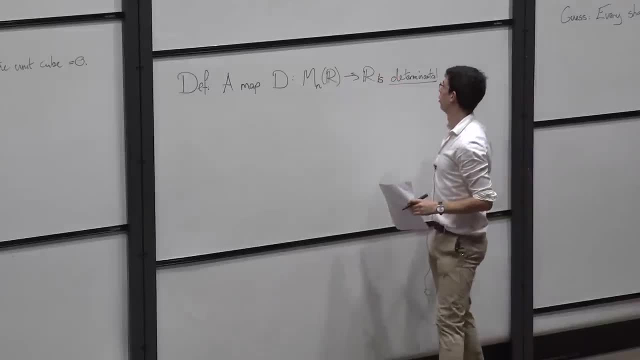 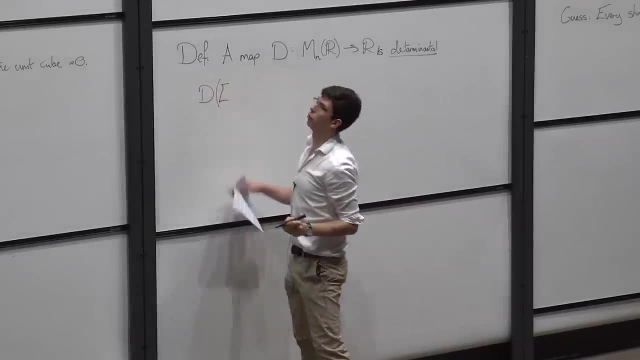 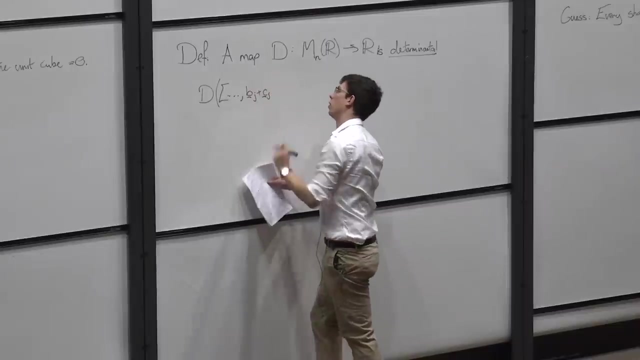 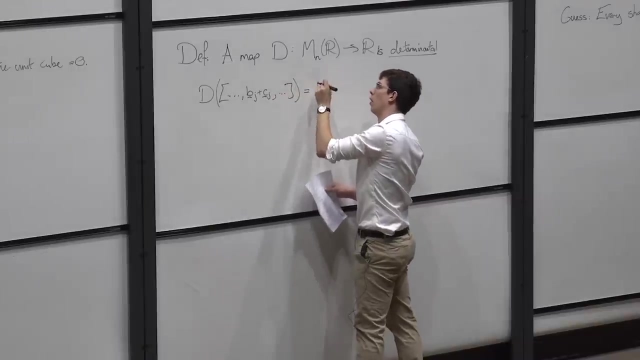 like If it satisfies the analogous properties. So if I think about my map acting on some matrix, well, I'll write it in the column form, And in the j-th column it has the vector bj plus cj. Then I want it to be equal to the determinant. 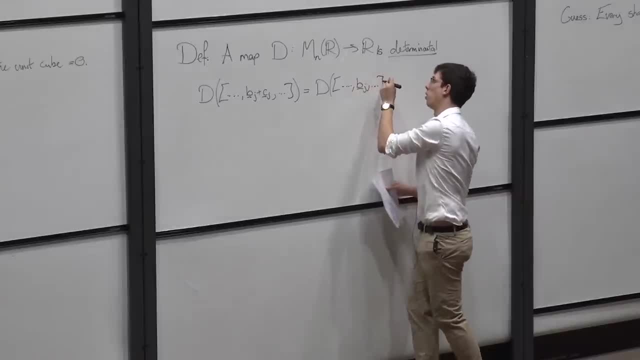 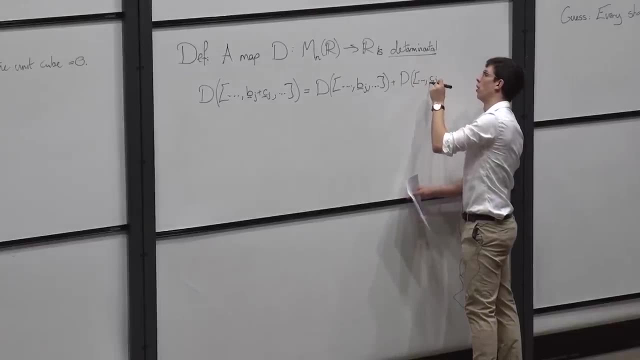 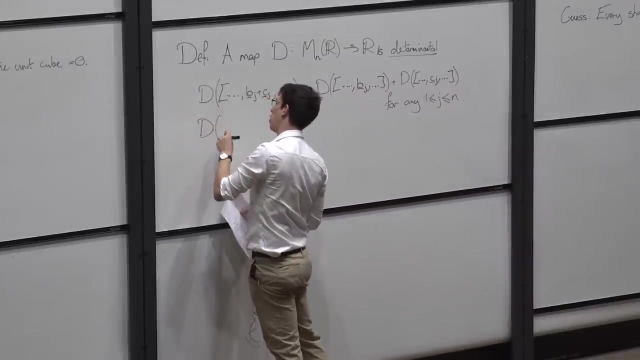 So j and j at j and the determinant at bj plus the determinant at cj For any choice of column index j between 1 and n. And similarly I want it to scale. So if I scale one column by a factor lambda, 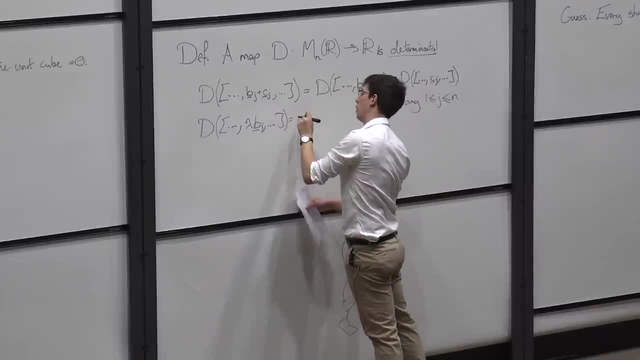 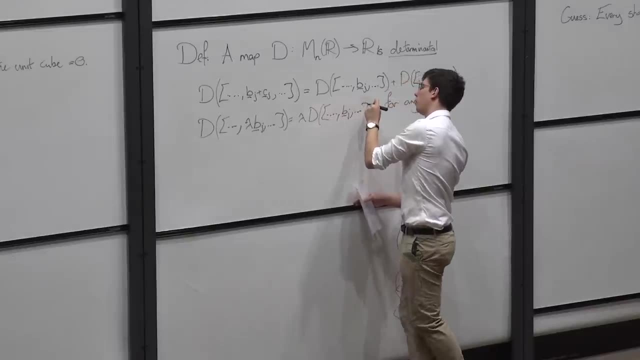 I want it to scale. So if I scale 1 column by factor lambda, I want it to scale 1 by factor lambda. then I just want this to scale the determinant by a factor lambda. so this is going to be the first property and I want this to be. 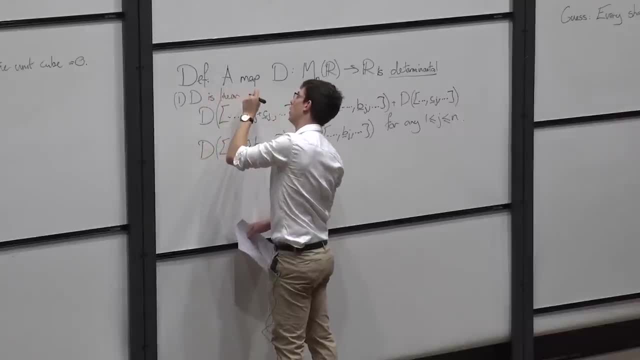 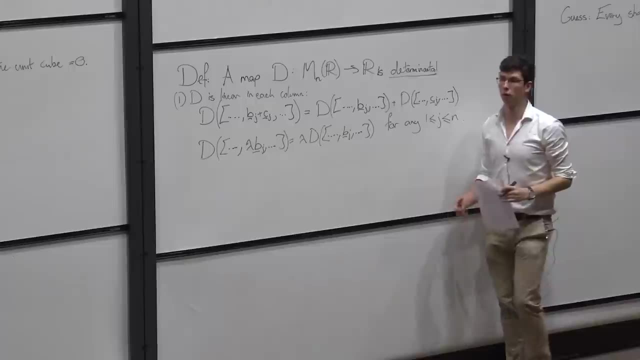 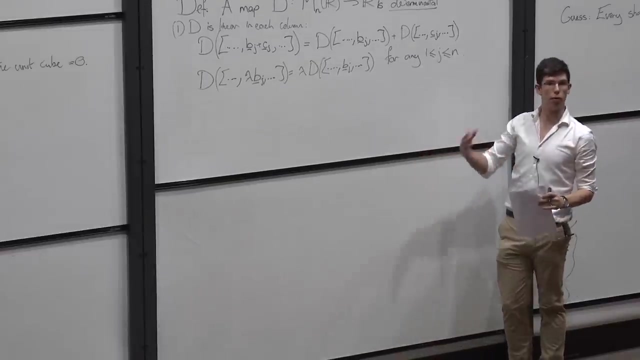 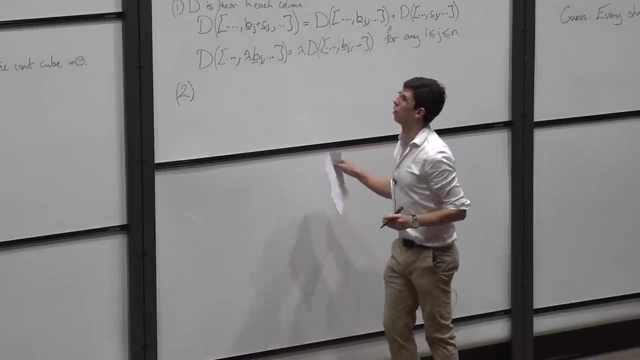 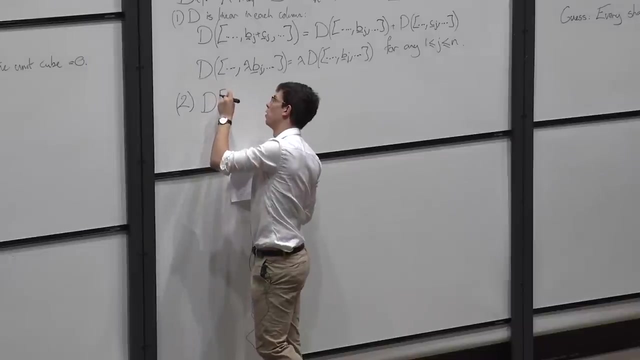 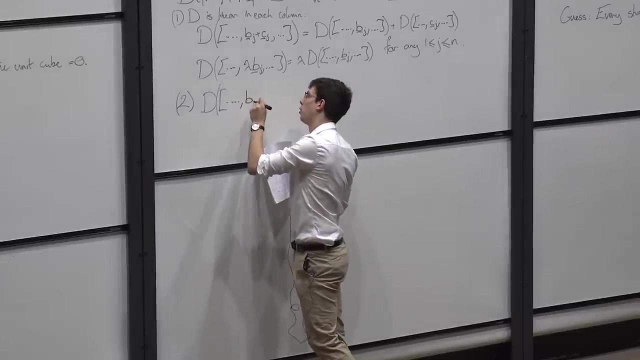 d is linear in each column, so this is basically the property that we guessed the volume of the image of the unit ball should satisfy for any layer transformation. the second thing is that I want d to have the equivalent of the second property here, that if I want. 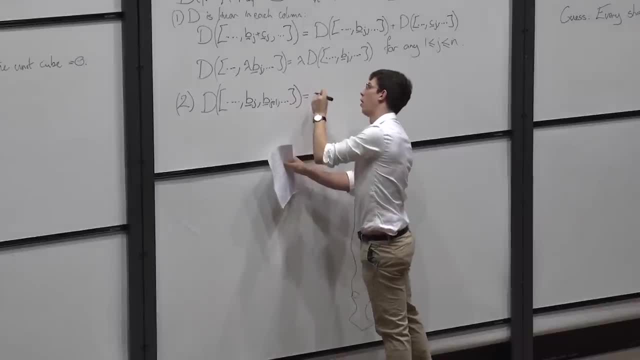 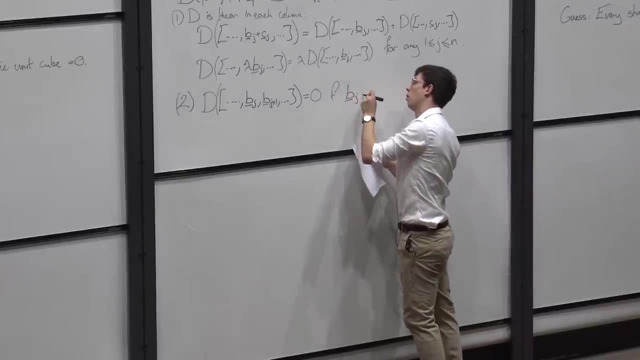 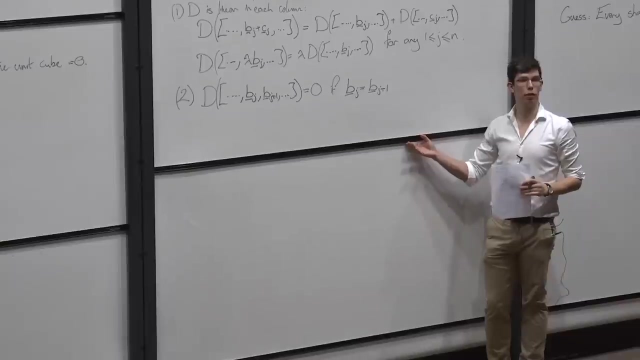 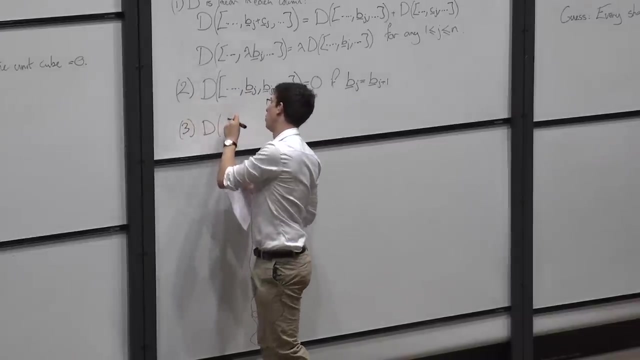 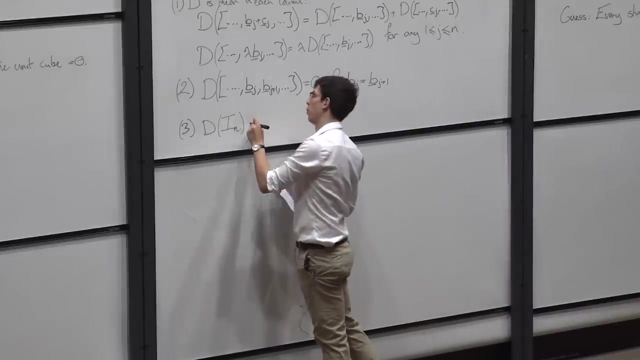 d to have the equivalent of the second property here, of the third property, then I guess I can put it inside. so if I evaluate it at some matrix and two of the columns are equal to each other, density matrix- I just want this to be equal to 1.. 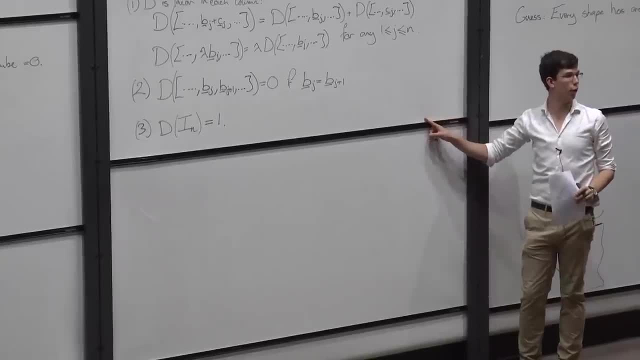 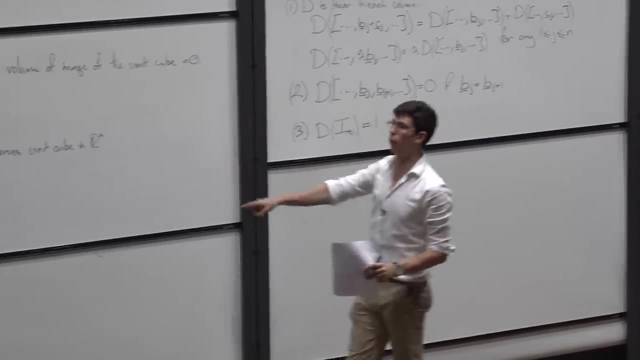 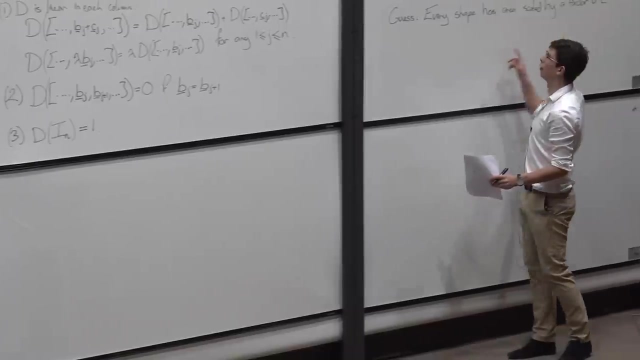 So this is a completely abstract definition of what it means for any function on matrices to be determinantal, And at least based on this motivation, we expect that the volume of the image of the unit cube should satisfy this, And so we think it should be an important property. 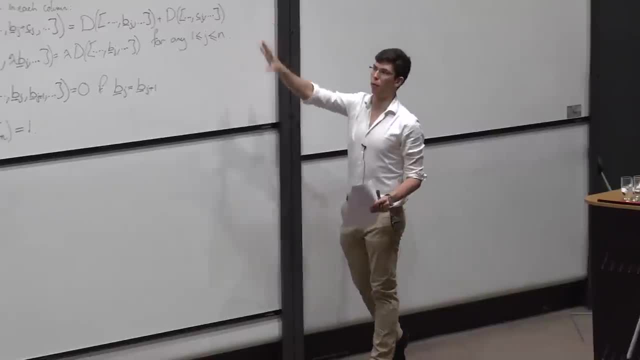 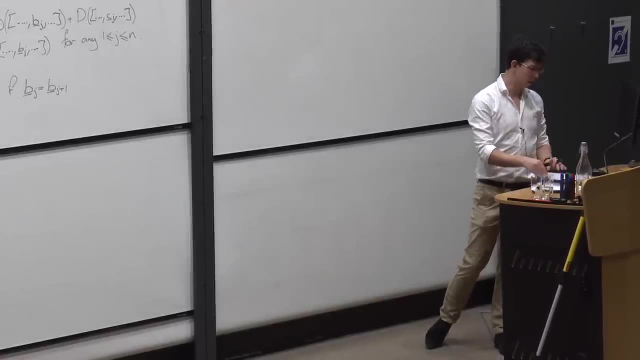 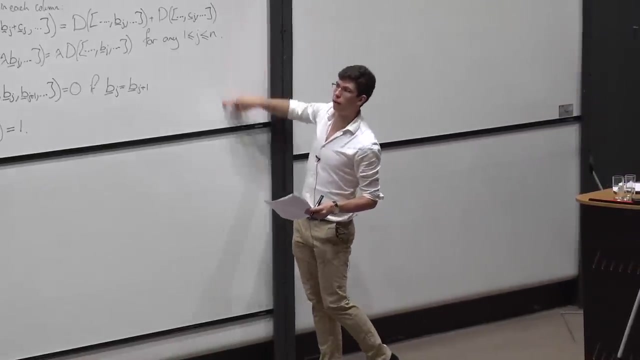 of any linear map, But now this applies in general to matrices in an algebraic way. So the first thing I want to do is to show you that if any linear map satisfies these properties, then it actually satisfies slightly stronger versions of these properties. 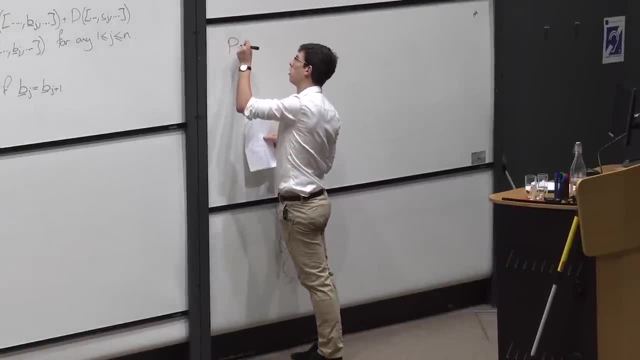 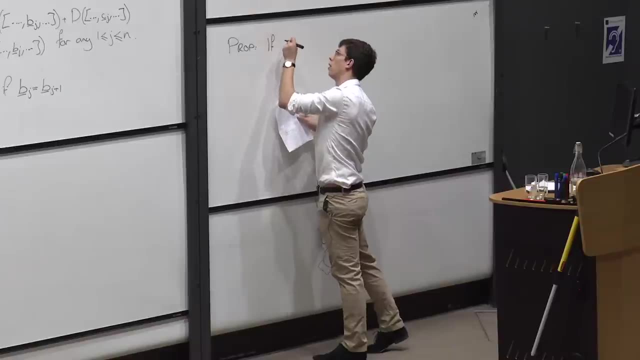 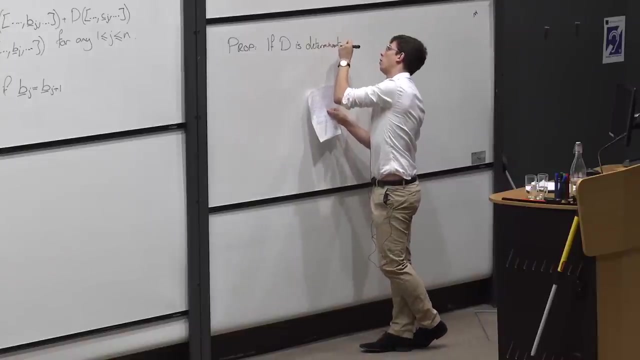 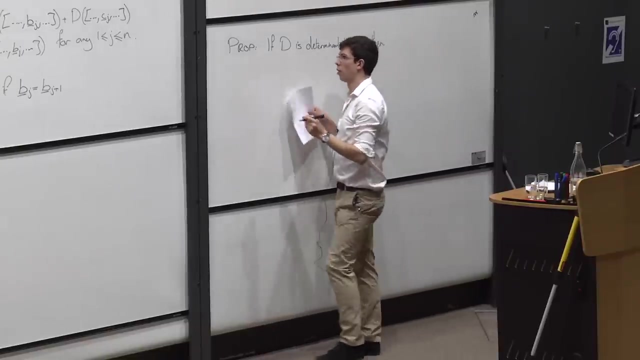 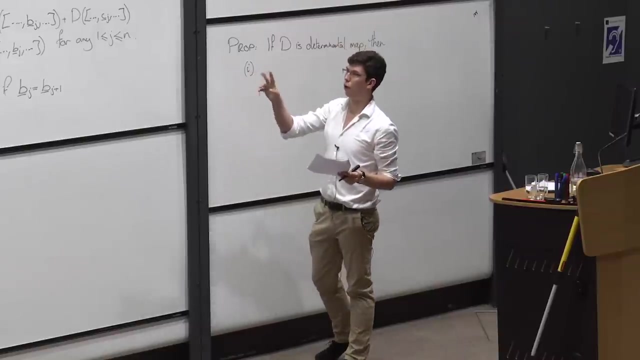 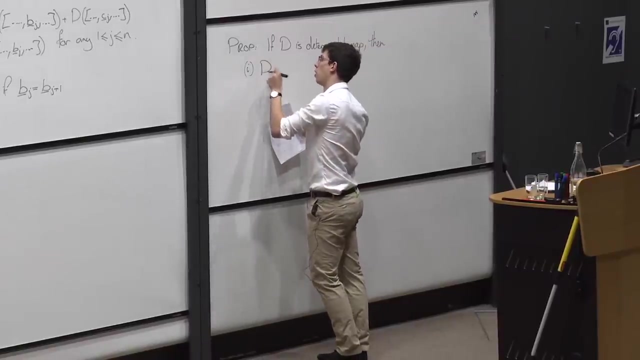 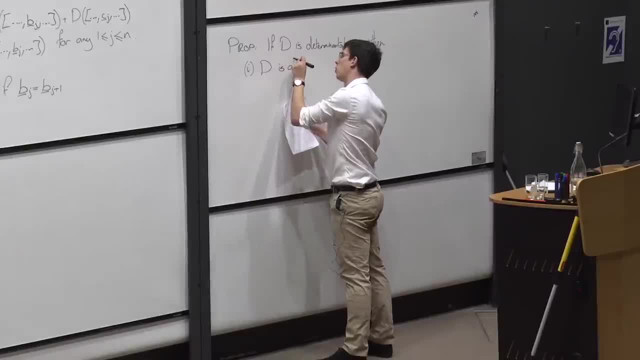 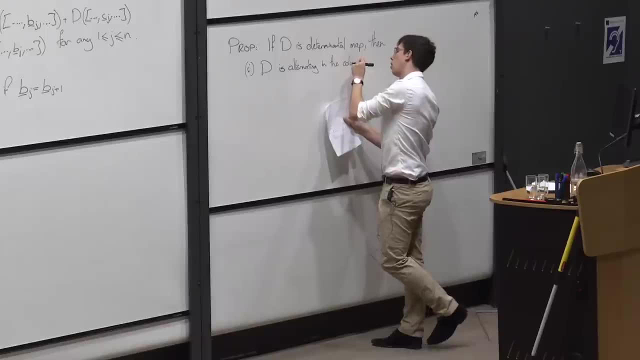 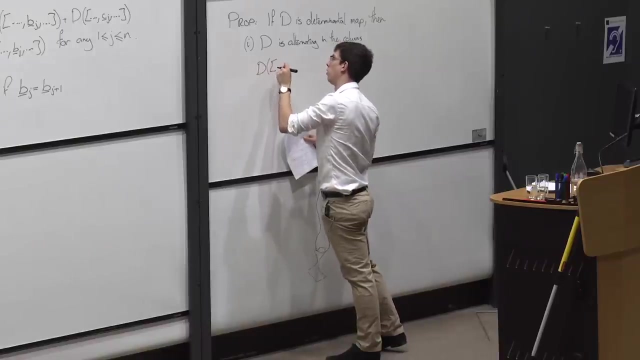 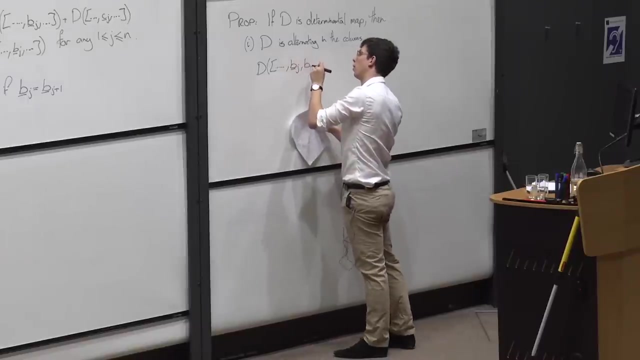 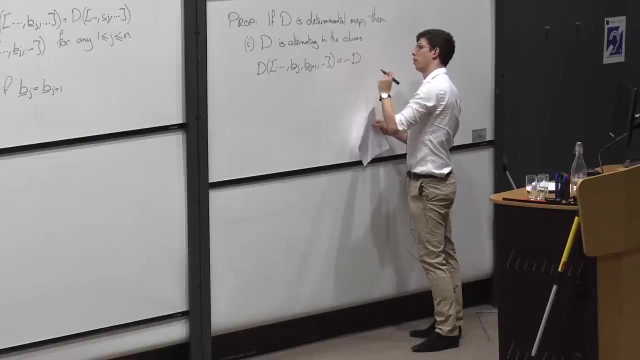 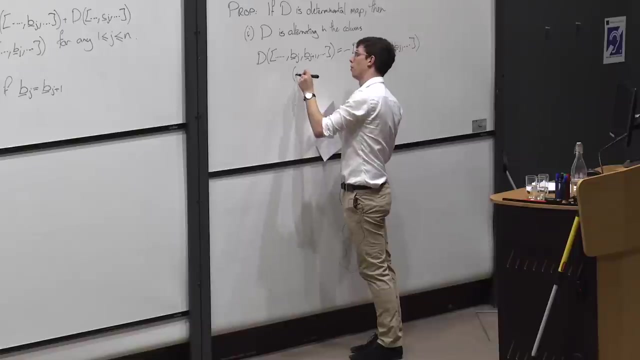 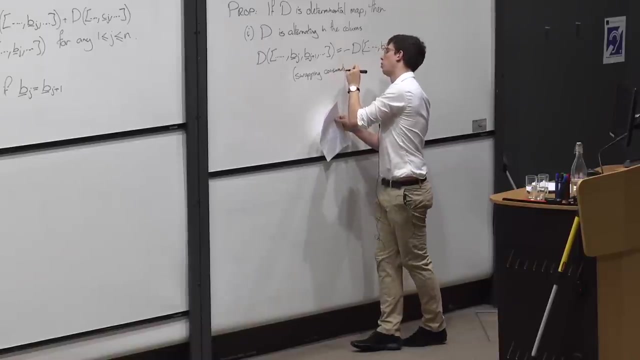 OK, OK, OK, OK. So let's say D is alternating in the columns, So D of some matrix with columns BJ and BJ plus 1 to minus the determinant of the same matrix if I swap the columns, So swapping two just changes the sign. 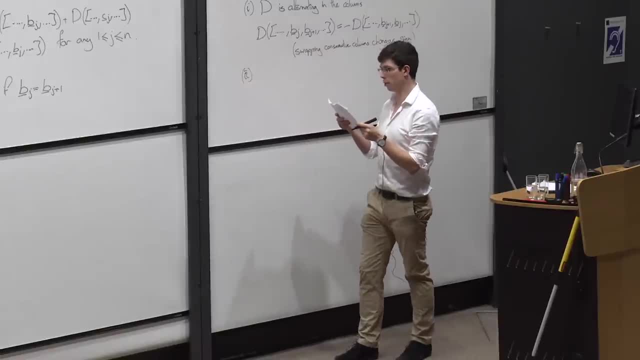 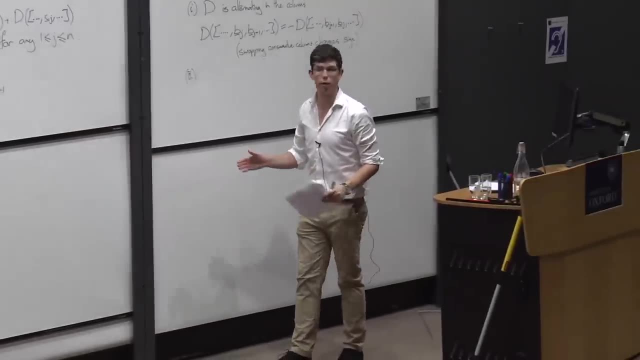 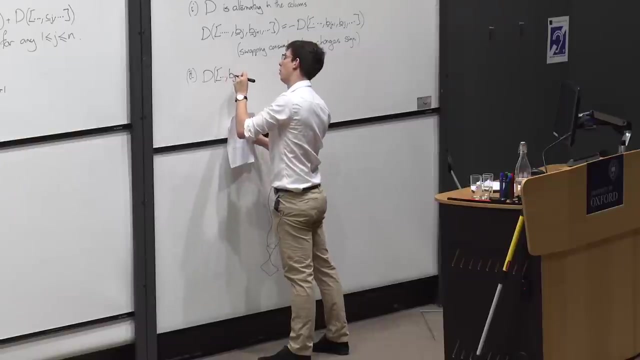 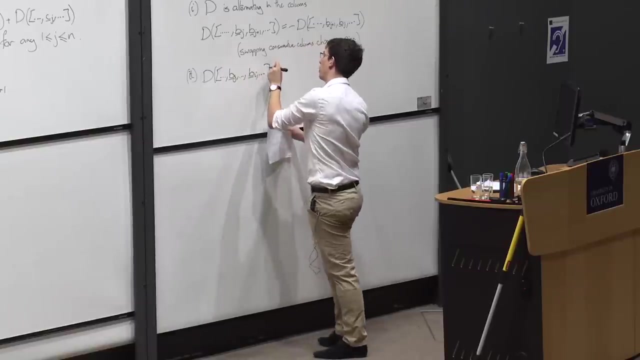 A second property is that: OK, I said the determinant is equal to 0.. Two consecutive columns are the same, But actually they don't have to be consecutive. so if I evaluated at some matrix with two columns, bj and bi, this is 0 if any two of the distinct columns 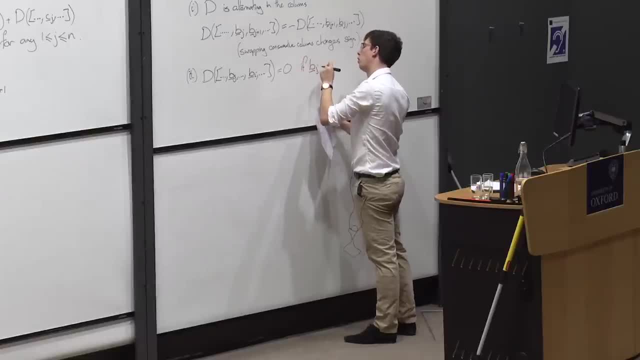 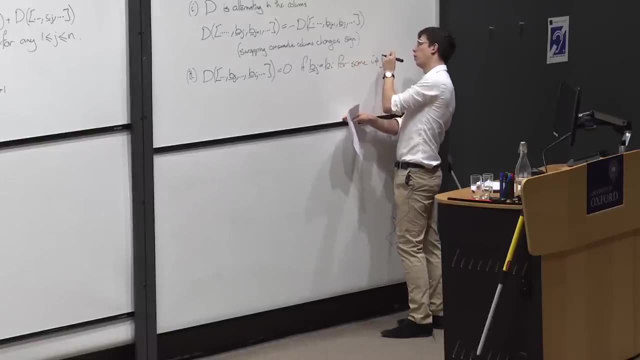 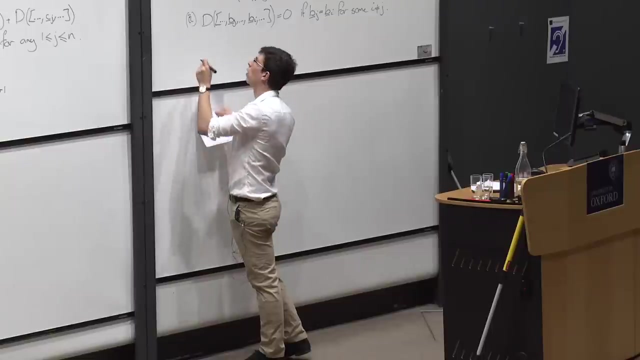 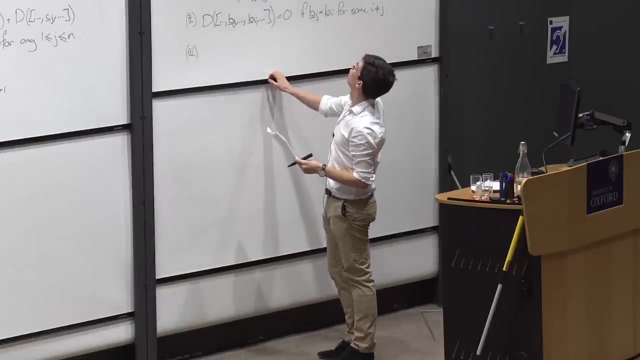 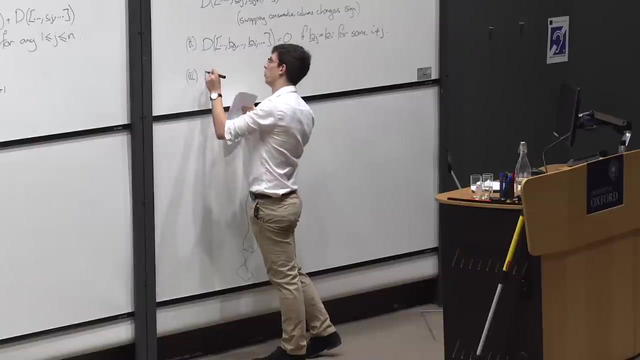 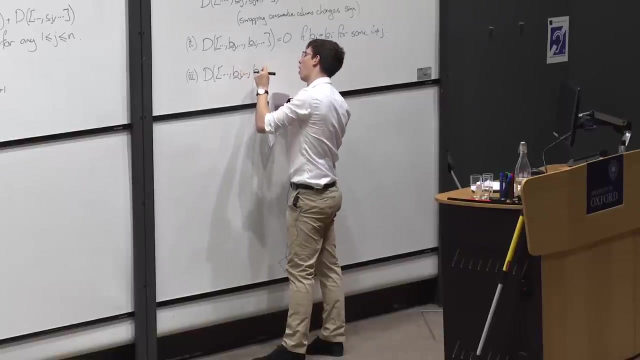 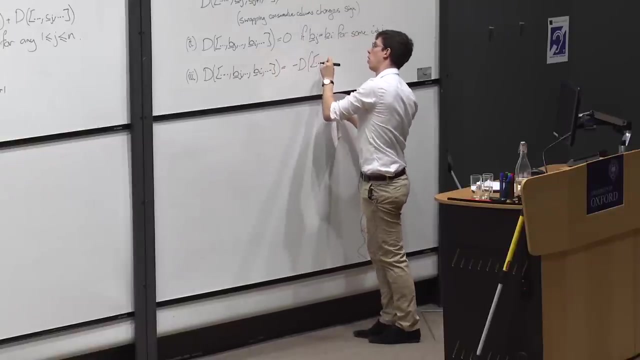 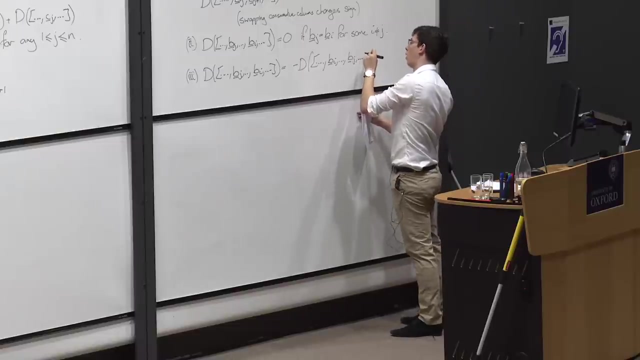 are the same And then a final property is a stronger version of it being alternating. but the first one was saying it's alternating in consecutive columns but actually I can do it for general columns. So if I swap any two columns I say whenever I swatch any two columns: 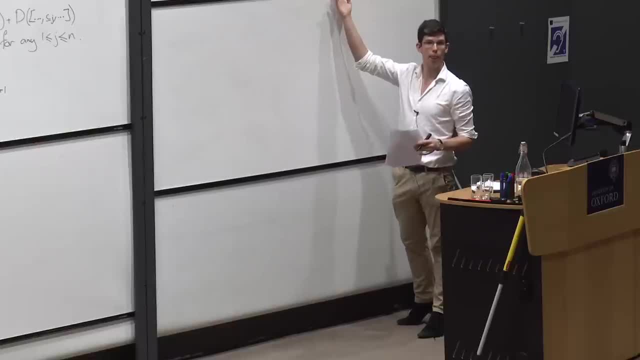 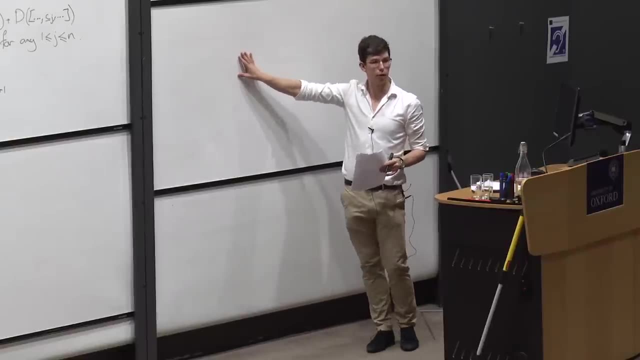 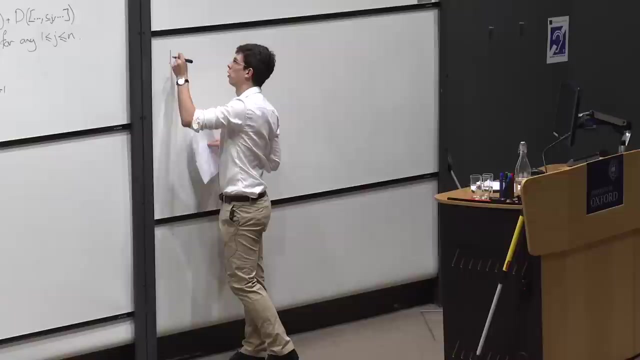 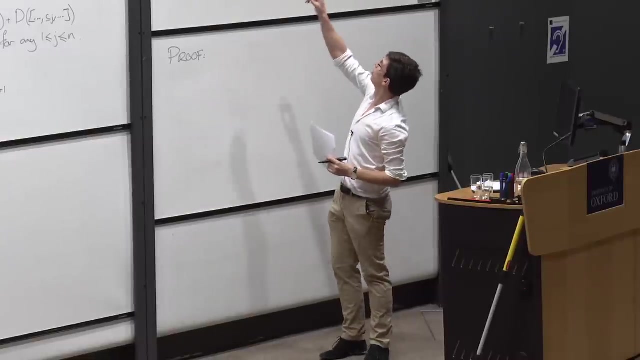 I just get exactly the same answer, but with the opposite sign, Just because it's in the깁. So let's go ahead and prove this proposition based on the properties that we've defined for determinant of the map. So let's start off with part one, because that really 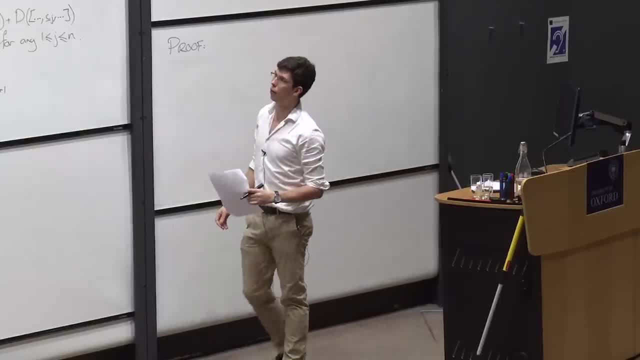 holds the key to the whole thing, And what I want to do is to think about d being evaluated, and what I want to do is to think about d being evaluated, really frankly, along the lines of very small strides in each of these factors. 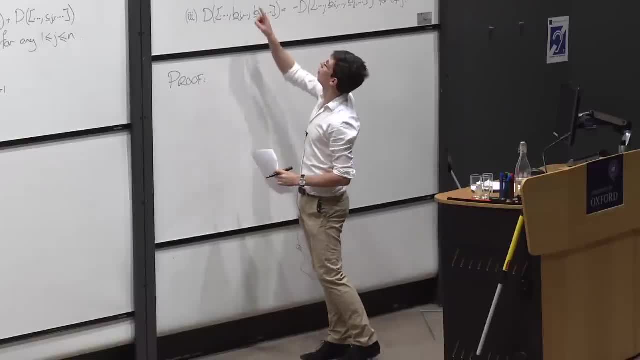 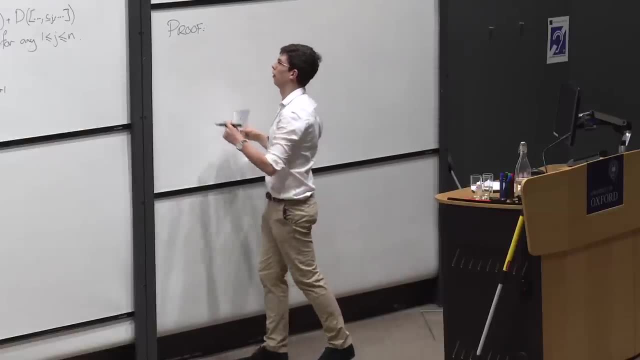 So if I replace it with 0 and quiet, because it's linking all to the illnesses, this would be PMT plus ten minus 1.. where I'm evaluating the jth common column and the j plus 1th column at vj plus vj plus 1.. 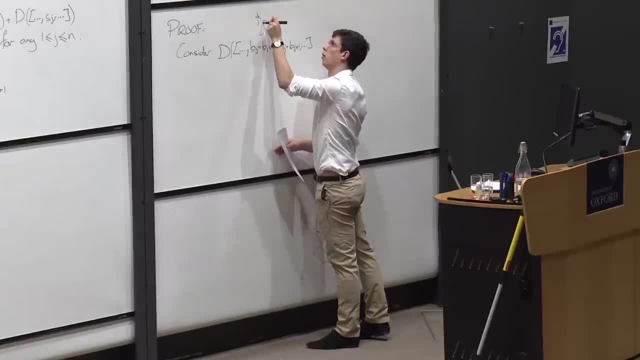 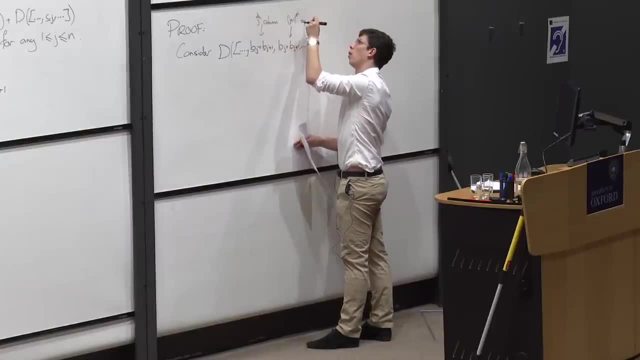 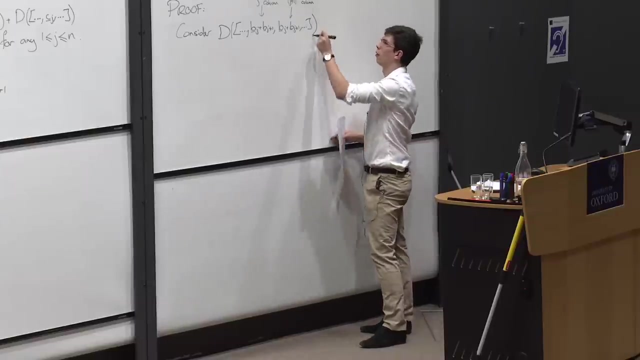 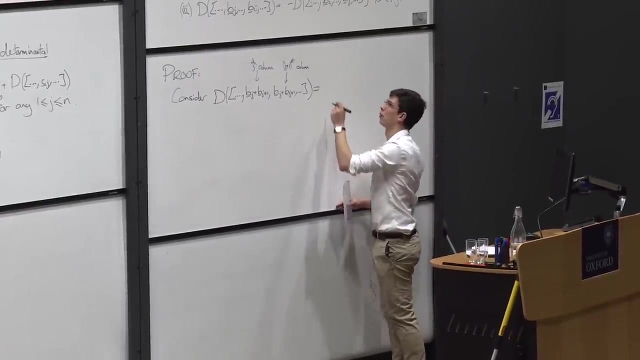 So here, this is the jth column and this is the j plus 1st column: j plus 1th column. So by linearity, I can expand this out. So what do I get? Well, I'll get 1t. 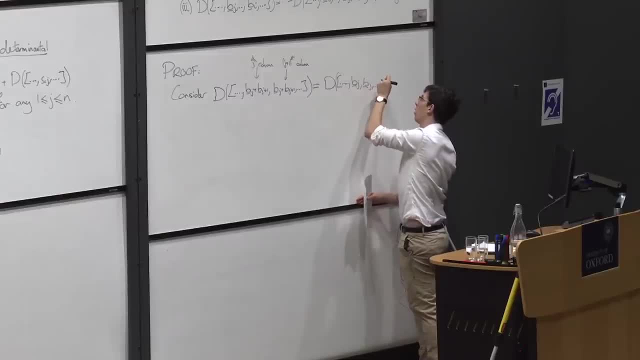 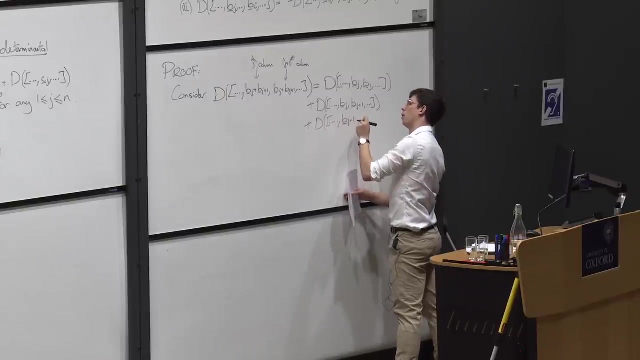 I'll get 1t with vj and vj. I'll get 1t with vj and vj plus 1.. I'll get 1t with jth column, vj plus 1 and j plus 1st column, vj. 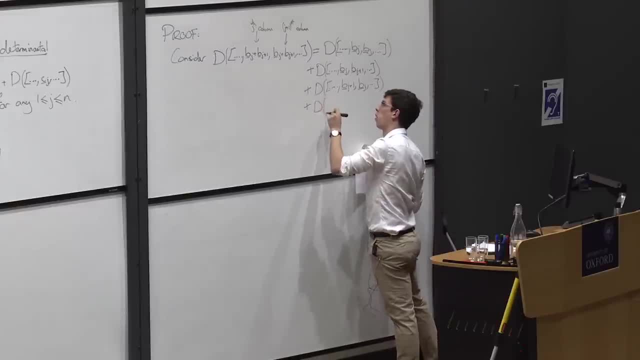 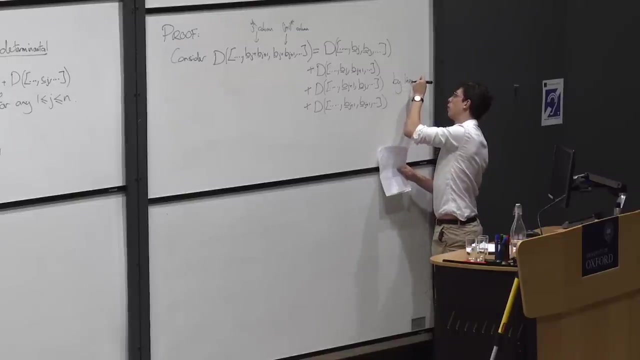 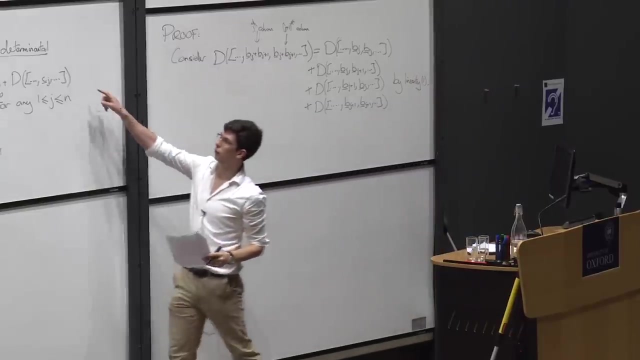 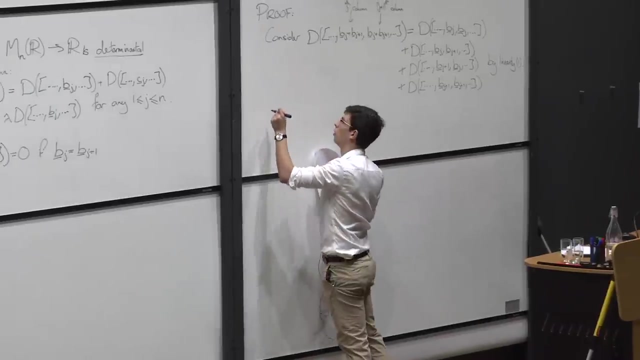 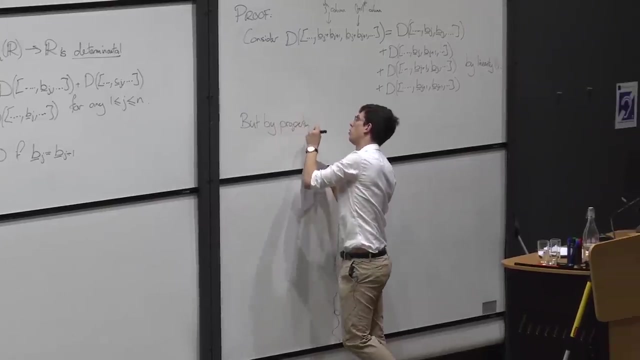 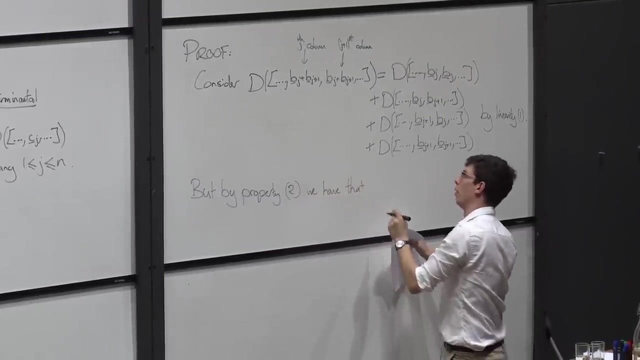 And then I'll get a final term with jth column, vj plus 1, and j plus 1st column, also vj plus 1.. So this is property 1. But by property 2, we have that, the left-hand side. 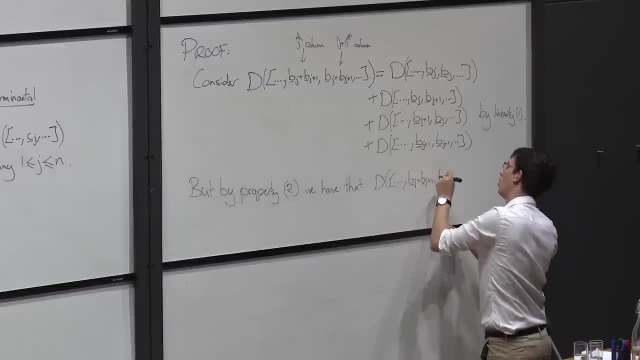 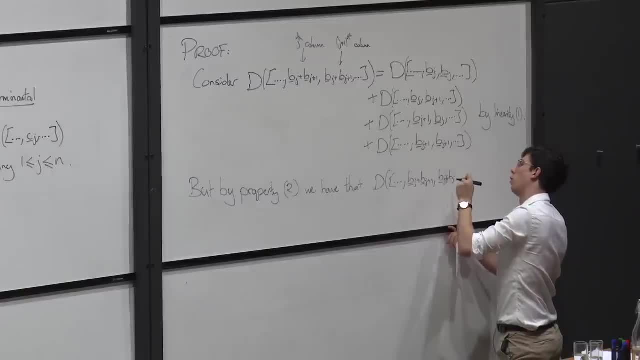 and then I get 1t is an unit of 2s and I get 1t. I get a maximum output here which is zero at one step. again, I get a constant at one step and I get a constant at one step to which I get the holiday. 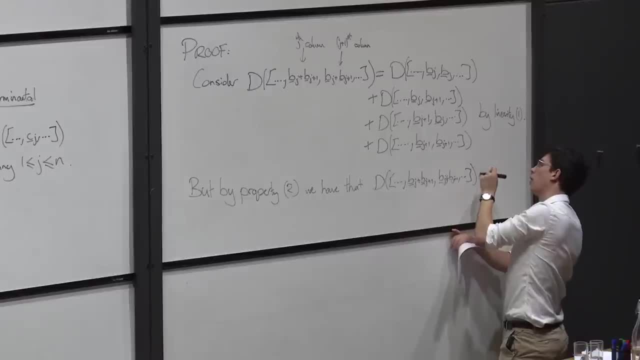 So I get positive luck. Let's assume the right side. I did that. I have one recycling and then I do that work. I did a great job with it, and then every lesson that I learnt away is equal to 0 because it has the jth column. 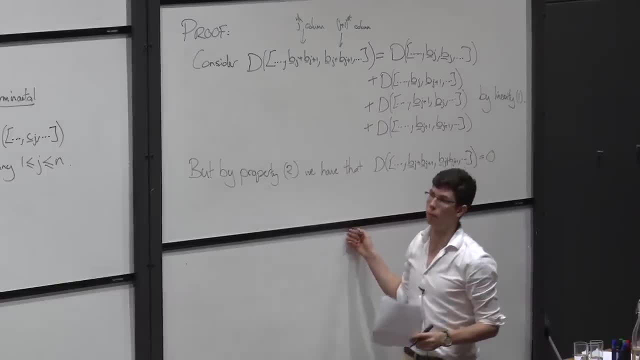 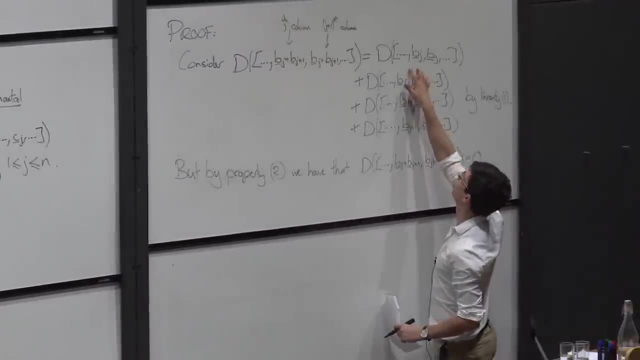 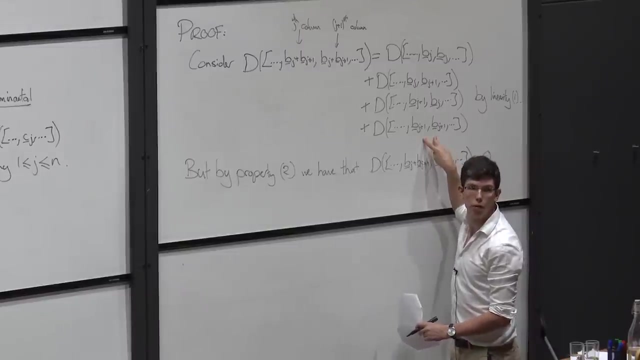 and the j plus first column being the same. So I'm just using this property, But moreover, we also have that in my expansion into four terms. on the right-hand side, the first term and the last term must also be 0, because these also have two columns which are the same. 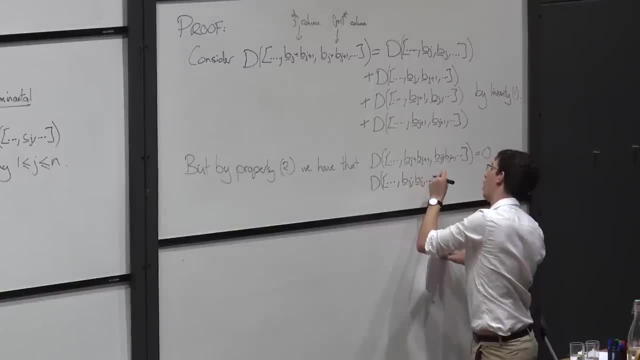 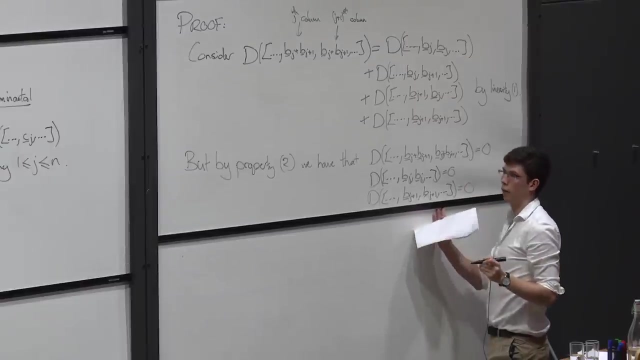 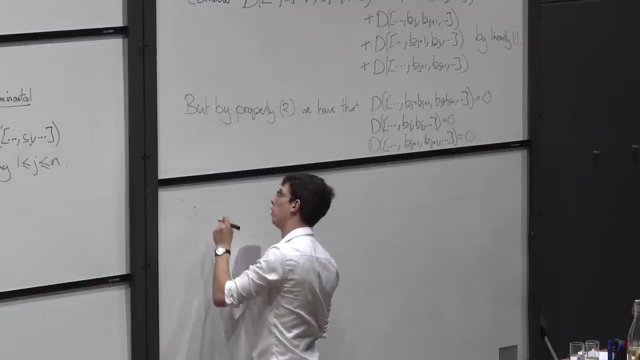 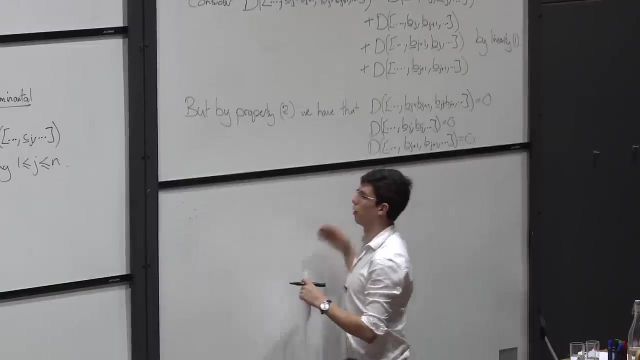 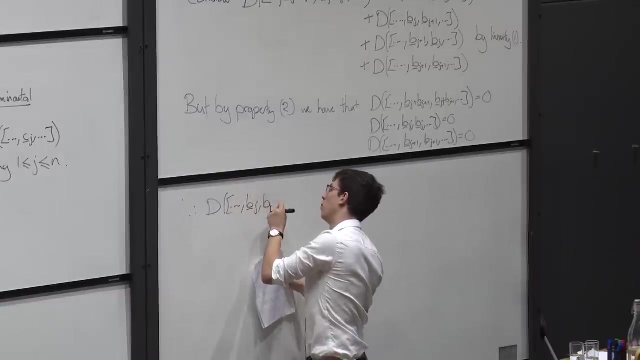 And so if I substitute these being equal to 0,, I therefore find that this is 0,, this term is 0,, this term is 0.. And so I just get that the sum where I have jth column be j, j plus first column be j plus 1, is: 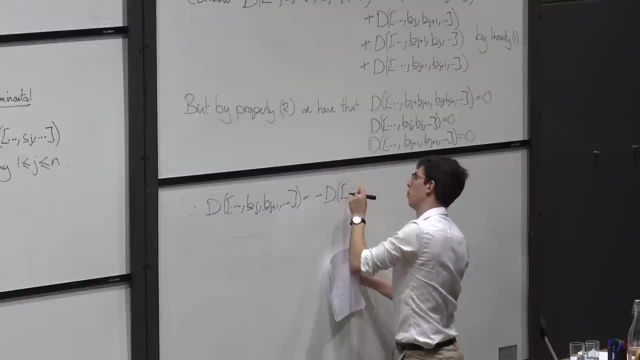 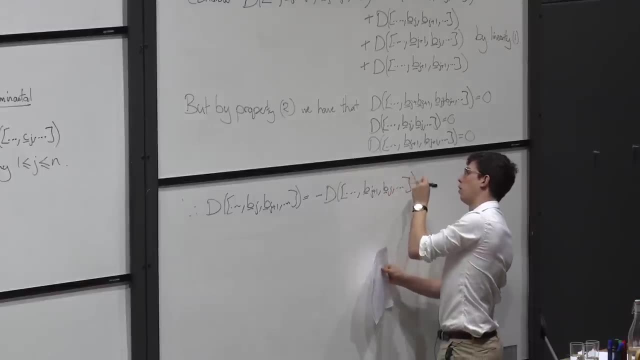 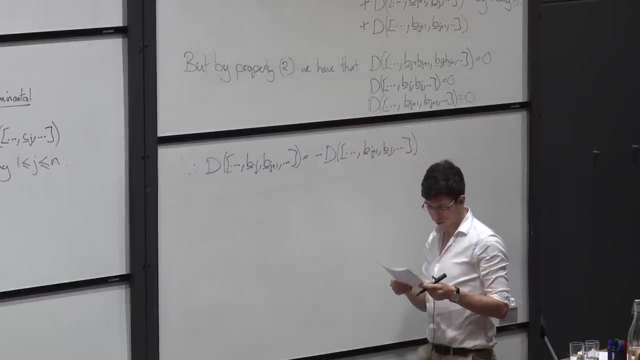 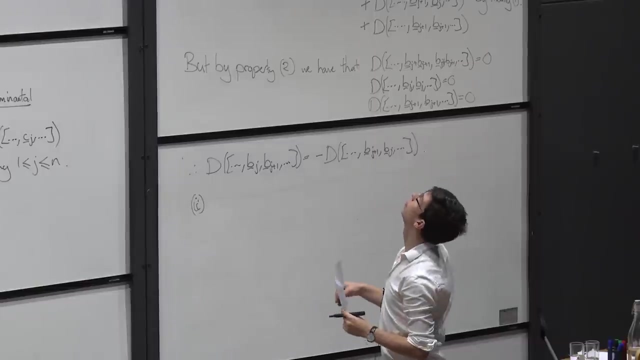 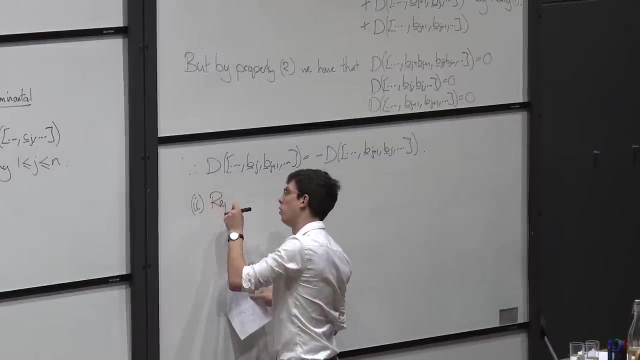 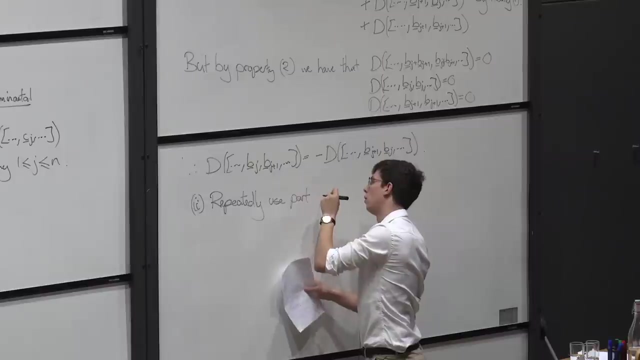 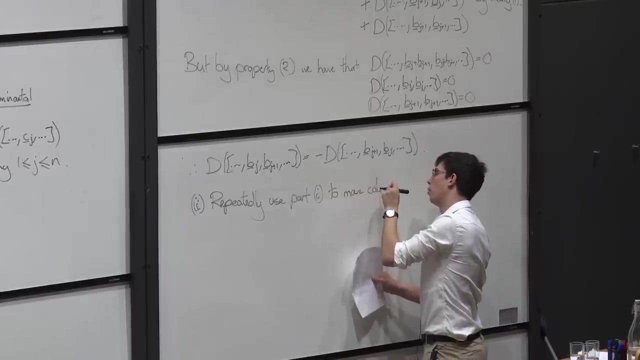 equal to the negative of exactly the same thing where I swap the two columns And so this gives the first property. So for part 2, I can now just repeatedly use part 1 to move column j to the left. So I can now just repeatedly use part 1 to move column j. 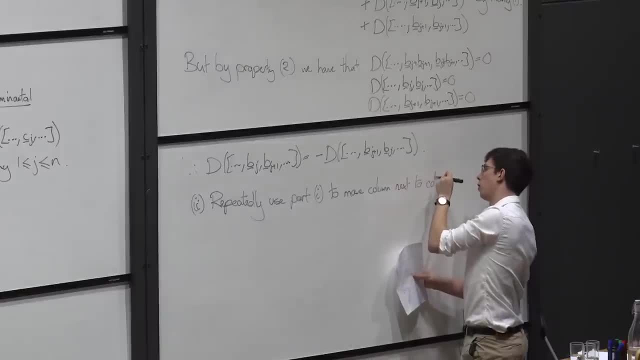 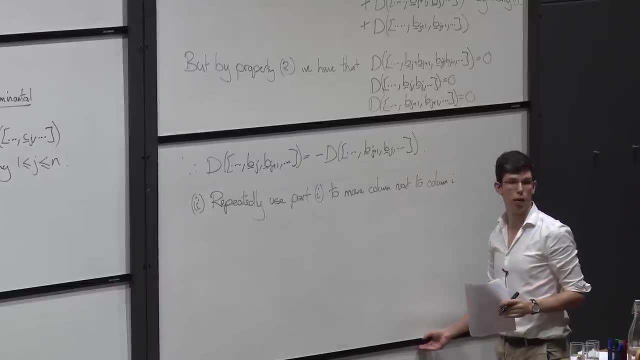 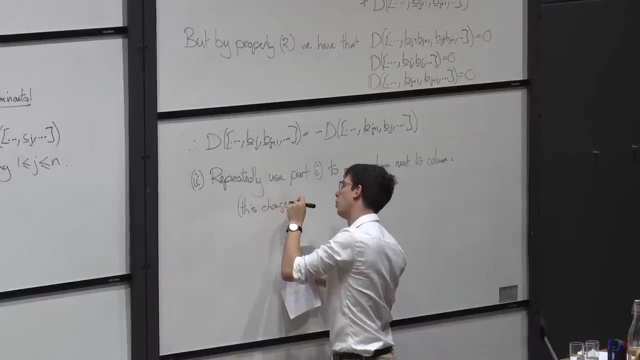 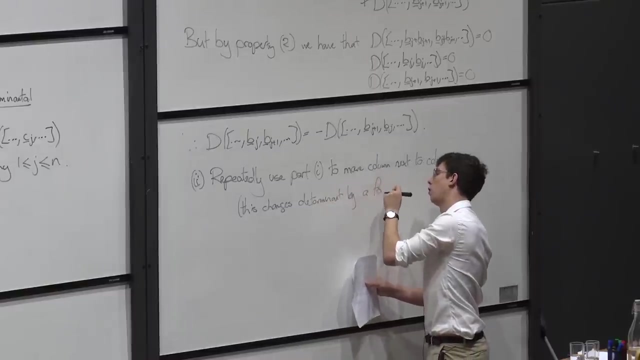 next to column i And I change the determinant just by a factor of plus or minus 1.. But then the determinant has to be 0 because I have jth column be j plus 1.. So I can now just repeatedly use part 1 to move column j. 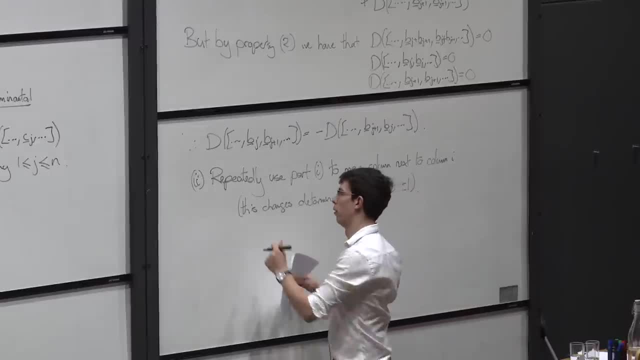 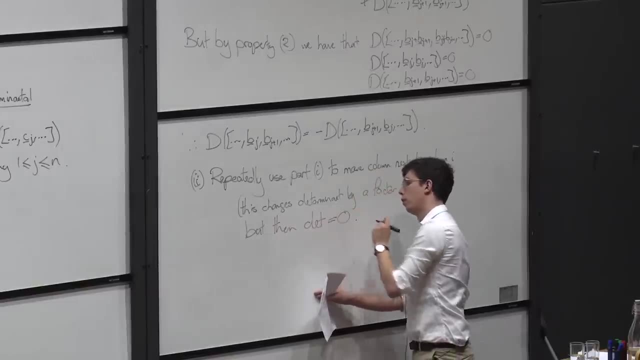 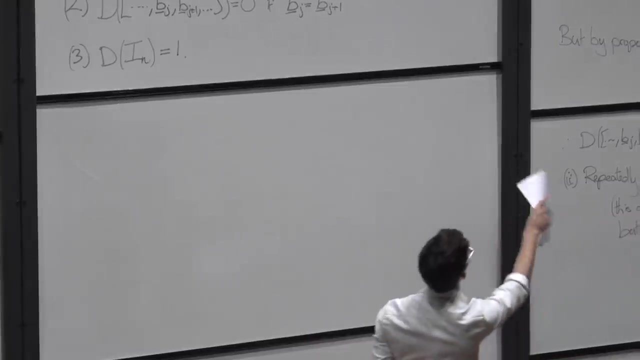 next to column i, And I change the determinant just by a factor of plus or minus 1.. But then the determinant has to be 0, because I would have two consecutive columns being the same, And so that instantly gives the final property. And so now for the third part of part 3,. 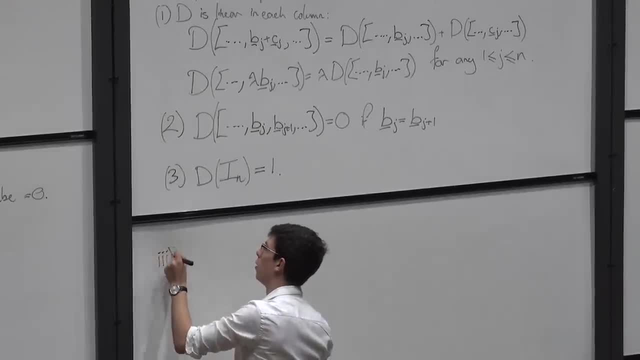 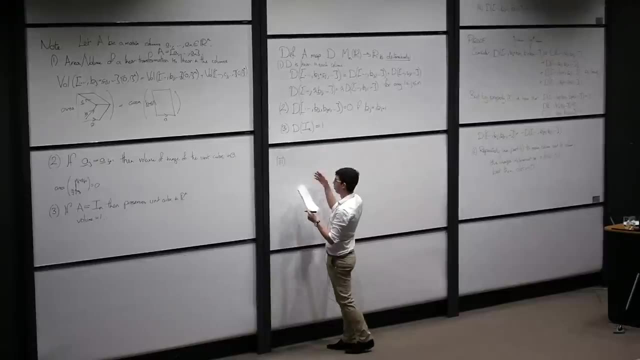 there's a few different ways I could do it, But I can essentially follow exactly the same proof as part 1, with this part 3.. Except that, again, if I want to add an interval in it, which is now called the productresse. 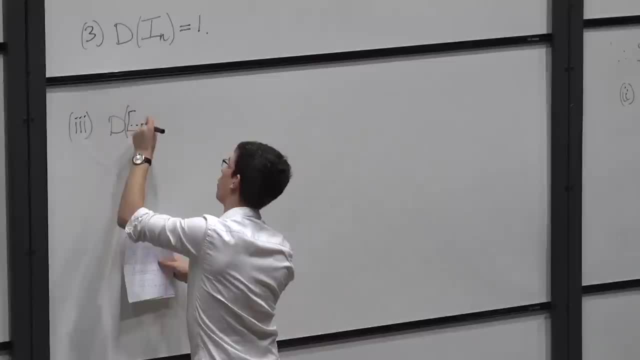 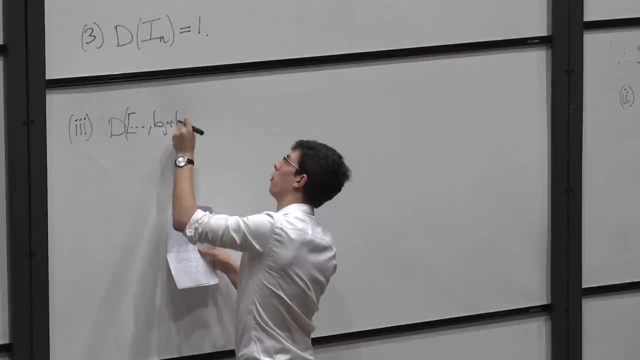 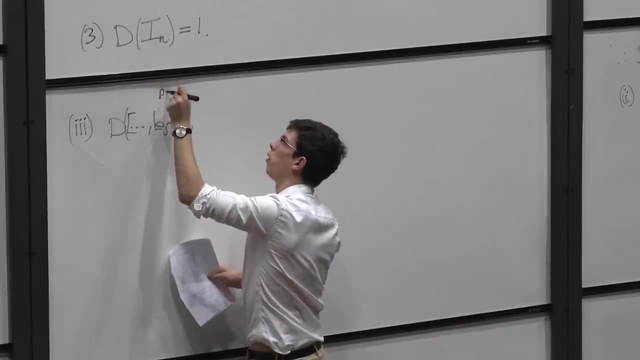 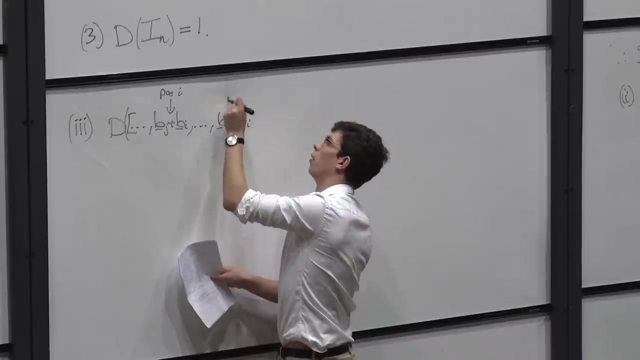 I can do thisron as I move thejis, So I can think about evaluating my matrix, where I'm now evaluating it with columns bi and b, j in position i and bj plus bi also in position j, and so that's essentially my rainbow method. 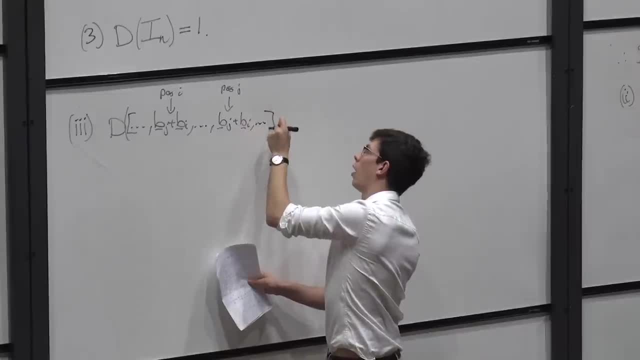 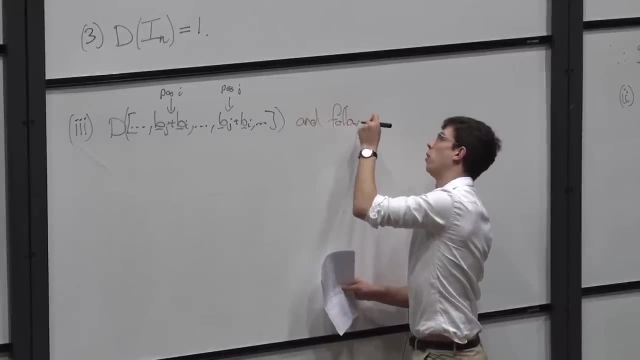 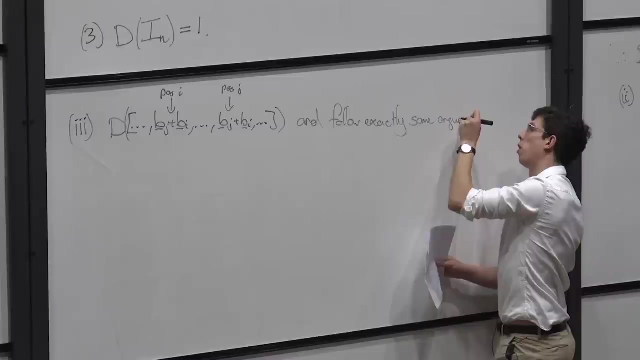 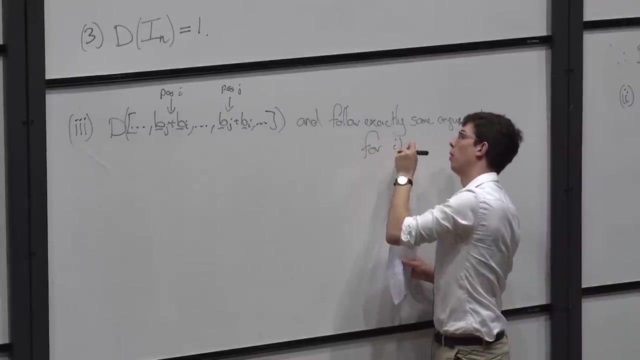 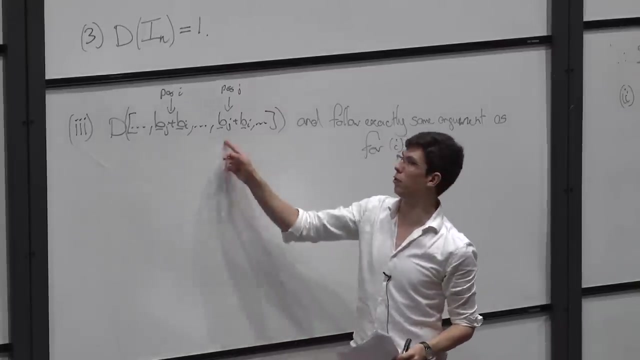 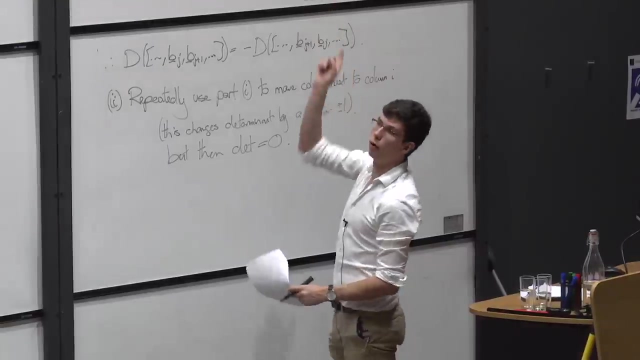 And then of course this is kind of worst-case scenario And I can follow exactly the same argument as for part i. I can expand this out as four terms: This left-hand side must vanish because two of the columns are the same, And by part ii I've seen that whenever two columns are. 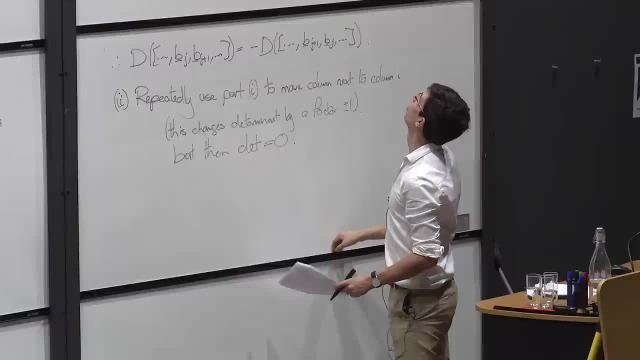 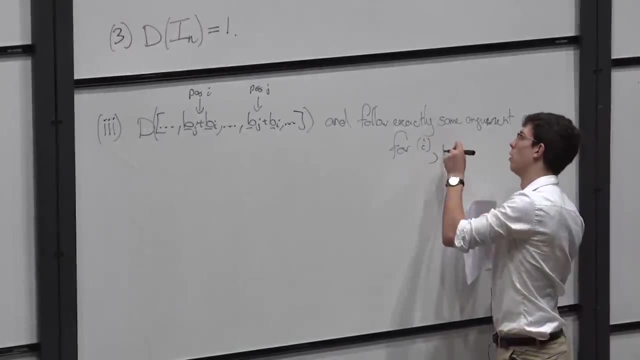 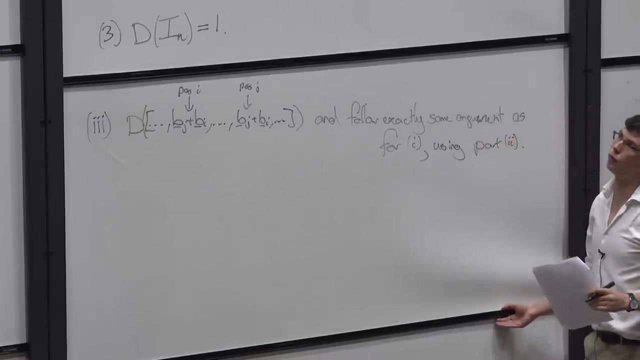 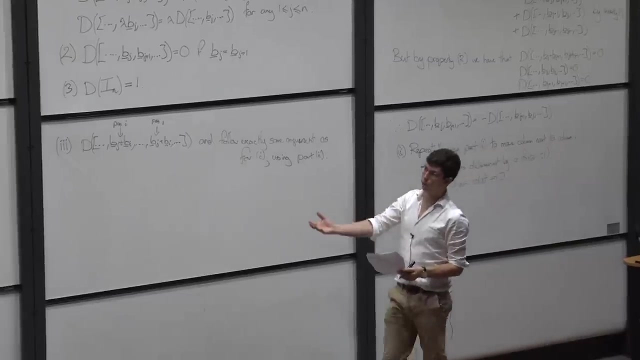 the same, the whole thing vanishes. But then, when I've expanded it out, the first term and the last term must also vanish using part ii. OK, so far what we've seen is that we've maybe had this geometric guess that there's. 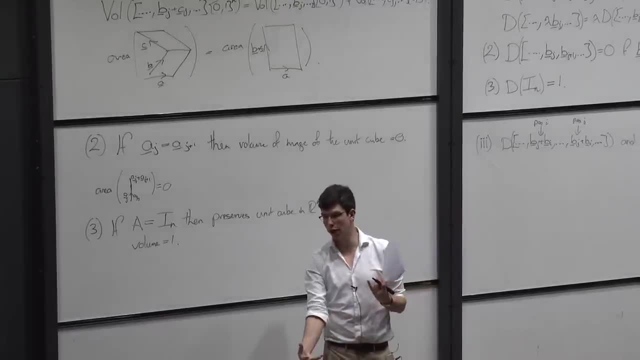 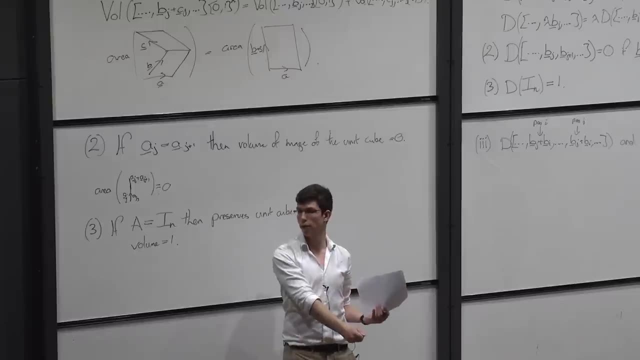 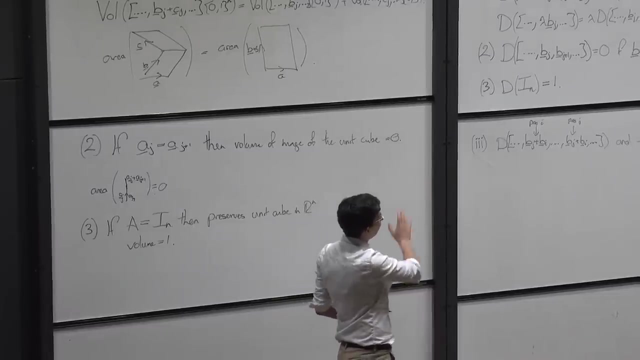 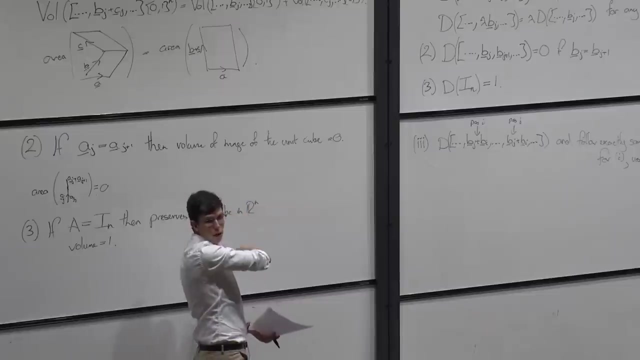 an important property of any matrix or linear transformation, which is how it scales volumes, And this is an important constant that you associate to any matrix. I've then defined this abstract property of any function being determinantal if it satisfies first of the properties that we expect this genuine constant to satisfy. 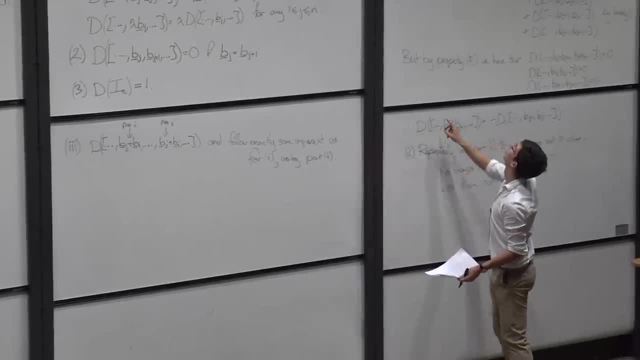 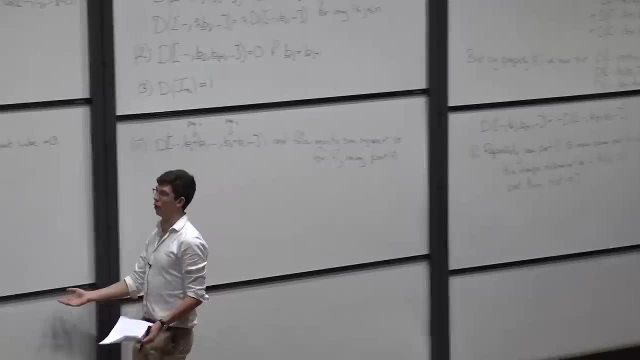 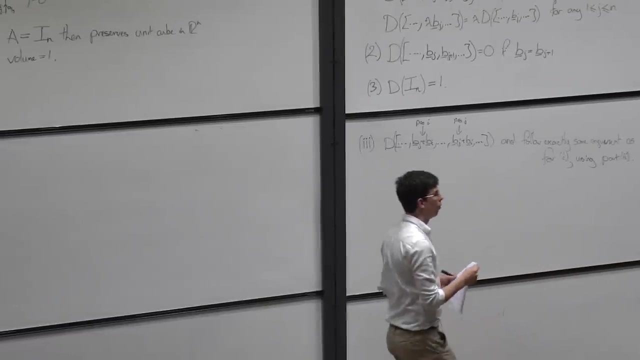 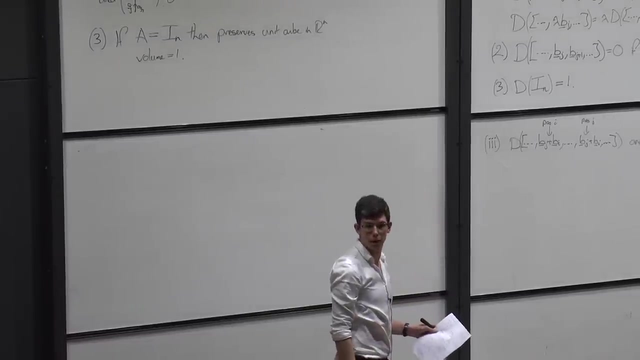 And I've seen that if it satisfies those properties then through this proposition it actually satisfies slightly stronger versions of those properties. So we've now done enough of the basic important properties of the determinant, But we haven't seen that actually there's any such map that satisfies these properties. 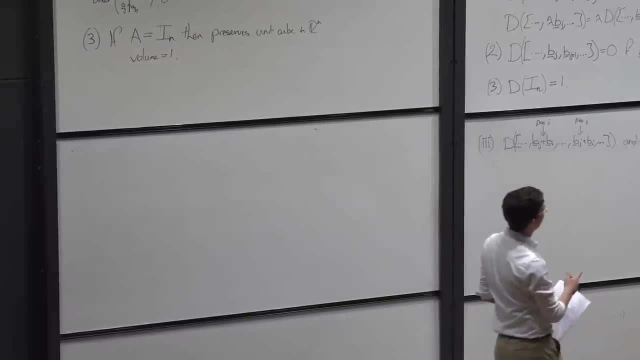 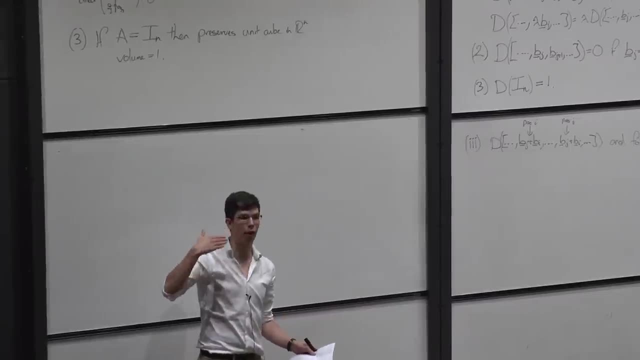 And so that's what I'd like to do now. I want to show you that there is at least some function which satisfies all these properties. In the back of my mind, I'm thinking that a function that satisfies these properties is the volume of the image of the unit cube. 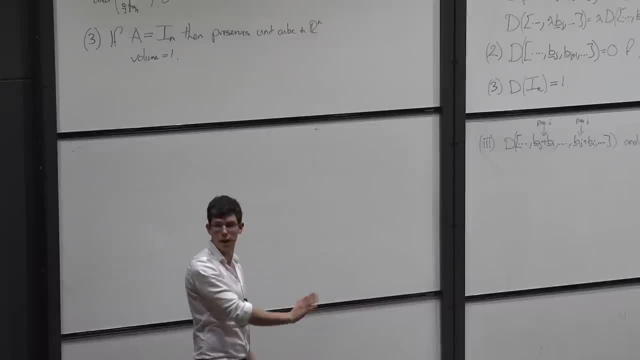 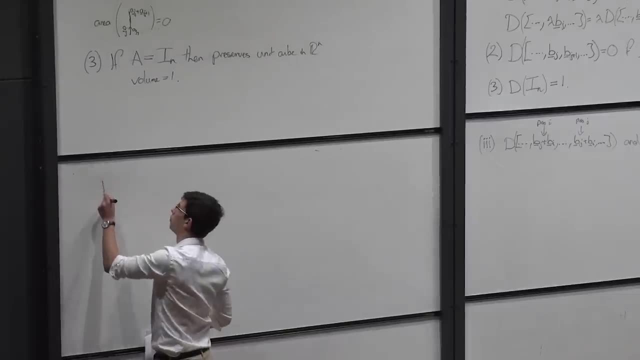 But again, I don't want to do any calculations geometrically, I want to do them all in an algebraic way, because that makes everything much, much cleaner. And so this is maybe the first important result of the course. So let's call it a theorem. 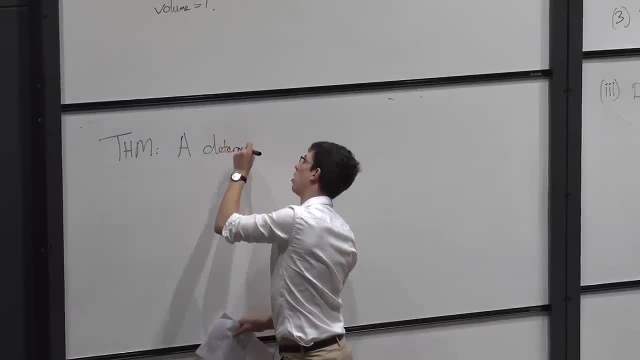 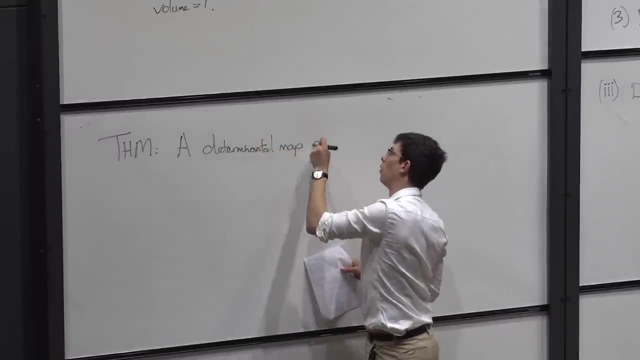 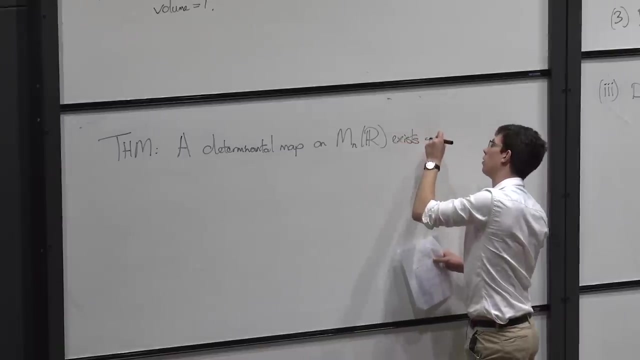 A determinantal map exists on n by n matrices. It exists for n by n matrices, And so this is maybe the first important result of the course. And secondly, I'm going to do all theupl limbs of each n bigger than equal to 1.. 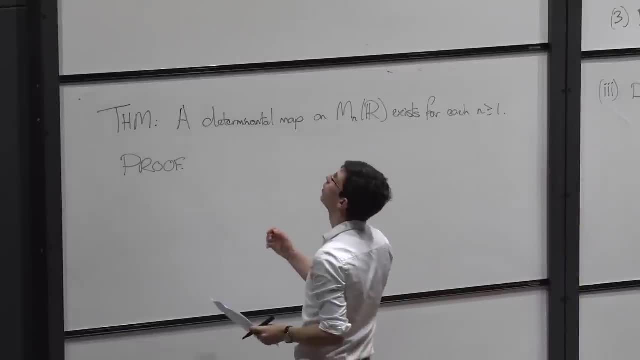 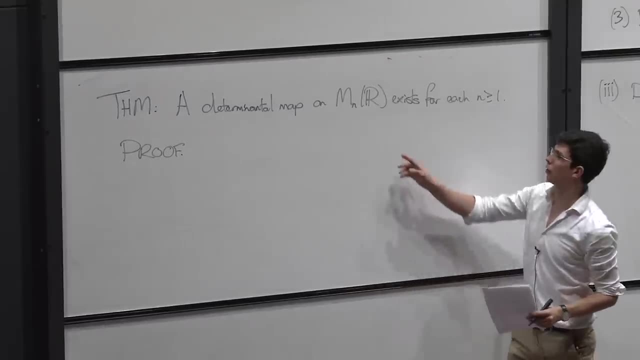 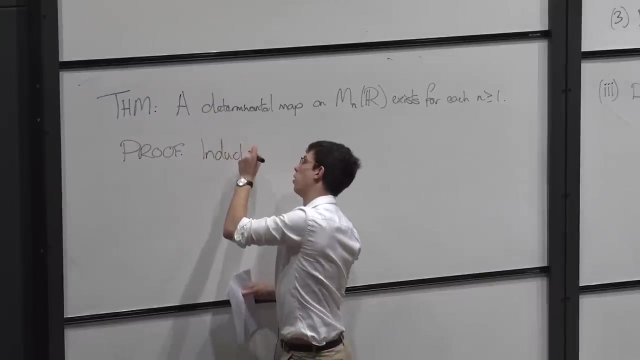 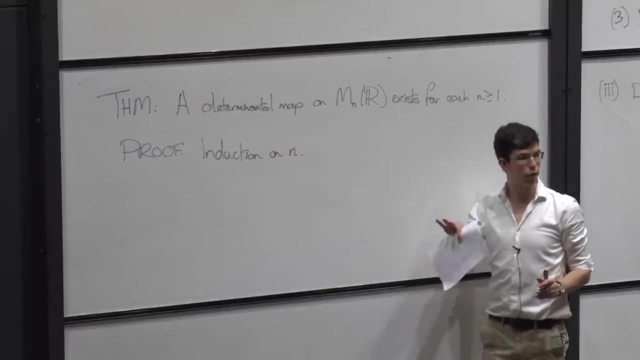 It's not totally obvious that something should exist from this, And to prove this, I wanted to a proof by induction, where I'm going to induct on the size of the matrices. OK, so let's first of all start thinking about the case. 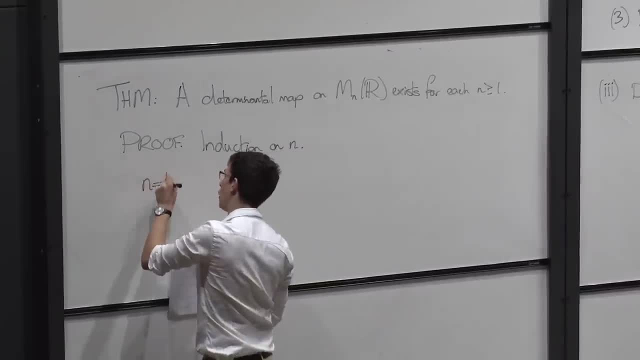 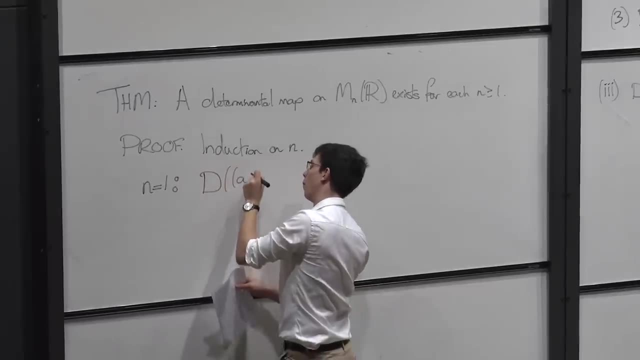 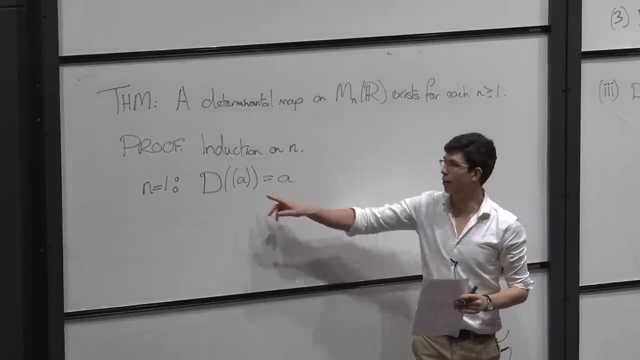 when n equals 1.. So we're just looking at 1 by 1 matrices And I can define d of just a 1 by 1 matrix A to be maybe the most obvious thing, just its entry A And since the identity function is certainly linear, 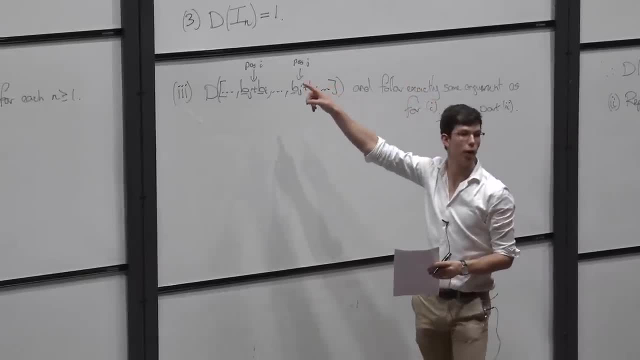 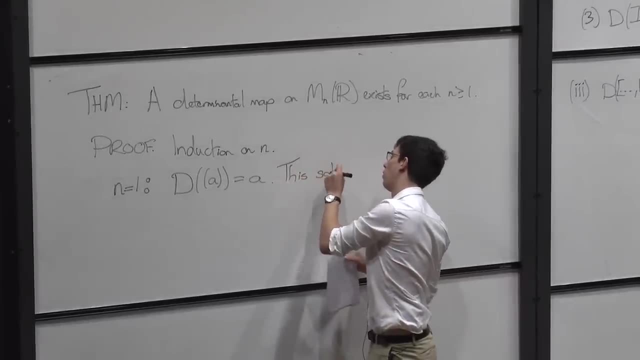 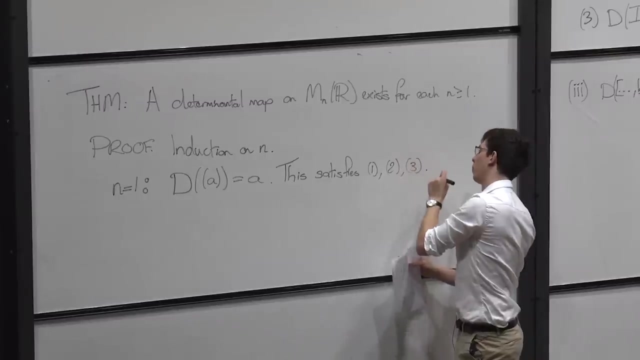 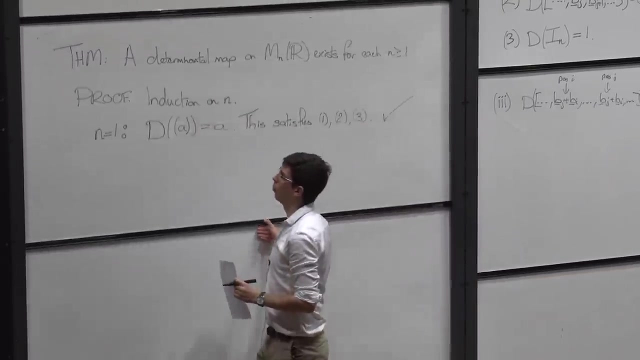 it's very easy to check that d satisfies the properties 1,, 2, and 3 here. OK, so we've shown that something exists for 1 by 1 matrices, And now we want to. We want to consider the case when n is bigger than 1.. 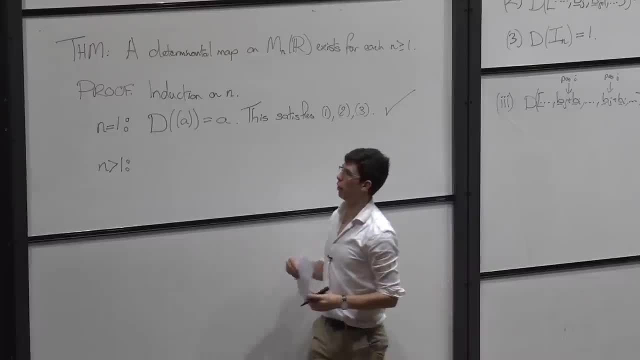 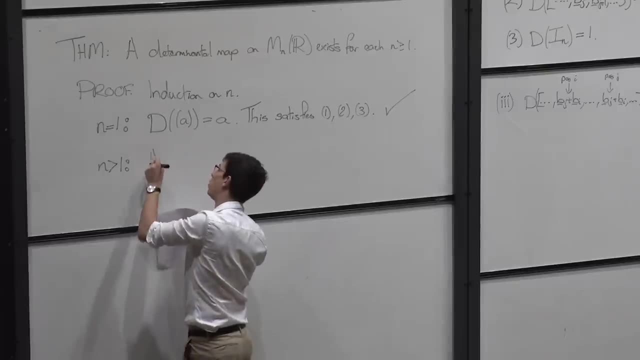 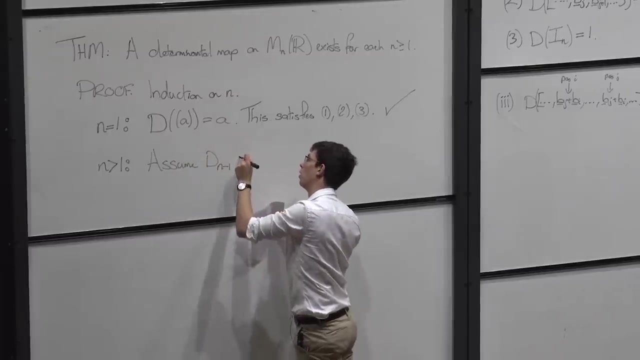 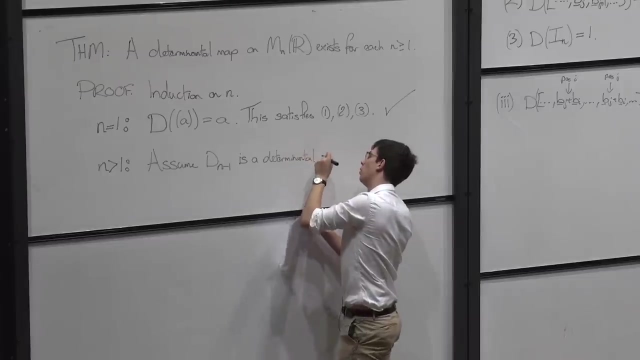 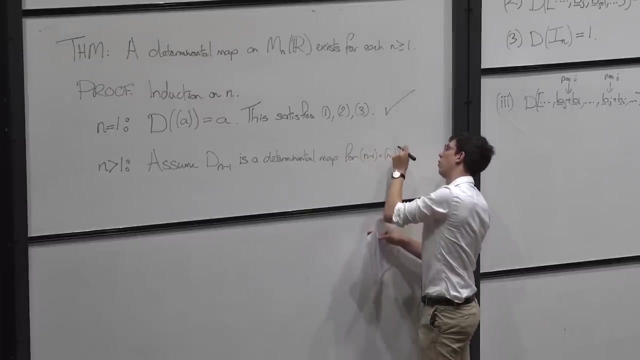 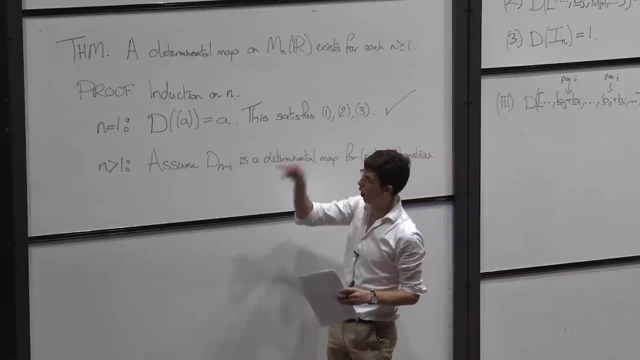 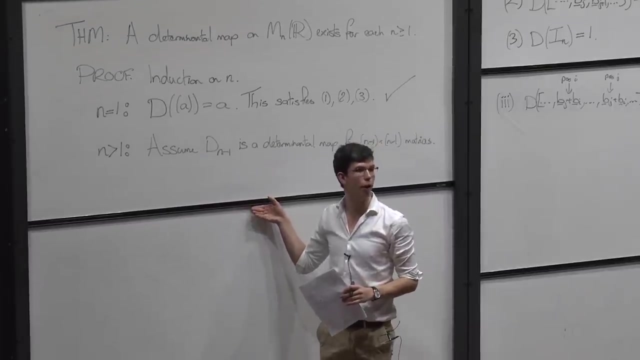 And we're going to assume that something exists. some determinative map exists for n minus 1, by n minus 1 matrices. So we somehow want to construct a function on n by n matrices out of this function that we're assuming to exist on n minus 1, by n minus 1 matrices. 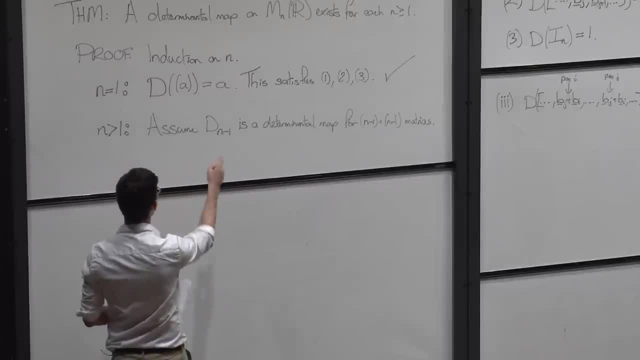 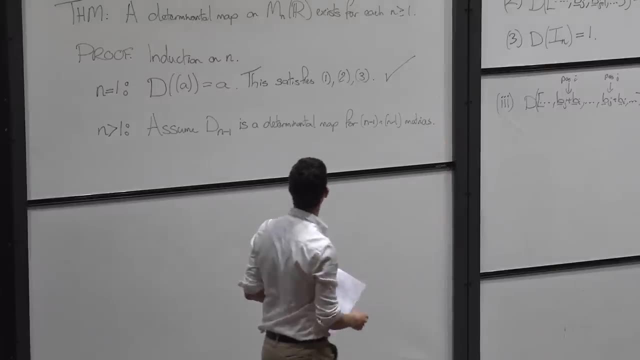 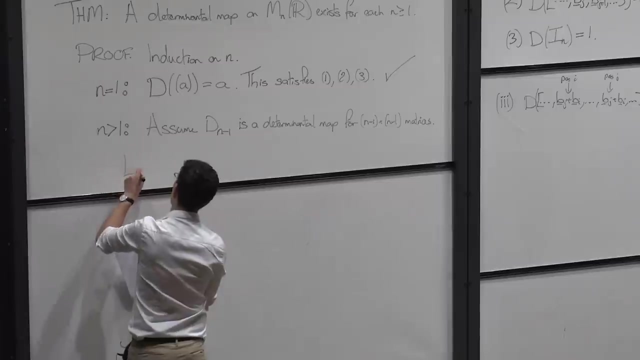 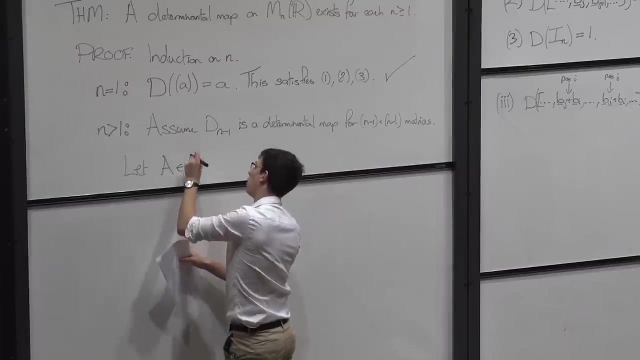 So I want to come up with some. I want to cook up some way of coming up with a determinative map that satisfies those three properties. But I want to somehow use this n minus 1 by n minus 1 map. So I want to think of some matrix A, which 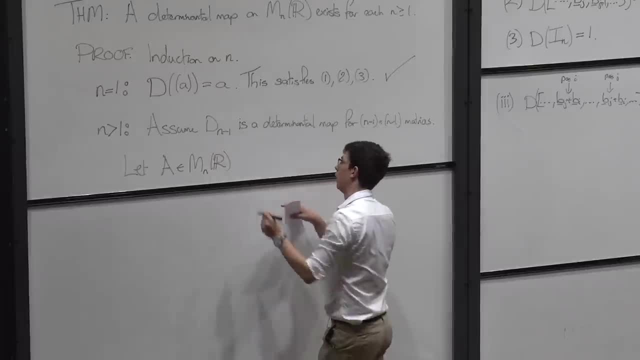 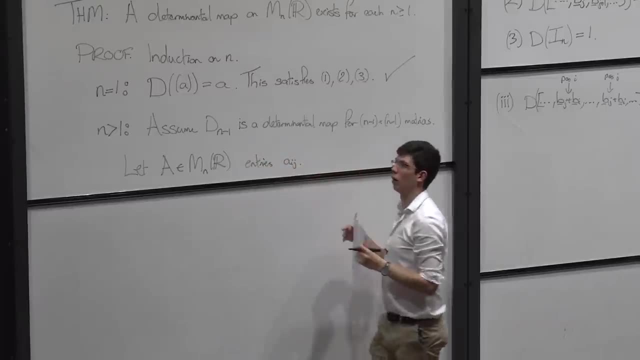 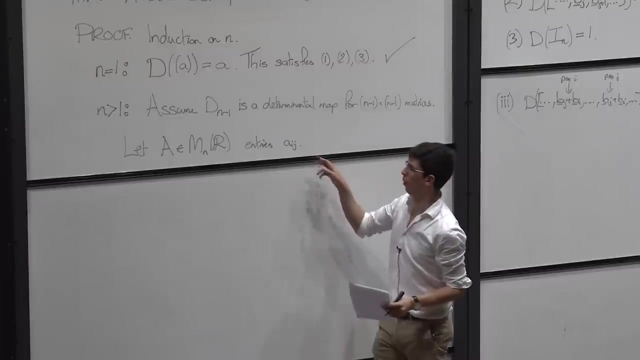 is an n by n matrix. So let's say it has entries little a And if I'm going to use this dn minus 1, which is clearly going to be important in the argument- I have to think about how can I construct a n minus 1. 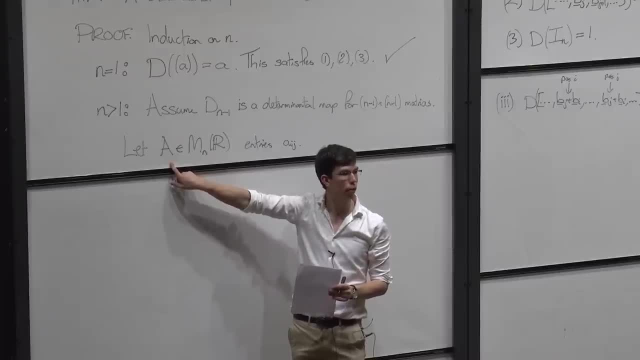 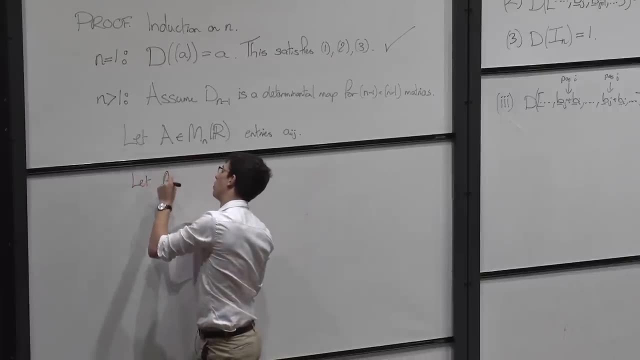 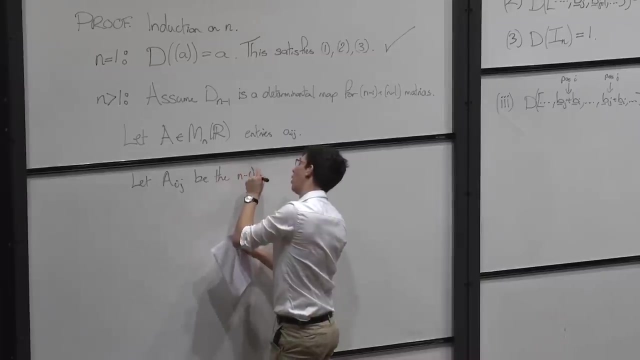 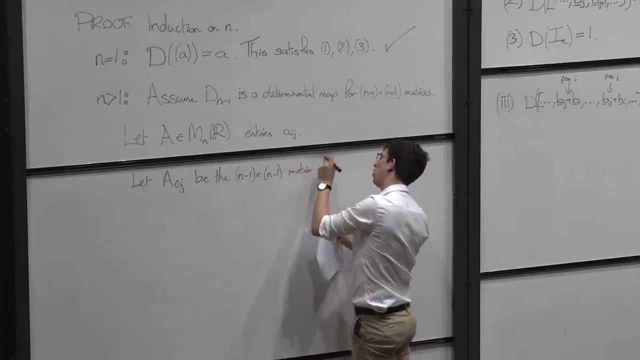 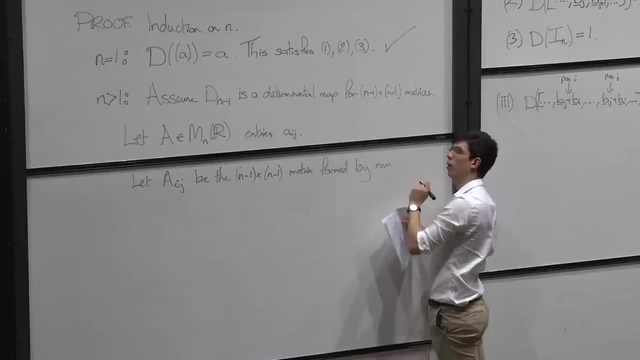 by n minus 1 matrix out of this n by n matrix. Maybe there's one easy way to do this, which is just to throw out some row and some column. So I want a ij capital, A ij to be the n minus 1 by n minus 1. 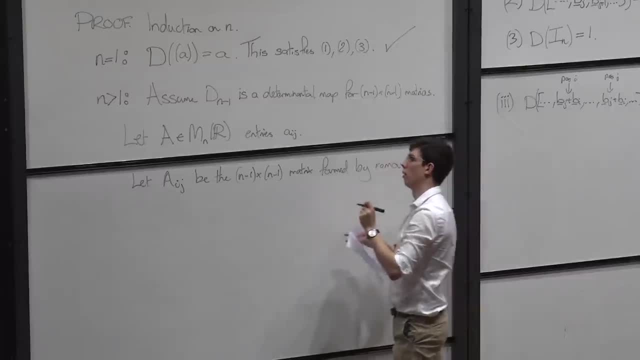 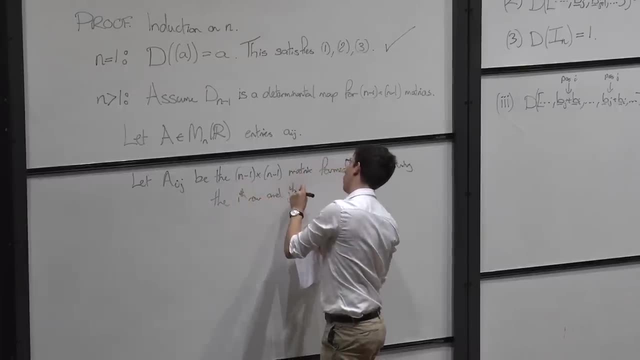 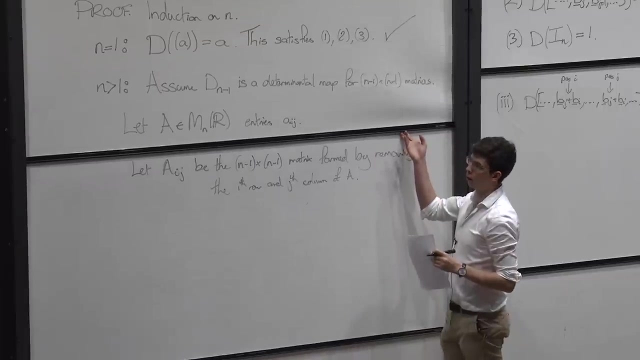 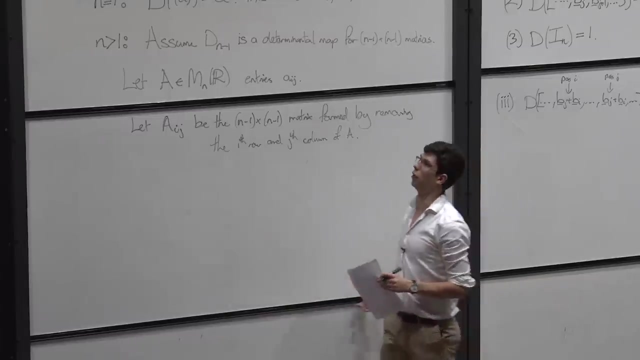 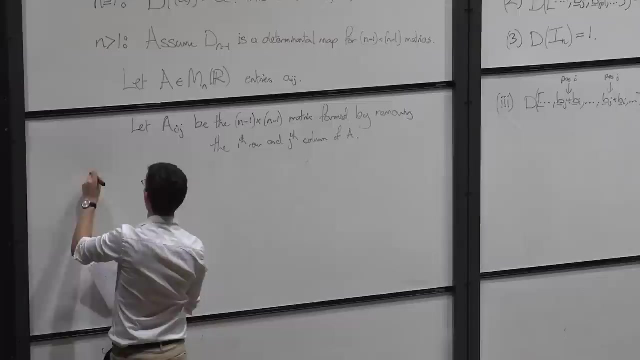 matrix formed by removing the i through o and j-th column. OK, So this is one way of constructing various different n minus 1 by n minus 1 matrices from my n by n, matrix A And I'm now going to consider. so let's choose some i. 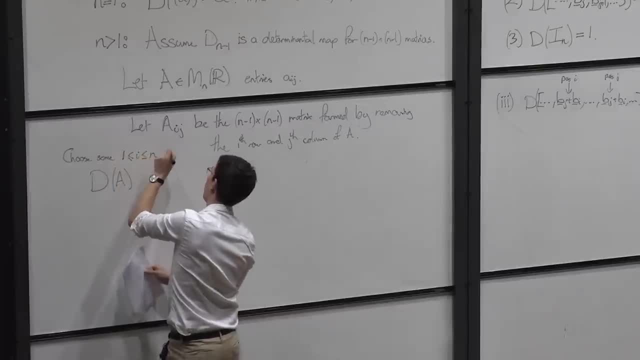 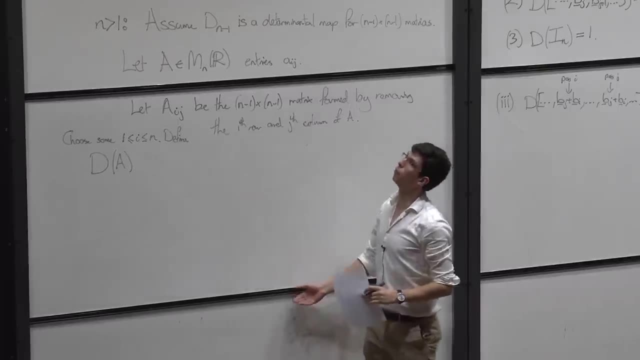 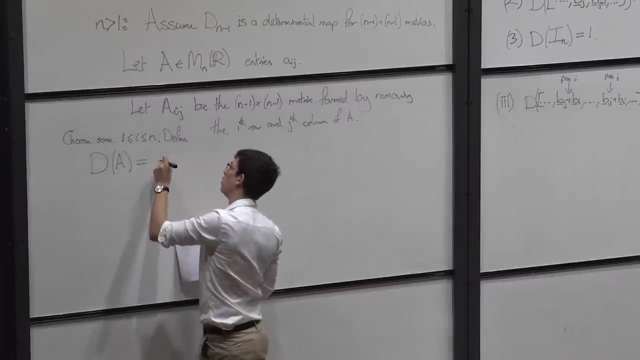 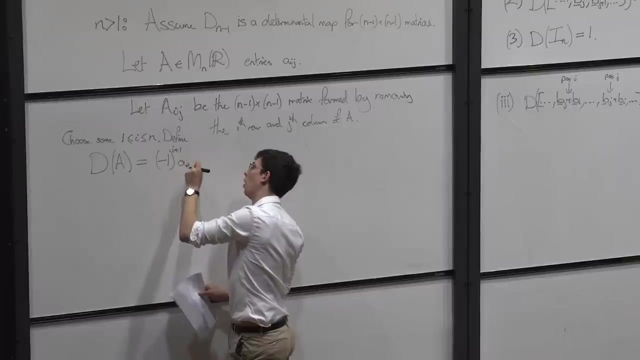 between, And I'm going to define 1 and n, And I'm going to define my attempt to a determinant function on n by n matrices as follows. So I will put minus 1 to the i, plus 1, a i 1.. 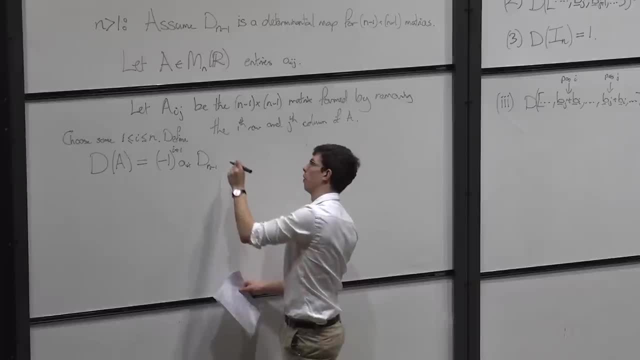 And then I'm going to use the n minus 1 by n minus 1 function And I'm going to put minus 1 to the i plus 1 matrix A i 1.. And then I'm going to put minus 1 to the i plus 1 matrix A i 1.. 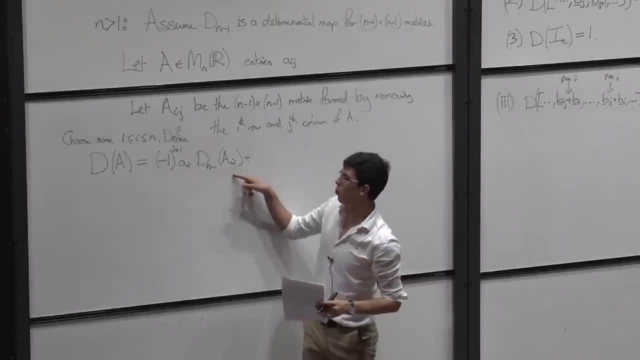 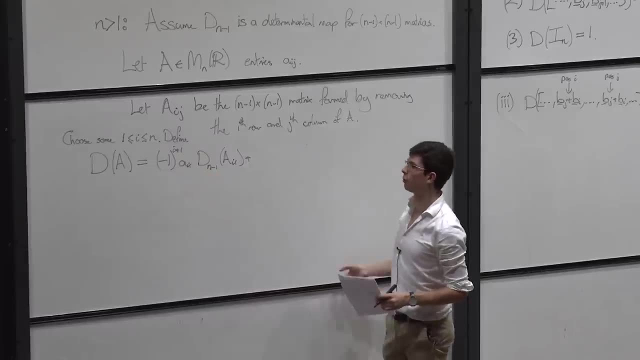 But maybe so. this is some function that would work on n by n matrices but is ignoring lots of the elements in the i throw. So instead I want to add lots of these similar versions of this together to get something that's sensitive to every single element in the matrix. 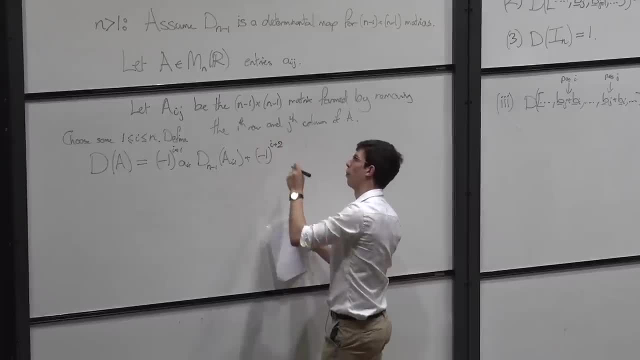 And it turns out that a good way to do this is to keep it in. And it turns out that a good way to do this is to keep it in. So I'm going to keep on multiplying by minus 1 and just going through all the different possible choices. 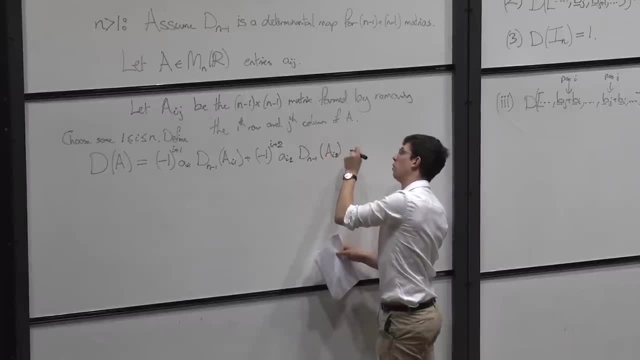 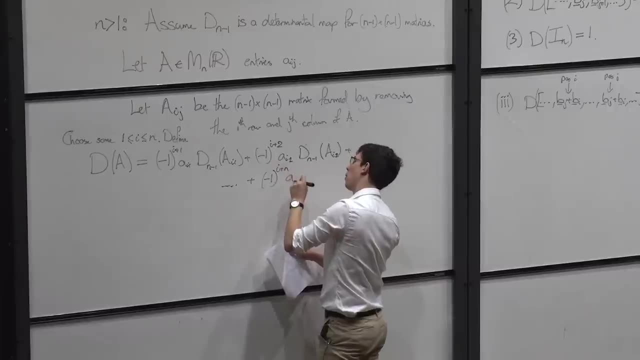 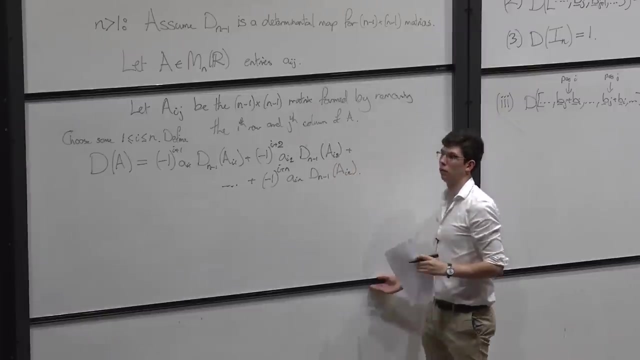 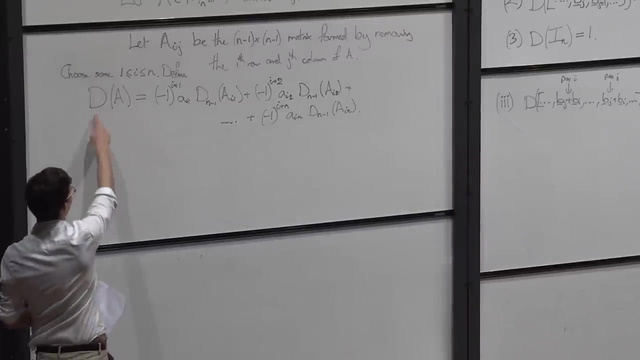 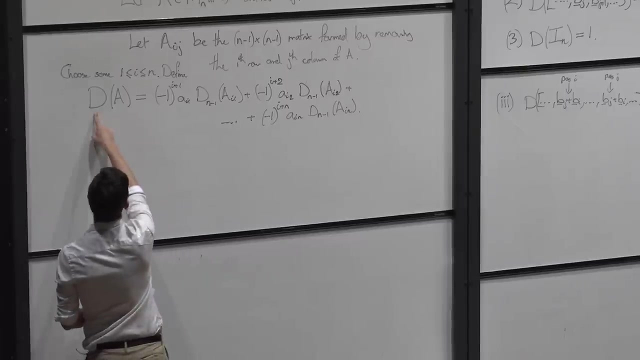 in the i throw OK. So I've just plucked from thin air this matrix here. But I think if you play around with it a little bit and you decide that you want to come up with some way of defining a function on n by n matrices. 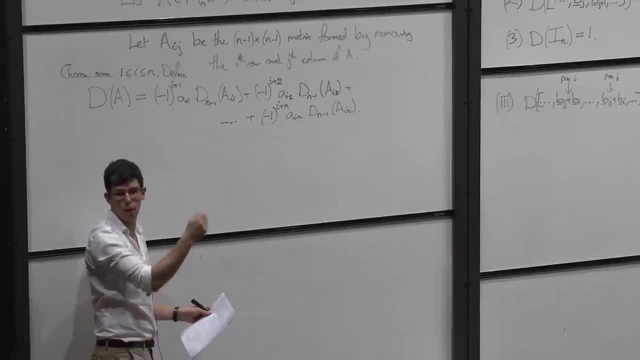 in terms of a function by n minus 1 on n minus 1 matrices. that depends on each element. you'll see that actually this isn't such an unnatural thing that I've just picked out of the air. Maybe you wouldn't have guessed these minus 1 factors. 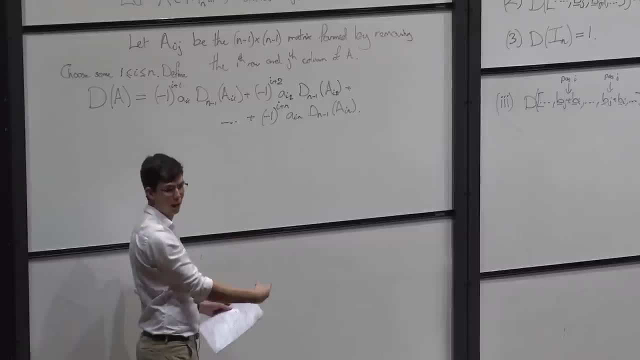 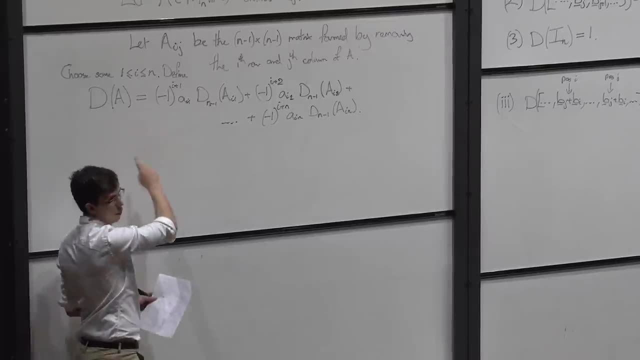 but it should be clear once we go through a bit more of the proof why these minus 1 factors turn off. Anyway, I've defined this function And this is a function on n by n matrices, And I want to show you that it's now. 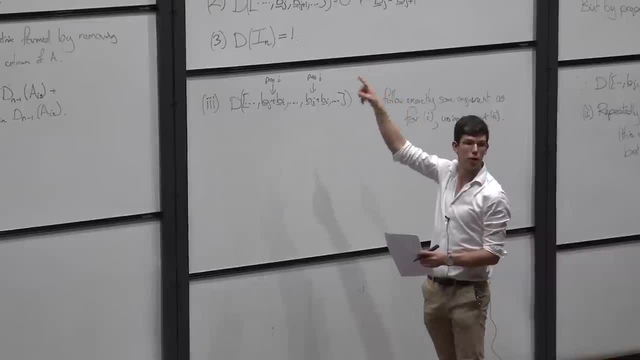 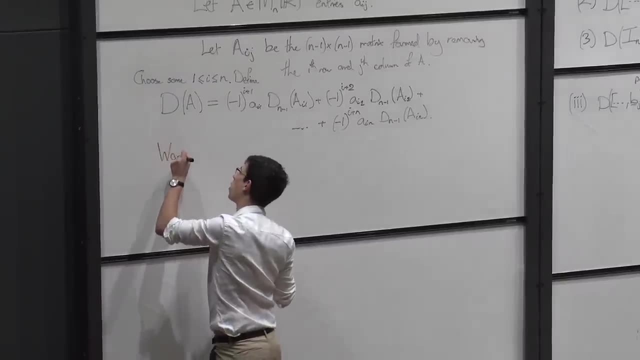 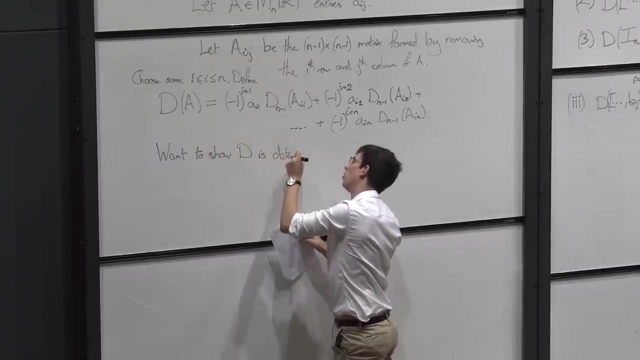 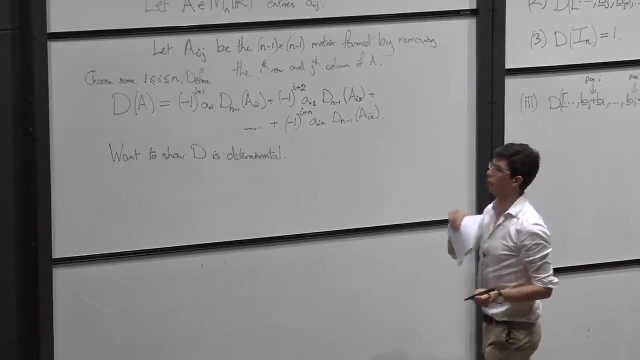 detrimental. so I want to verify that it satisfies properties 1,, 2, and 3.. And if I've done this, I have completed the proof. OK, So I'm just going to verify the properties in order. Maybe I'll move on to the middle board. 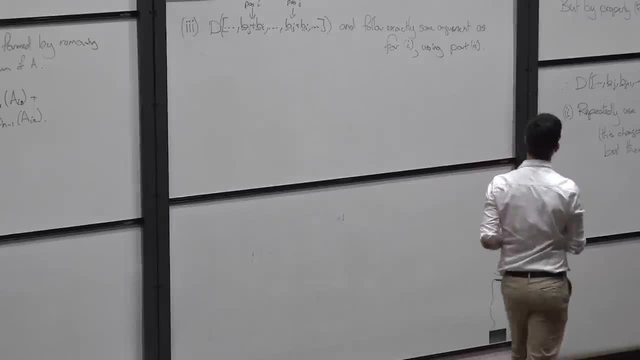 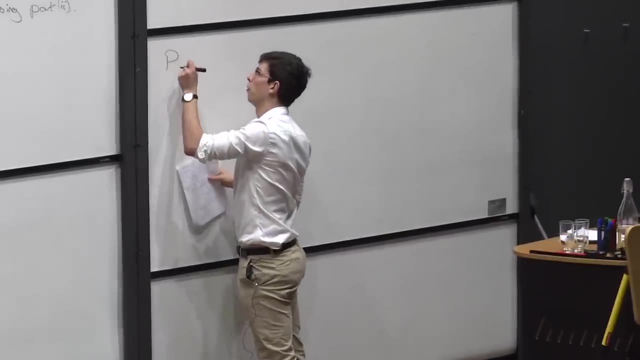 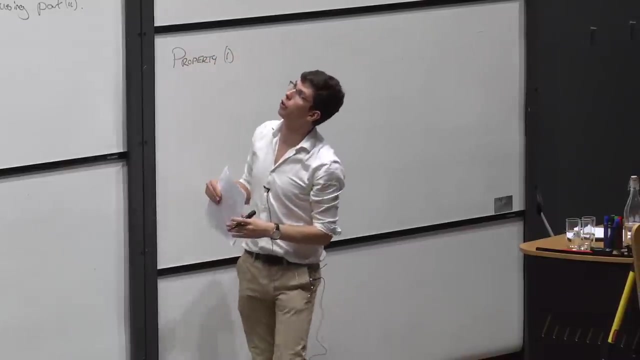 I guess maybe it would be useful to keep this board up so that we can see what the properties are. So maybe I'll move over to the right side. So let's start off with property 1.. So we'd like to show you that d is linear in each column. 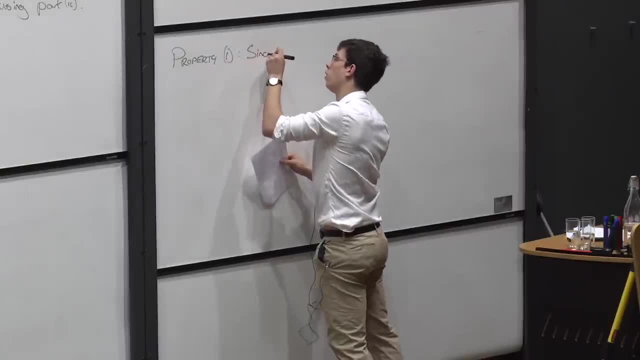 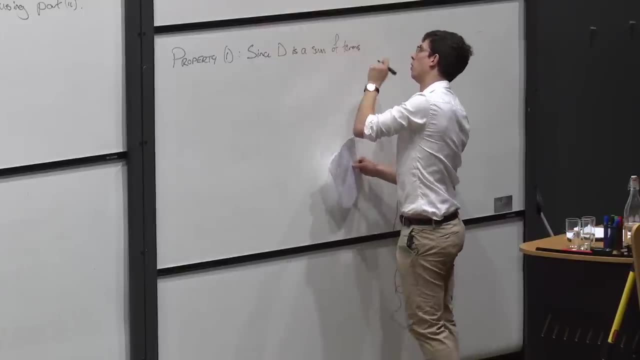 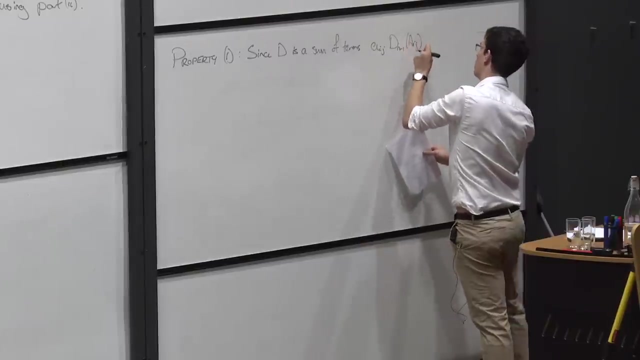 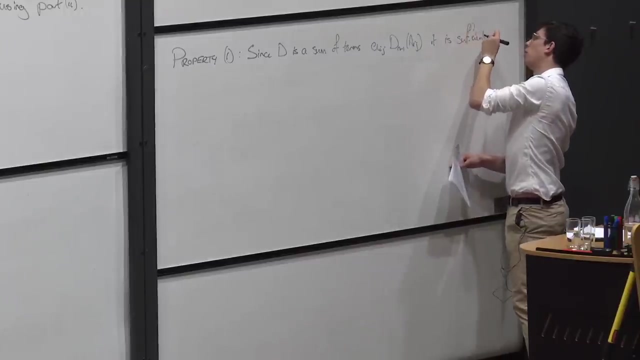 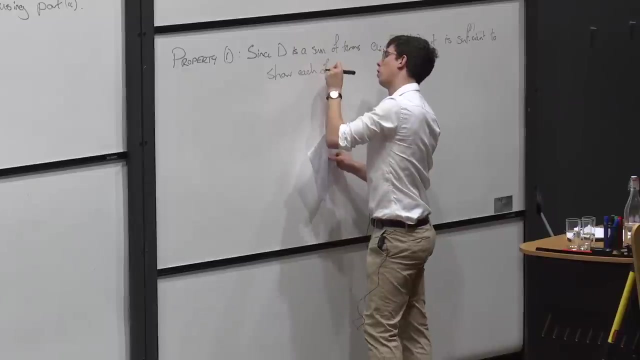 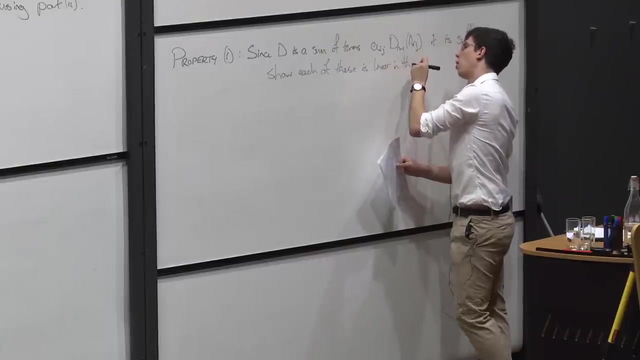 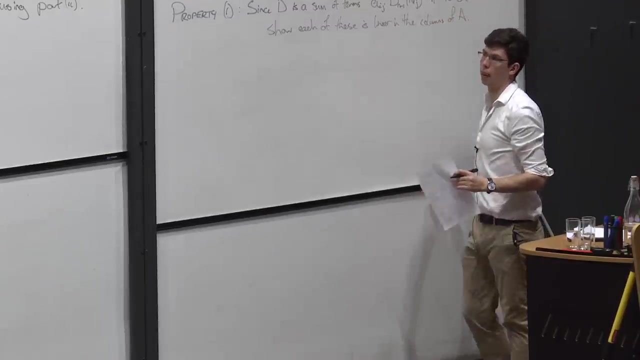 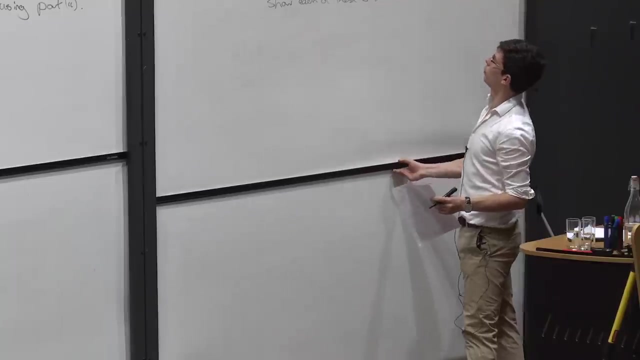 So since d is a sum of terms- aij, d, n minus 1, aij- it is sufficient To show each of these is linear in the columns. So I just need to show you that, each of these different quantities. Let's see. 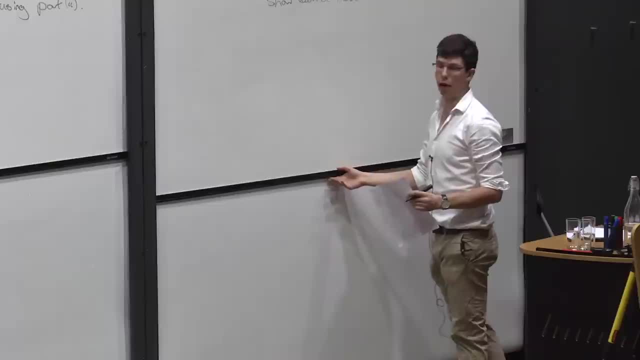 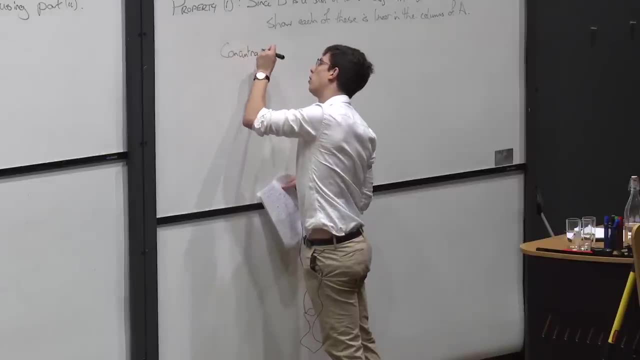 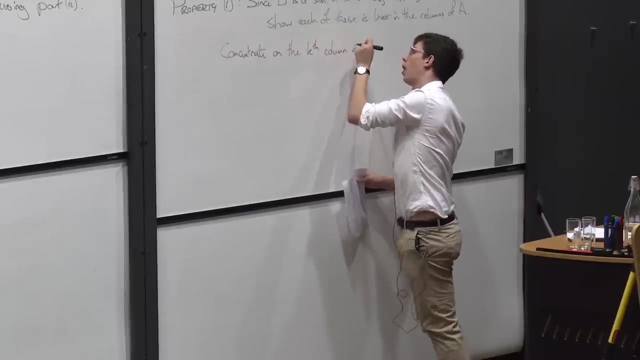 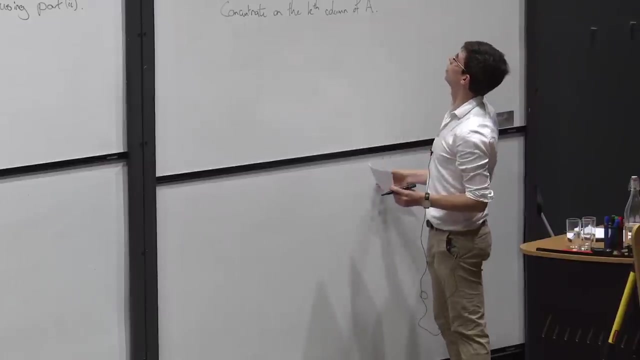 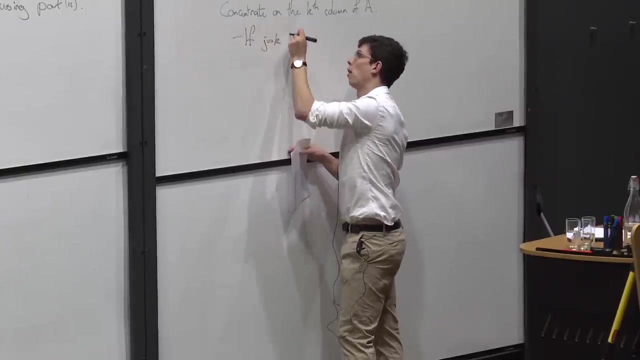 All right, is aij dn minus 1 of capital. aij is linear in the columns, And so let's concentrate on the kth column of my n by n matrix A, And I'm going to consider these functions. So if j is equal to k, then aij doesn't. 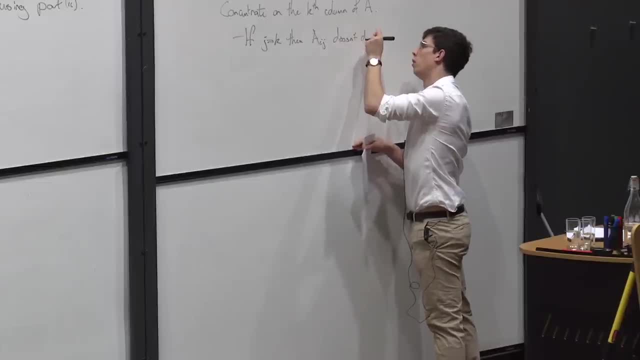 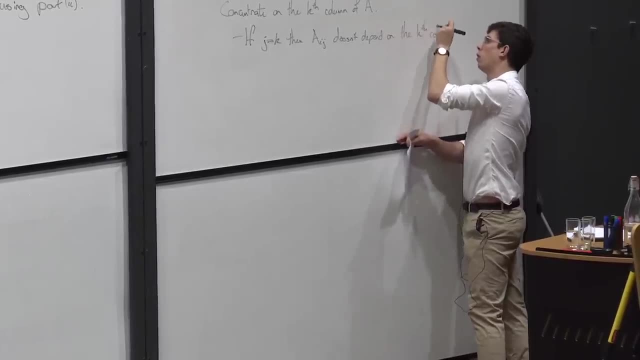 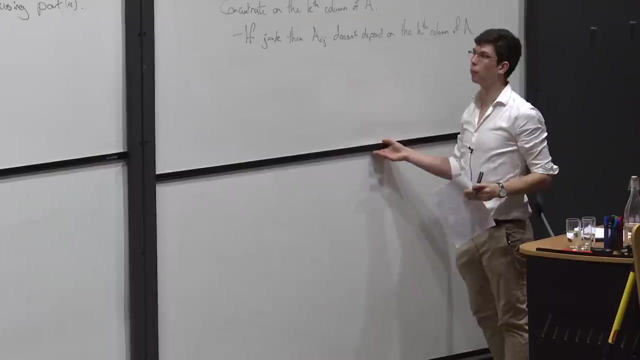 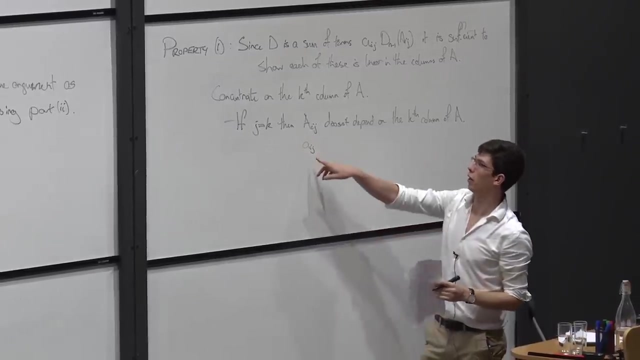 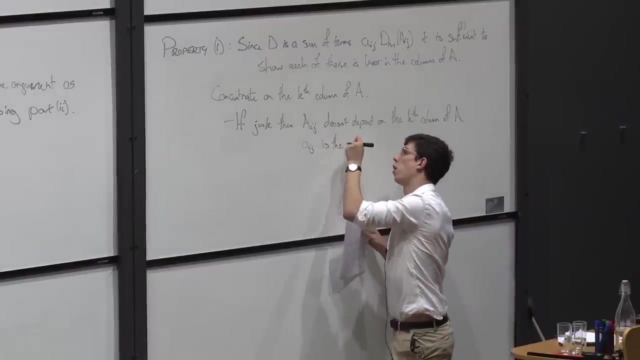 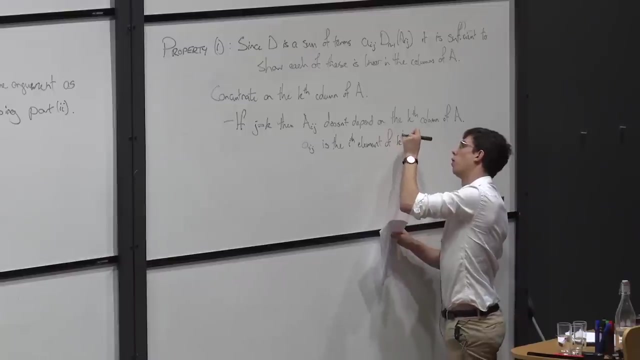 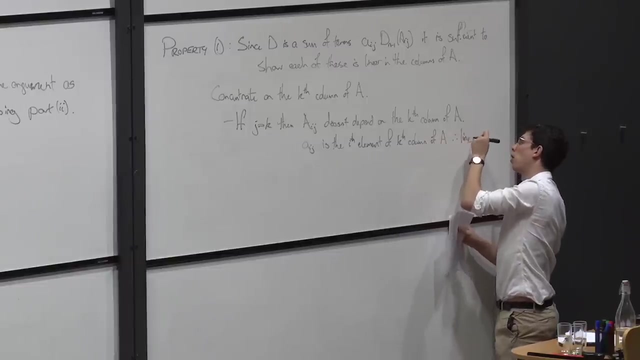 depend on the kth column of A, because this is formed by removing the kth column of A, But little aij is just the ith element of the kth column, and so it's certainly linear. And so by putting these two things together, 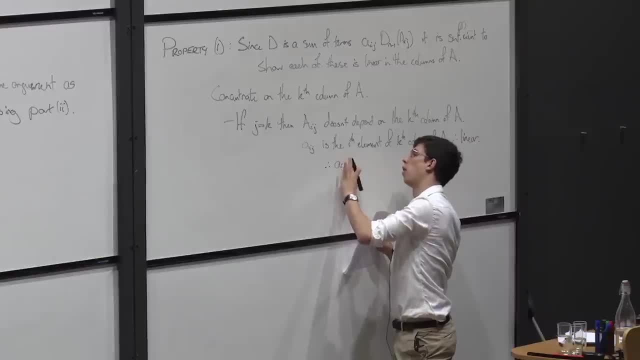 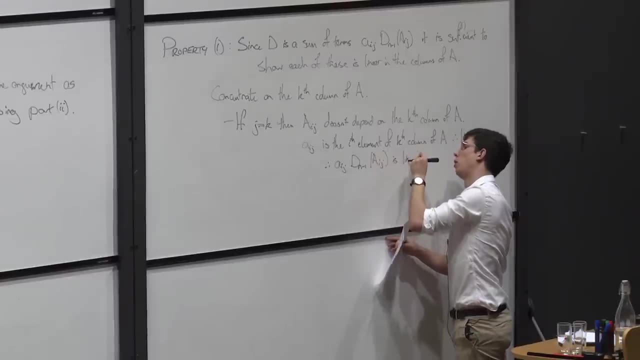 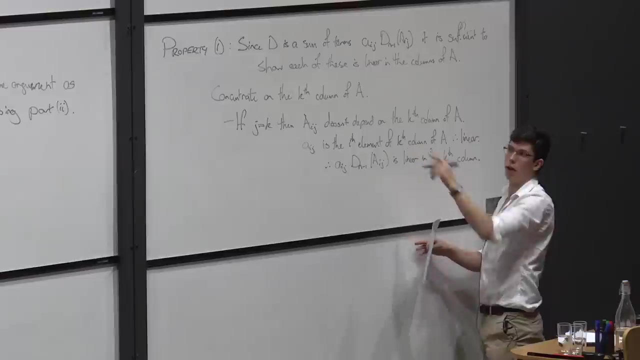 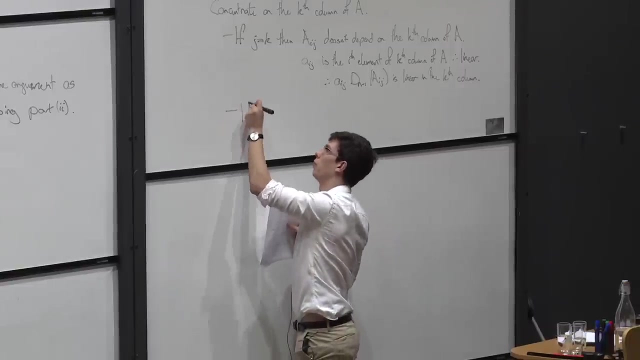 we see that aij, dn minus 1 of aij is linear in the kth column when j is equal to k. What if j is not equal to k? Well then, we can do this, We can do this, We can do this. 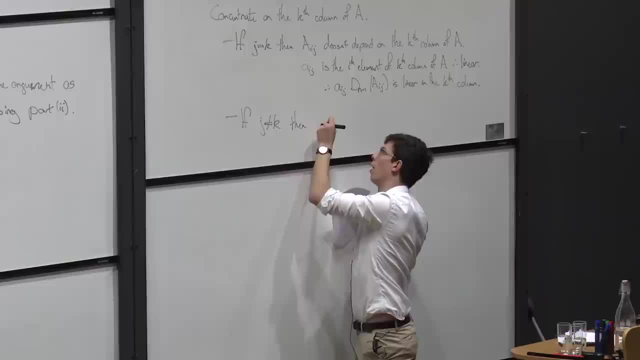 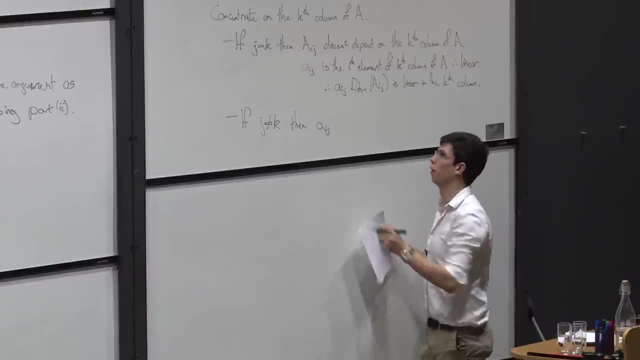 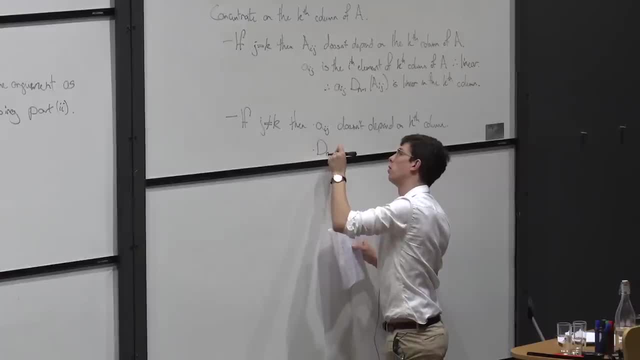 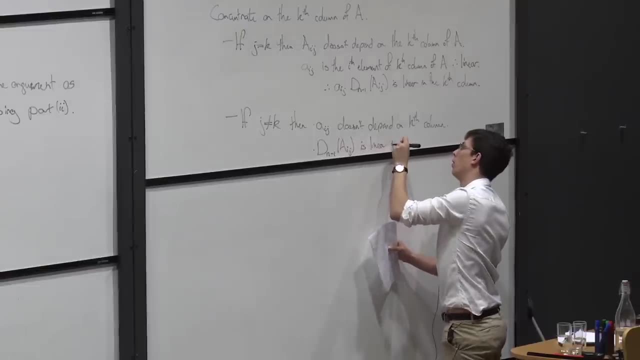 But we have that dn minus 1 of aij is linear in the kth column. But we have that dn minus 1 of aij is linear in the kth column. And so aij, dn minus 1, aij is linear in the kth column of a. 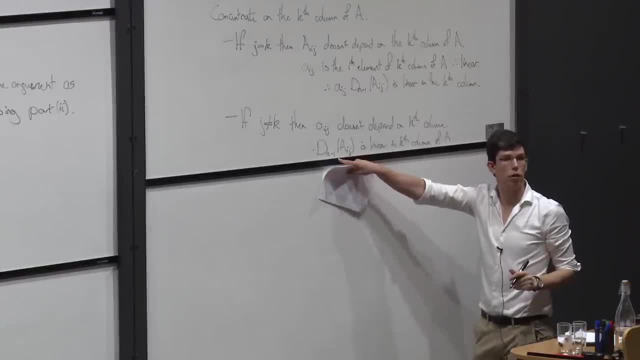 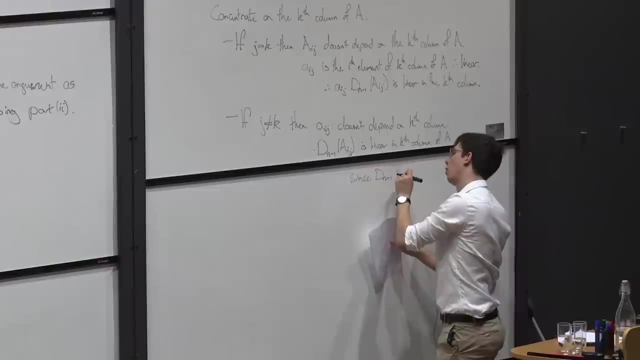 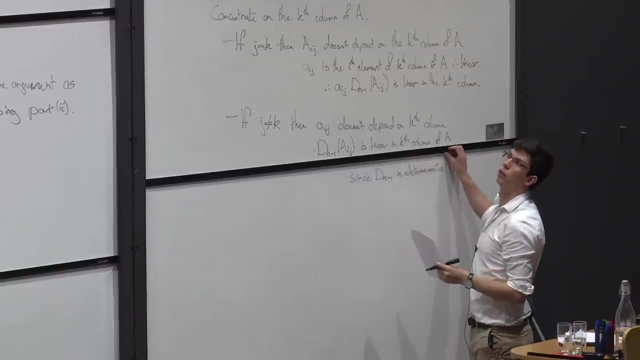 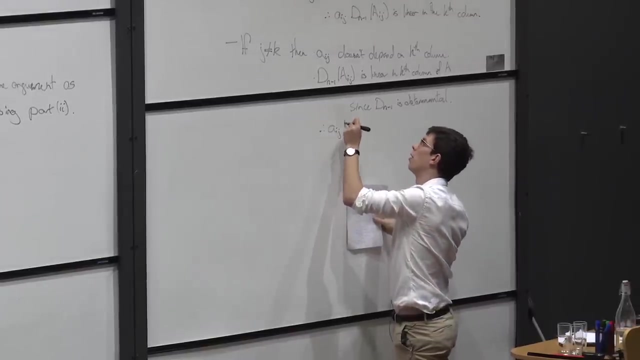 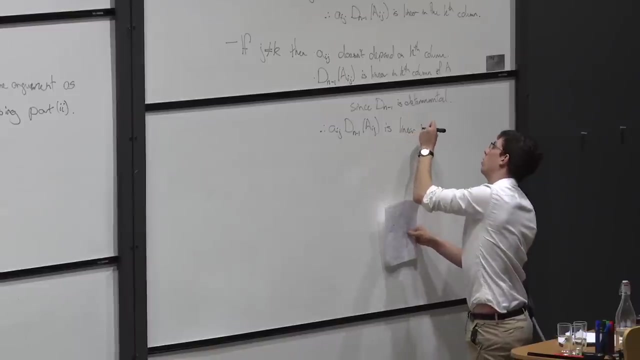 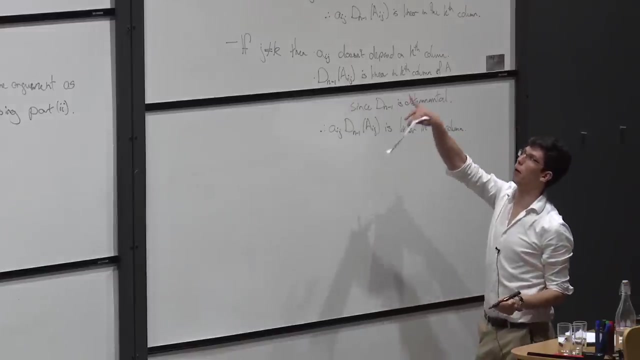 since we're assuming that this function is detrimental and so it's linear in the columns and therefore in this case we have the AIJ. dn minus 1 of AIJ is linear in the kth column and therefore, regardless of what value of j is, these functions are always linear in the kth column. 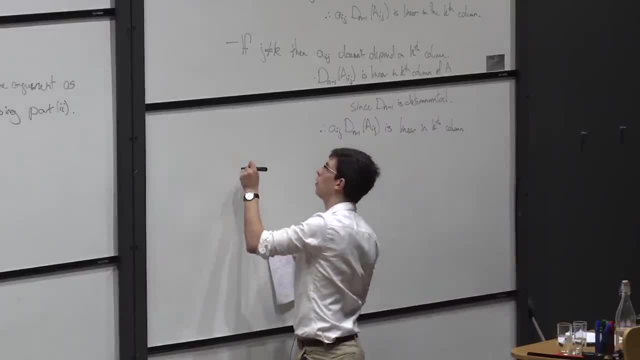 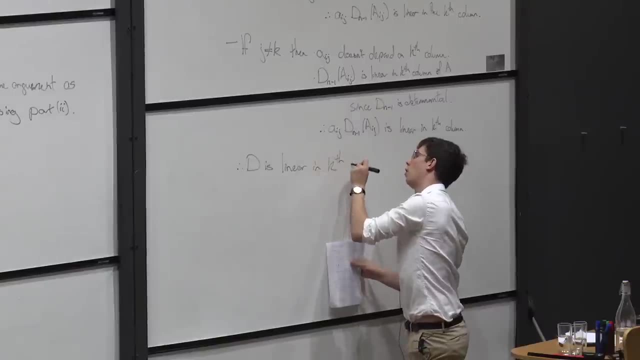 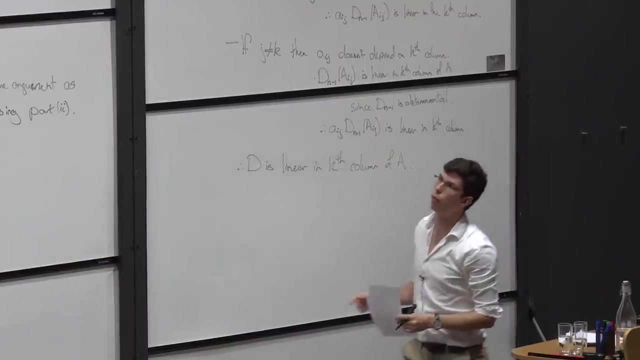 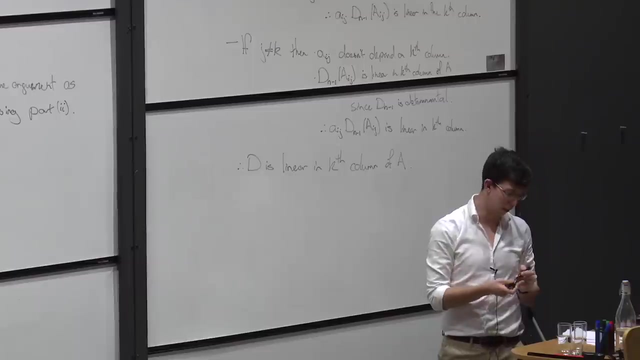 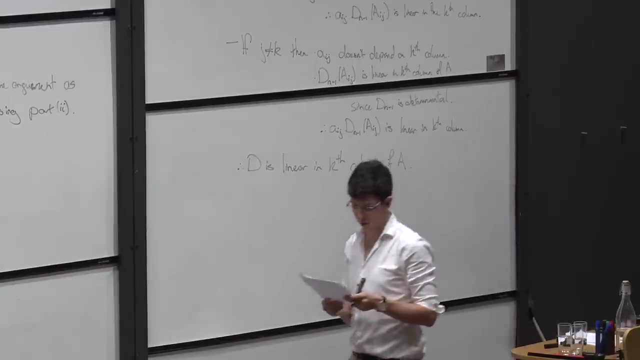 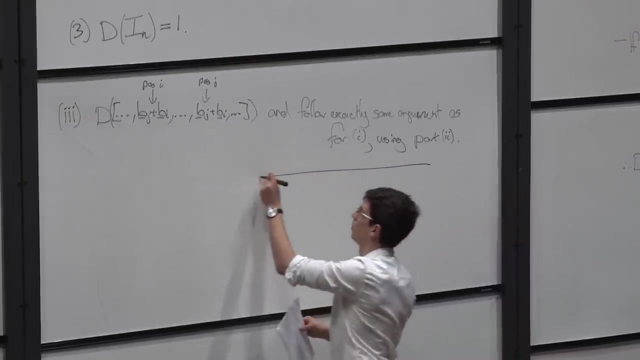 and so d is linear in the kth column. okay, so we've therefore verified property one for this function d that I've received, so we're left to verify properties two and three. so maybe we have just enough space here, so let's go for property two. 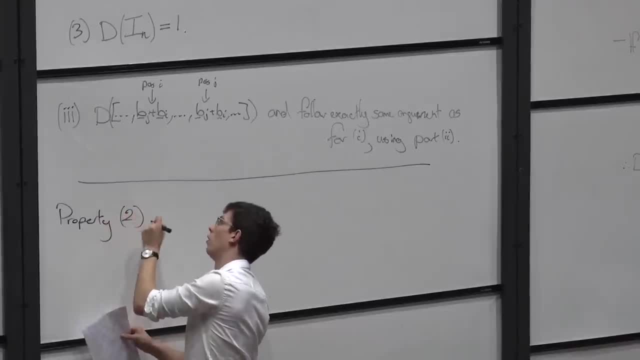 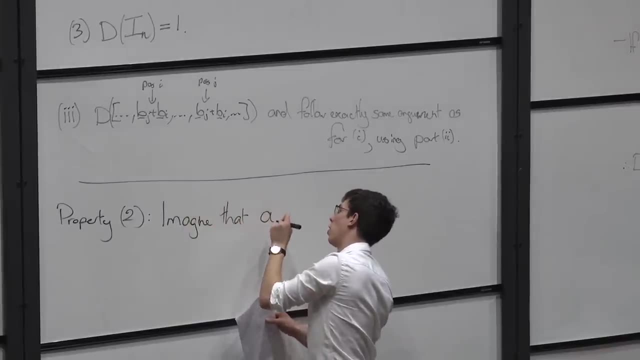 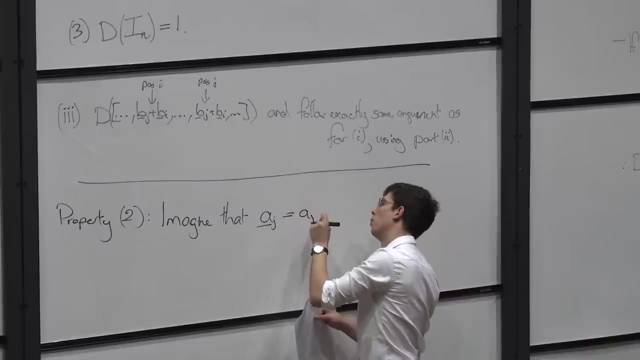 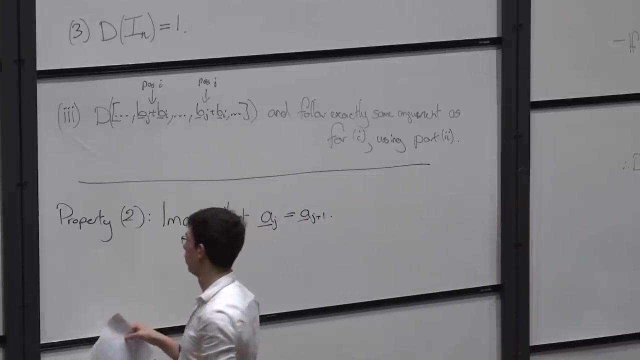 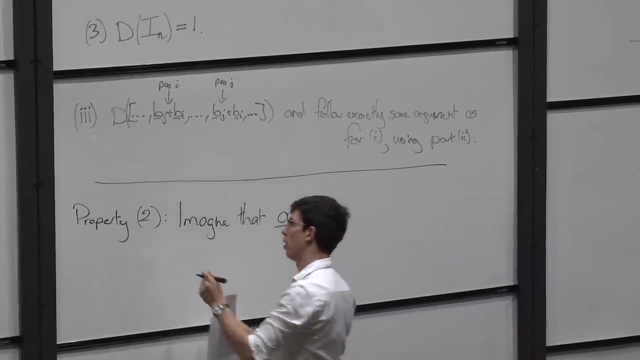 imagine that in my matrix a, I have a, the jth column is equal to the j plus first column, and so I want to show you that this determinant has to be zero then. so again, it's going to look a little bit similar to this: um, a, i, j. 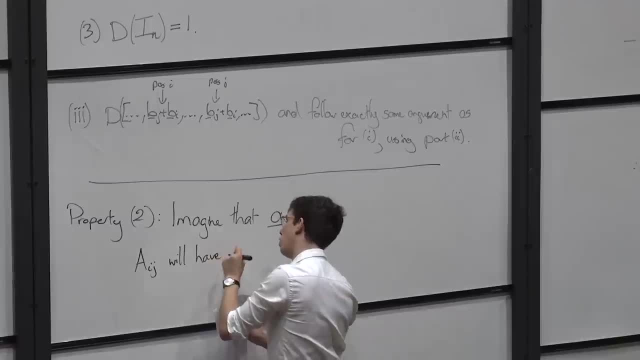 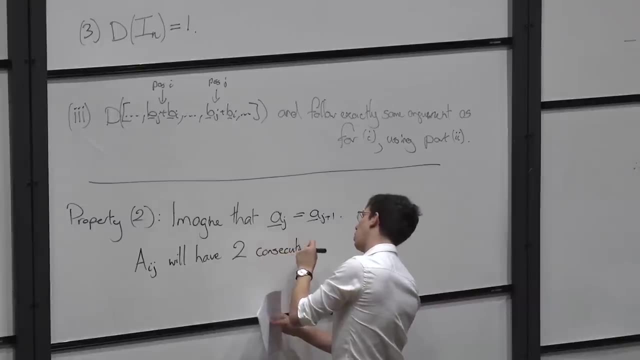 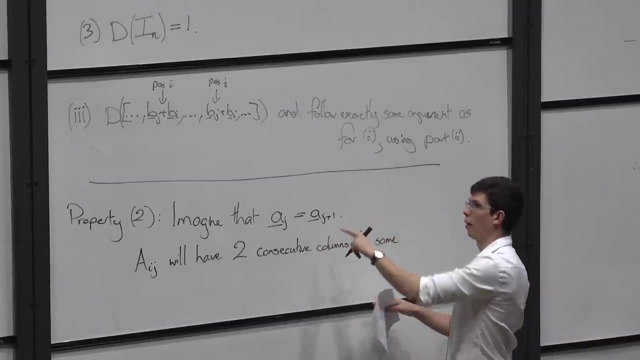 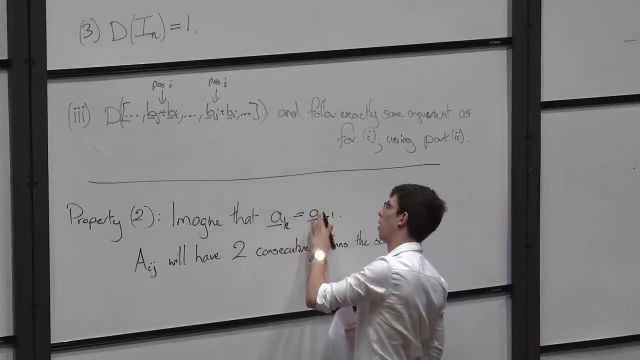 we'll have two columns the same, two consecutive columns the same, because it essentially has the columns inherited from aj and aj plus one, unless we removed one of these two. um okay, sorry, my notation's slightly bad. let's imagine that ak is equal to ak plus one, just because otherwise I'll get confused by all the indices. 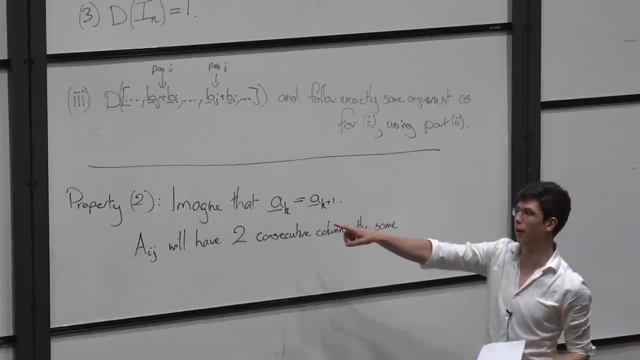 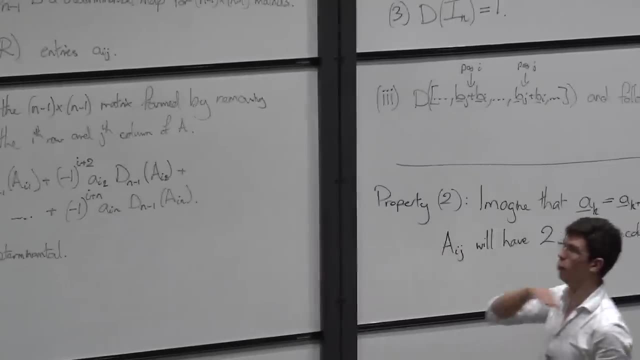 apologies. so imagine that the kth column is equal to the k plus first column. and now I'm looking at one of these matrices aij, where I'm removing the, i throw in the jth column. if I haven't removed either the kth column or the k plus first column. 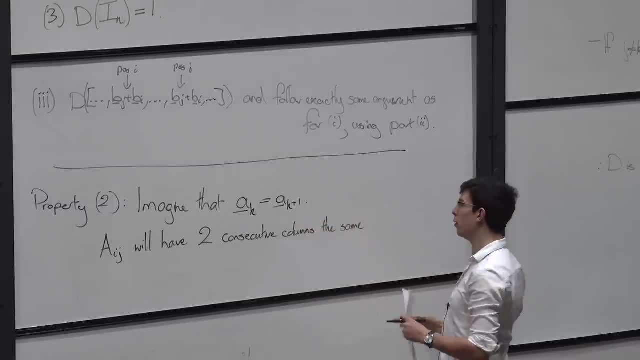 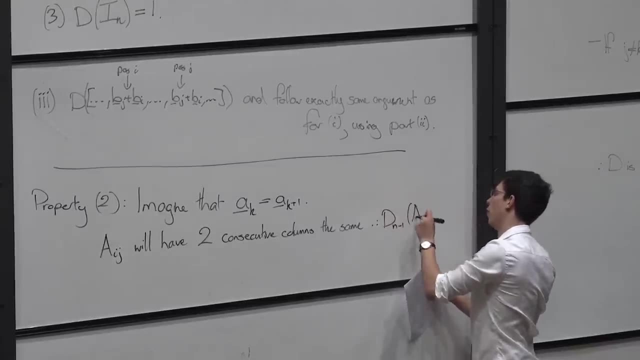 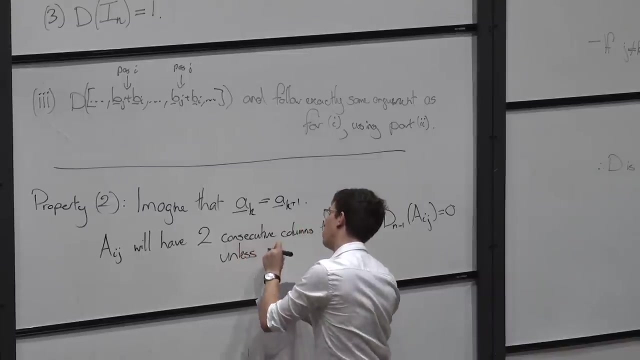 then whatever corresponds to these two will still be the same, and so we'll have two consecutive columns the same, and therefore our we'll have the dn minus one of aij is equal to zero, but this is only true if I haven't removed one of those two columns. 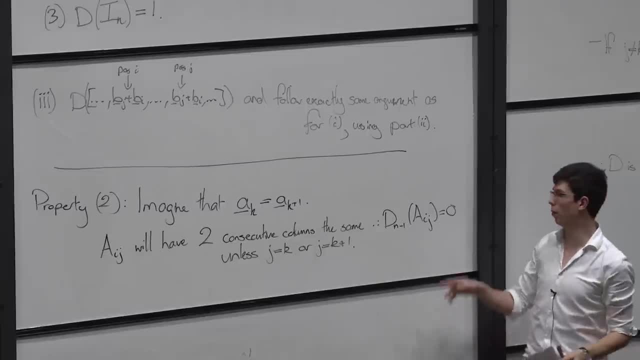 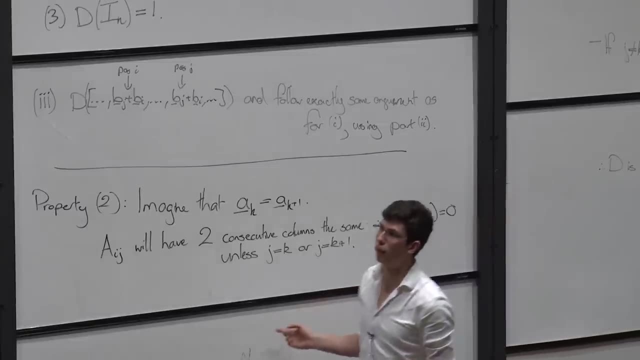 so if I didn't remove either of those two columns, then two of the columns will be the same, and so the determinant will vanish on these n minus one by n minus one matrices, and so this means that when I'm evaluating d at a, I would have loads and loads of terms. 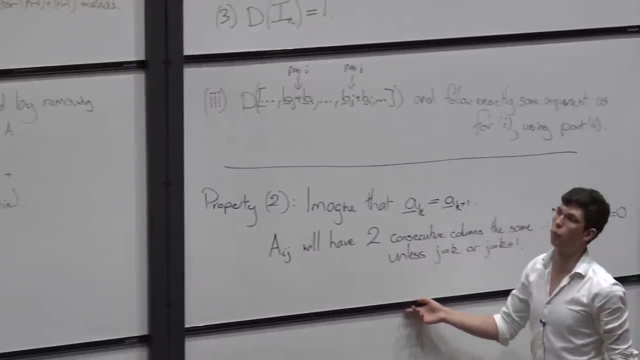 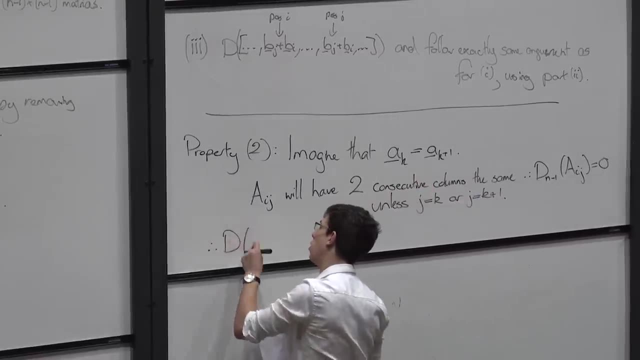 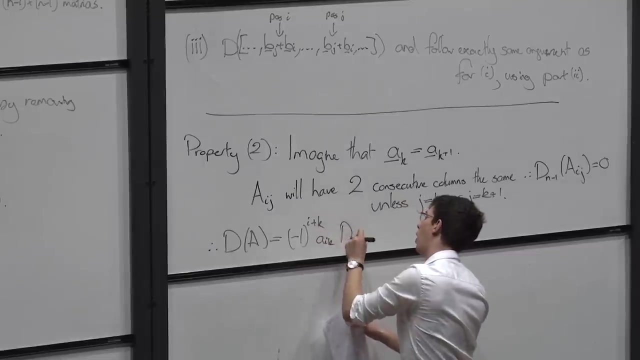 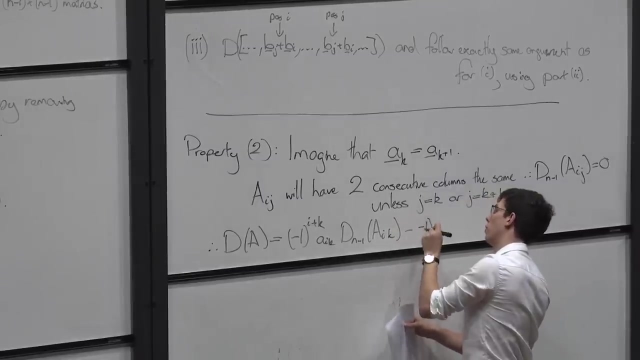 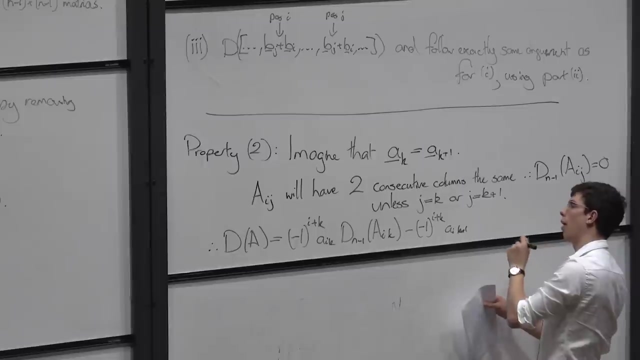 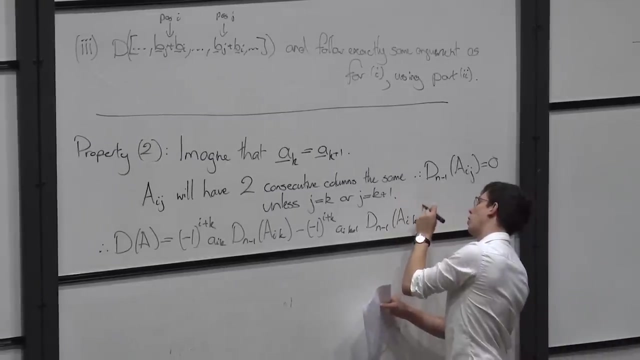 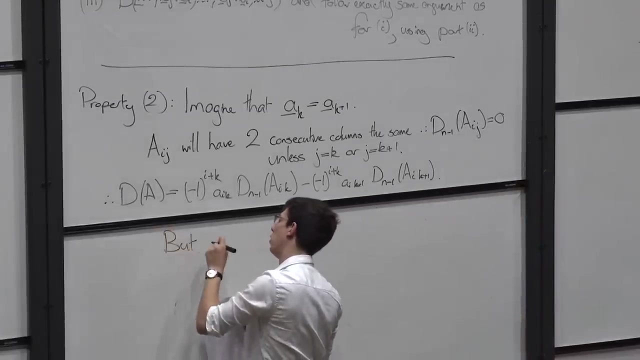 but virtually all of them are zero. I'm only going to get the terms from aik and aik plus one so I can write out precisely what this is. and I just get the two terms from when I have aik and aik plus one. but then if the kth column is equal to the k plus first column, 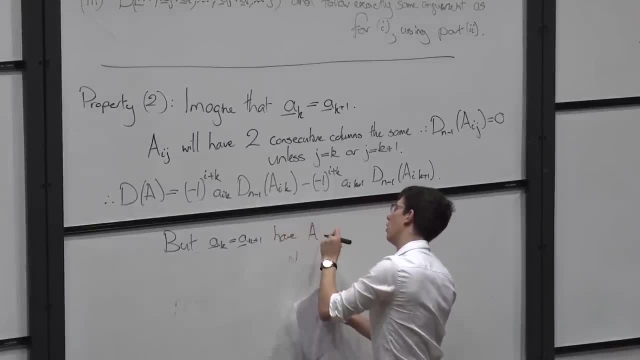 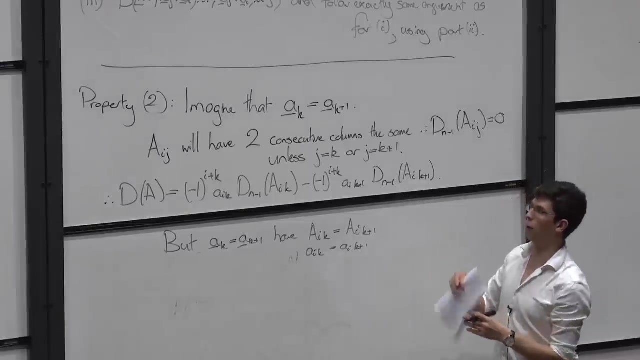 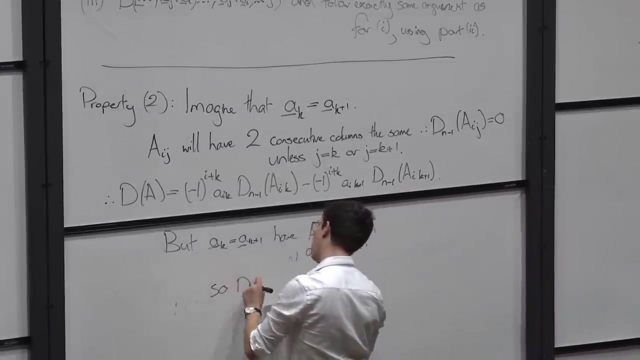 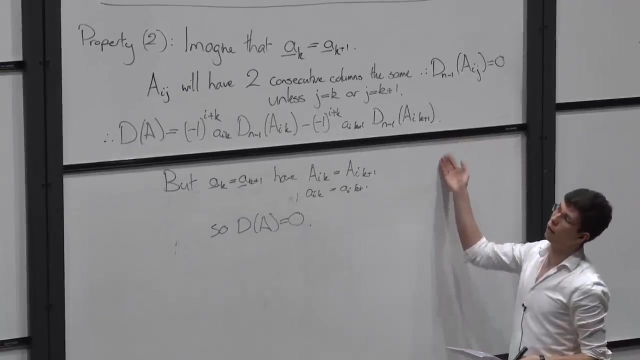 I have that aik is equal to aik plus one, and little aik is equal to little aik plus one, and so, in particular, these two terms are equal to each other, and so the determinant vanishes. so now, finally, I just need to check property. 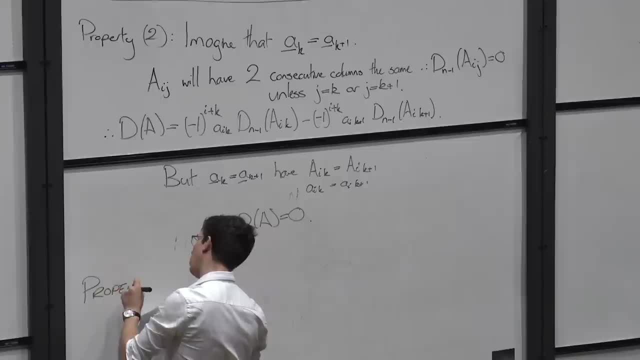 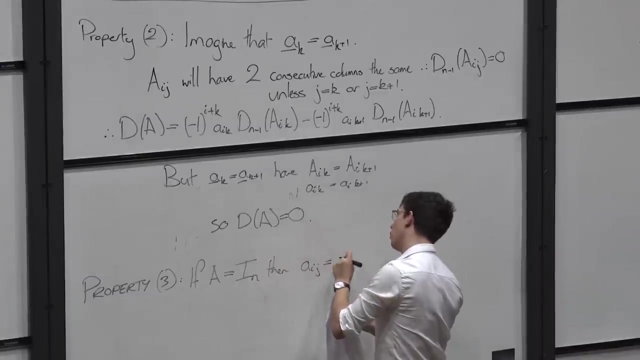 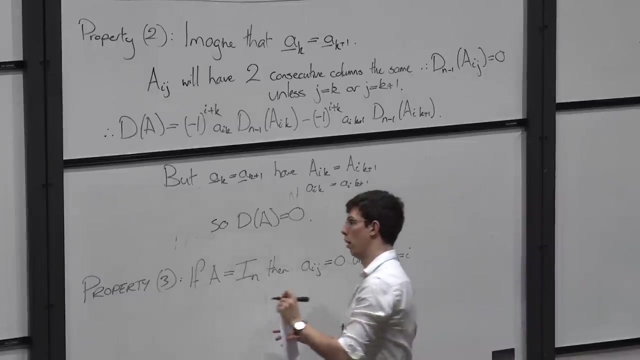 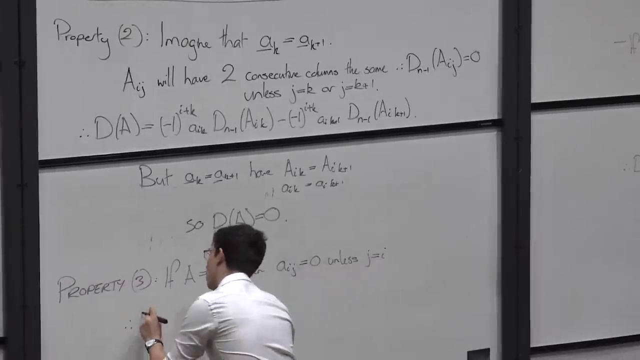 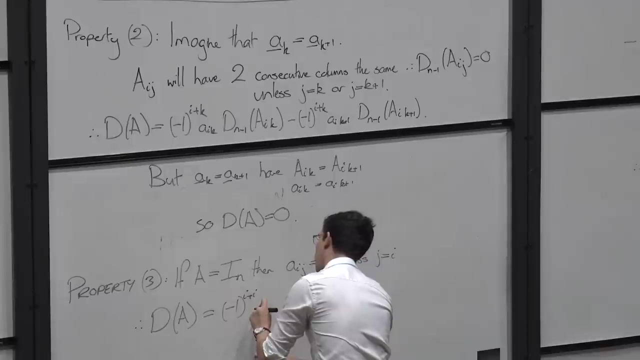 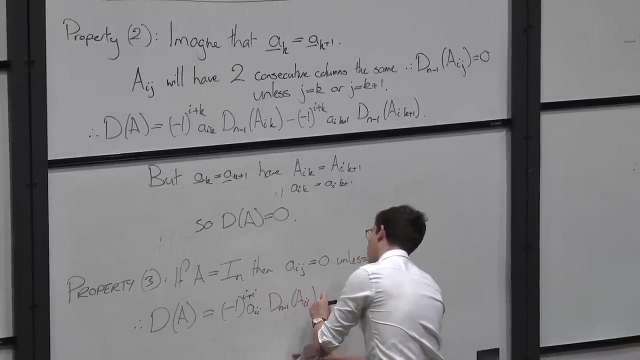 So if a is equal to i n, then a i j is equal to 0, unless j equals i, And so all but one term in this huge expansion vanishes, And so I have this function evaluated at a. It's minus 1 to the i, plus i a, i i d n. minus 1 of a- i i. 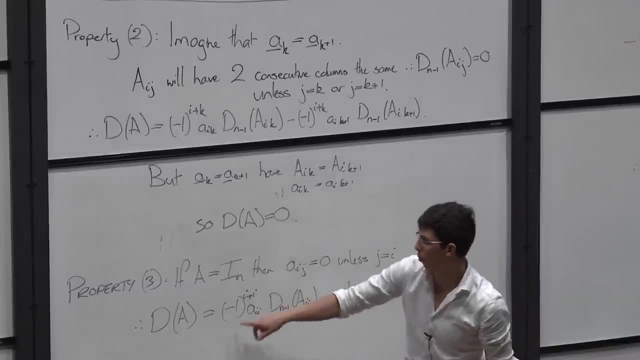 But this is equal to 1, because minus 1 to the i plus i is 1.. a i i is 1 whenever i is the identity matrix And, by assumption of the n minus 1 being determinantal, this also evaluates to 1 at the identity matrix, which. 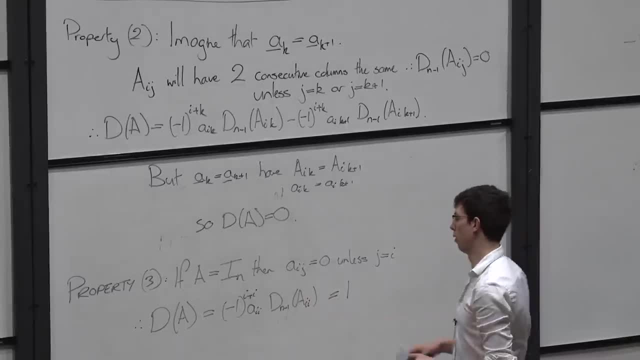 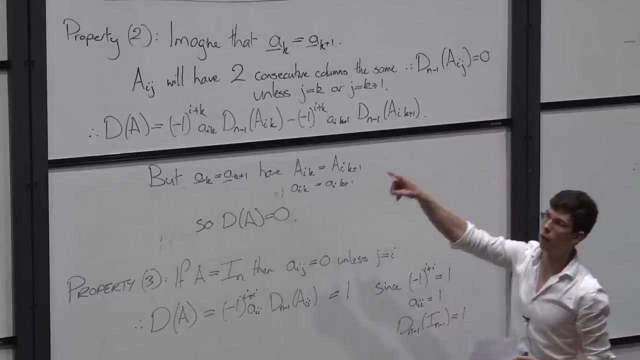 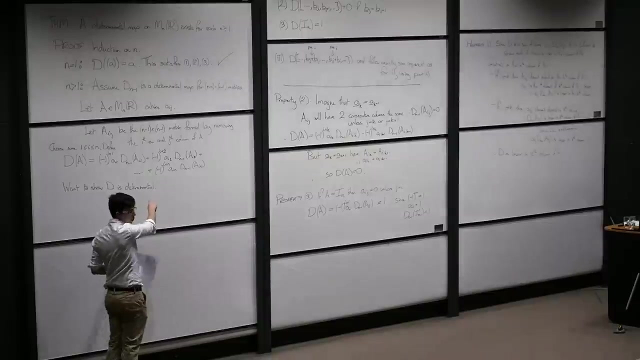 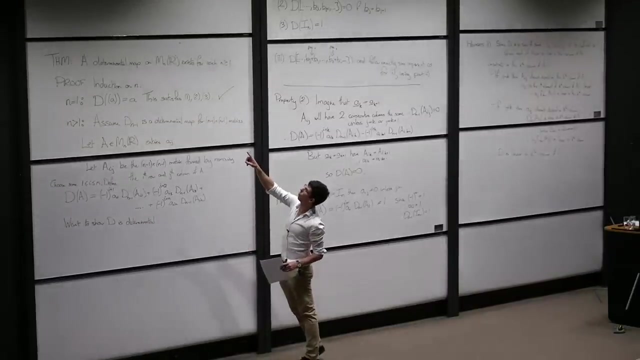 is what I get when I remove the i-th column and the i-th row, And so this means the function d satisfies properties 1,, 2, and 3.. And so I've shown it's determinantal, And so therefore, by induction, we 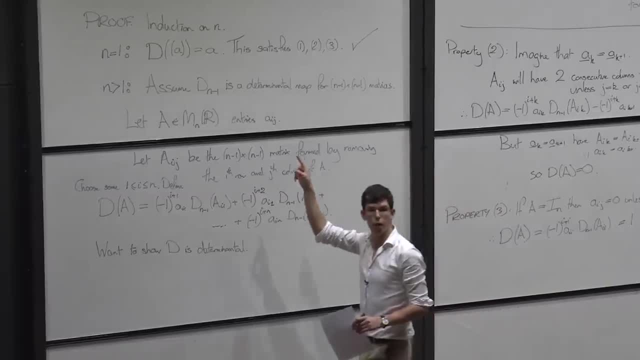 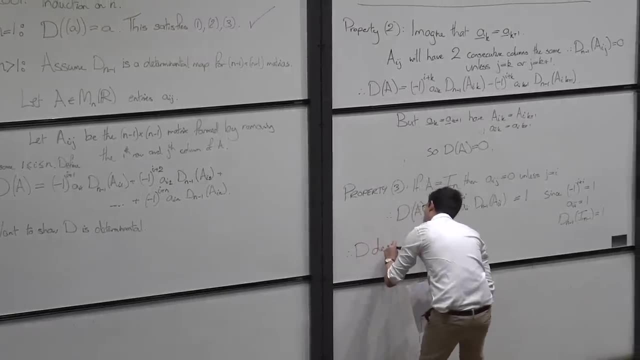 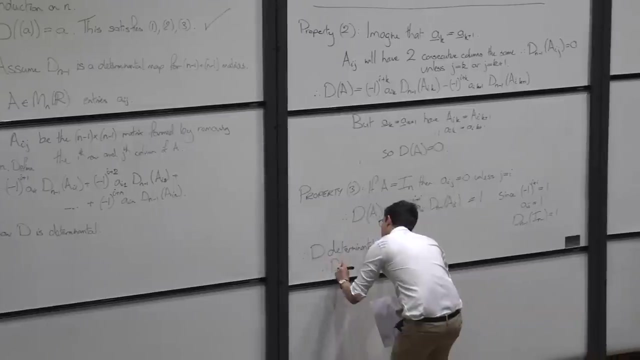 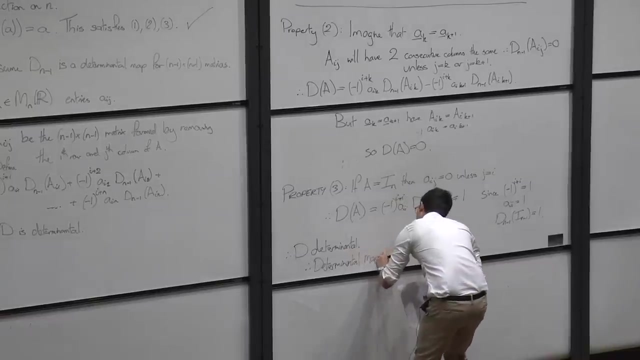 know that there exists at least one different determinantal map on n-by-n matrices. So therefore d is determinantal And therefore d is determinantal, And therefore d is determinantal And therefore d s. is this OK? 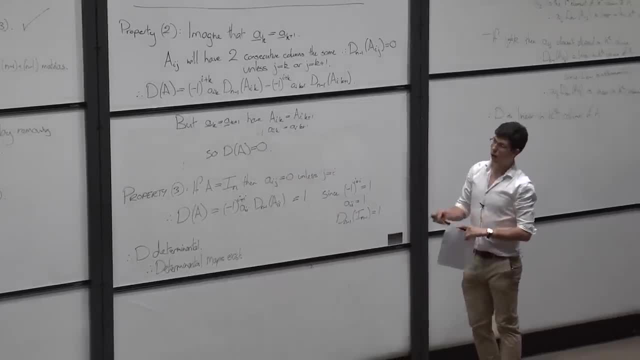 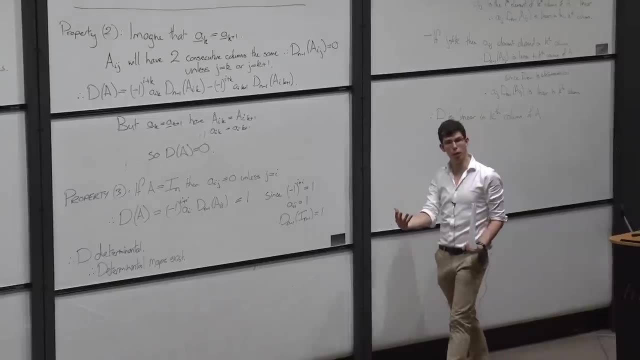 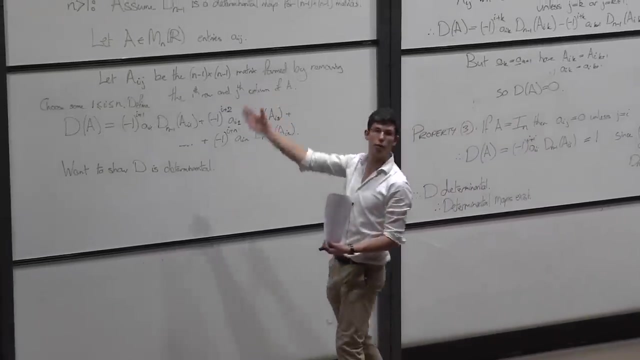 So I'll stop here. What we've seen is that there's this. we guessed that there's this important geometric property of matrices, which is how they scale volumes, But it turns out that it's very difficult to work with that, so we've abstracted this out. 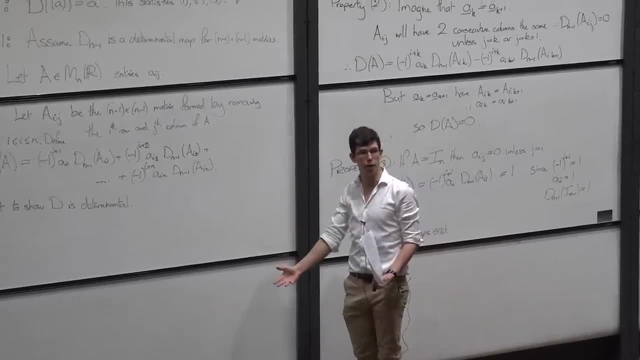 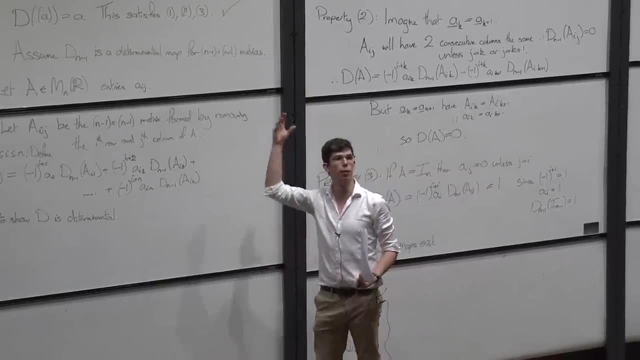 So some algebraic properties, properties and then, working with those algebraic properties, we've shown that there's something that exists that behaves in exactly the same way, and next time we'll show that this is, in fact, a unique map that has all of these properties. okay, thanks a lot. you. 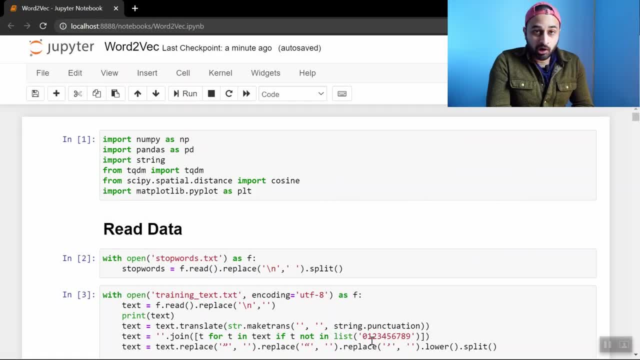 Hey everyone, welcome back. So today we're going to be looking at coding Word2Vec. So the best case scenario is you come here having watched the Word2Vec video that we made, or at least understand the idea of Word2Vec, and then here we'll look at how to code it pretty simply. So I've written all